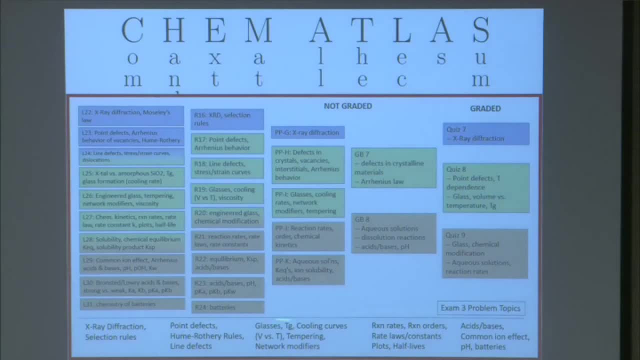 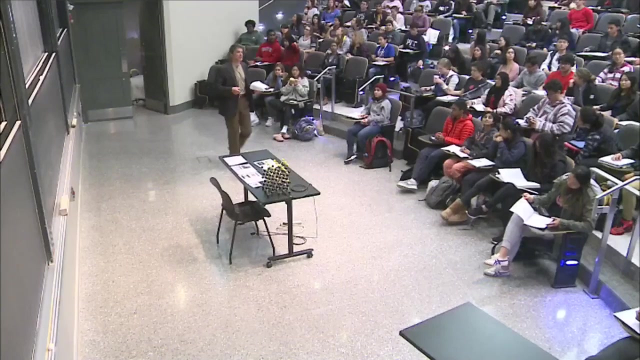 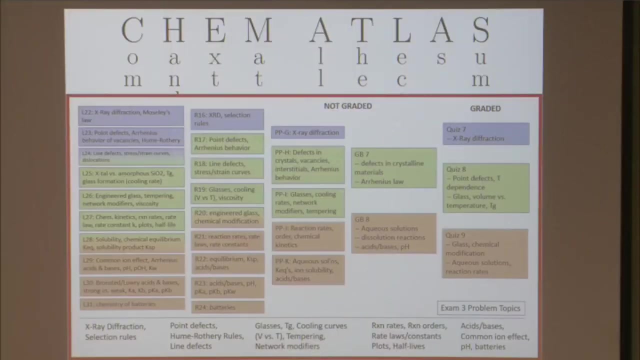 um, uh, holiday in between And there's one topic here we have to start before the exam. It's not here because it won't be on the exam. but we're going to start polymers, but it won't be on the exam. I'm going to spend the whole lecture before exam three just reviewing for exam three. Um, because we're going to have that Thanksgiving break and all that. So that's what. that's what's not listed here. These are just the topics that are covered on exam three. Okay, good, If anyone has any questions, please do let me know. The concept map. 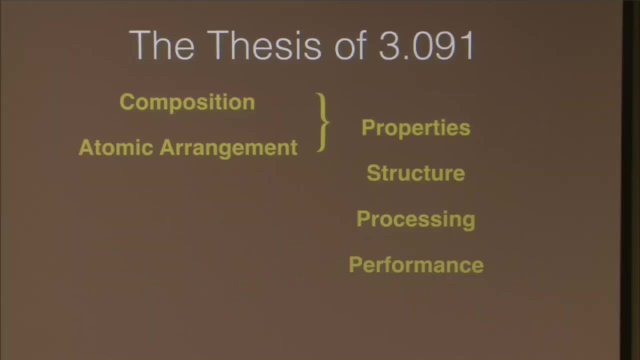 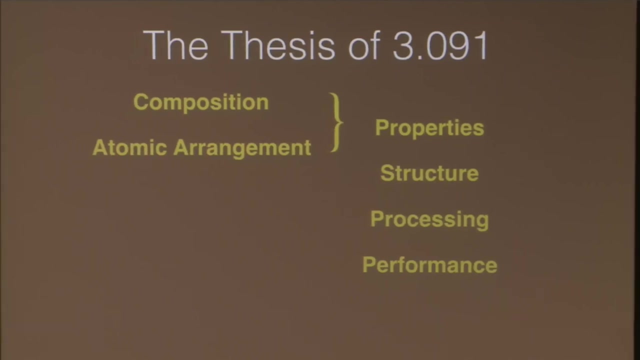 Now the thesis of 3091,. you have seen, in multiple different ways I have tried to convey to you that the electronic structure of atoms is is the key to life, It's the key to chemistry, It's the key to understanding, Um, and and within that you get things like this, which is what we've been talking about recently, like composition and arrangement, right, That's these crystals, That's these, these different right, BCC, FCC, Okay, Um, uh, and then the chemistry you put inside. But you see, the other thing about it is that 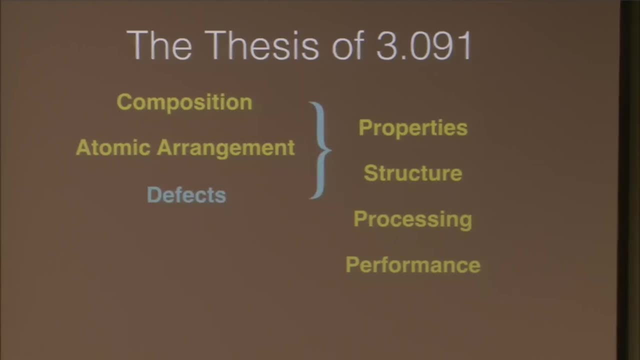 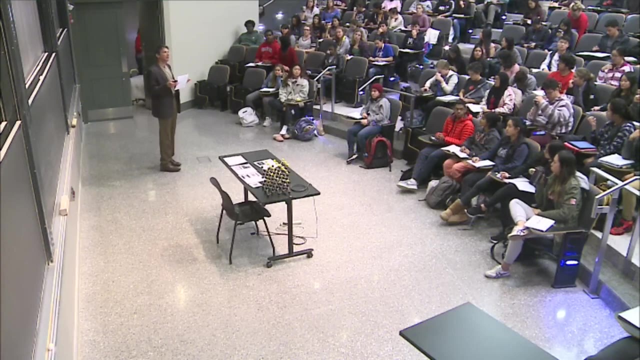 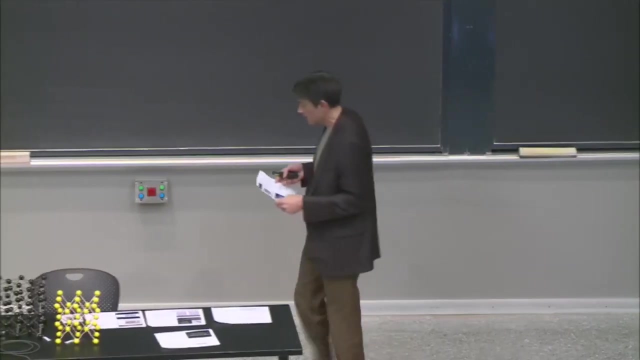 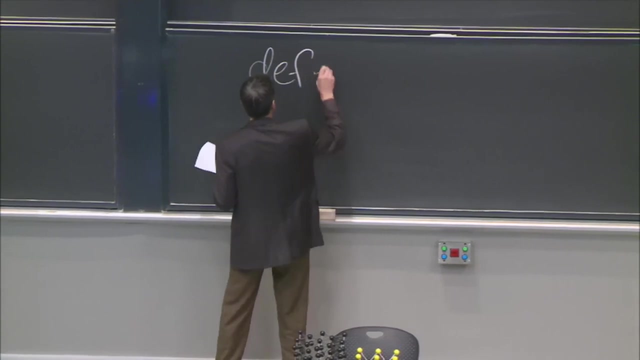 defects. you know, because the thing is that that defects, which is the topic of today and Wednesday, they are absolutely crucial for understanding the properties. If. if they're there- and I just told you they're always there- The question is: how much are they there? All right, Um and and so so if you don't know about defects, if you don't know about defects, then you really cannot fully understand properties. 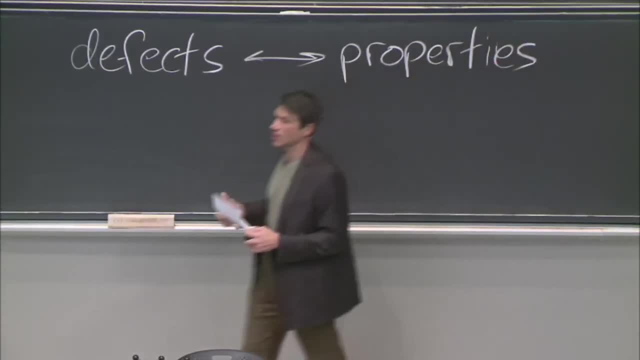 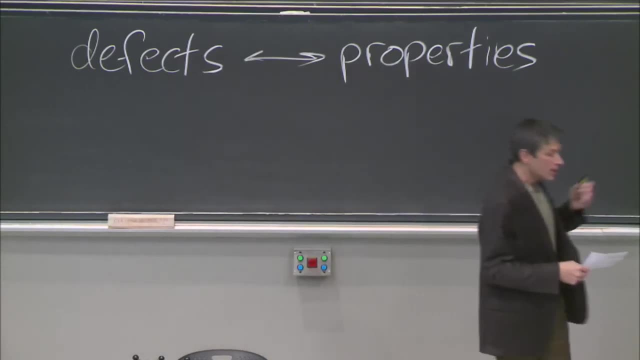 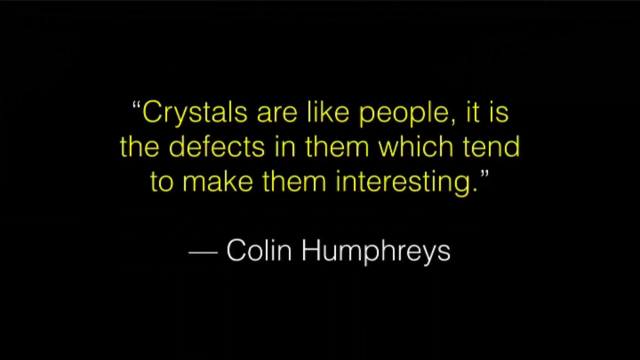 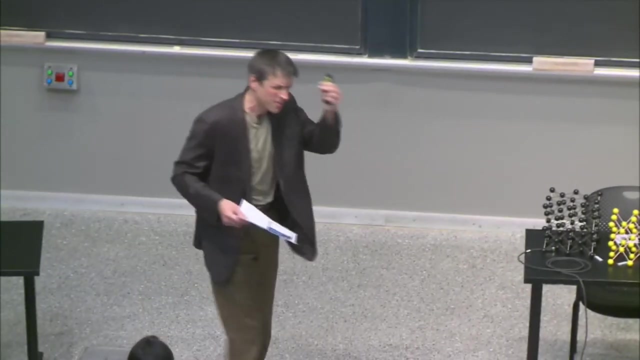 There is a very strong correlation between the two And that's why we have to talk about them. We have to understand them. Now, I love this quote from Colin Humphreys. He said: crystals are like people: It is the defects in them which tend to make them interesting. Yeah, And, and that's actually really true, because defects right Defects sound. you know, I don't want a defect. No, actually, oftentimes you do want defects. 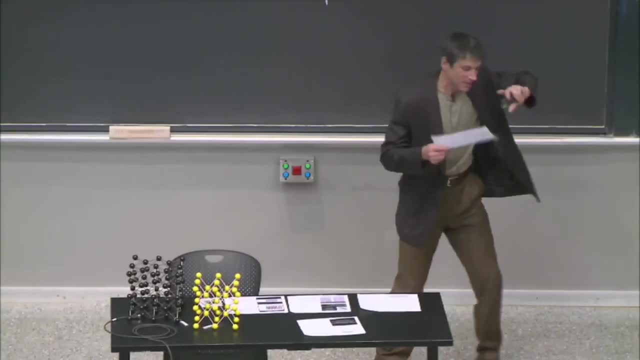 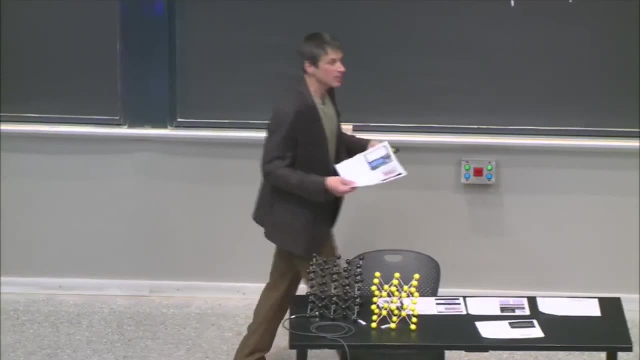 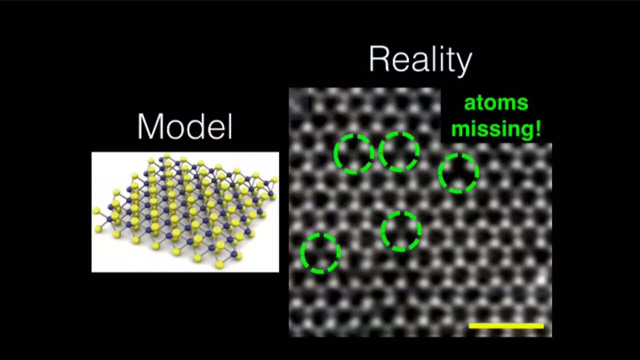 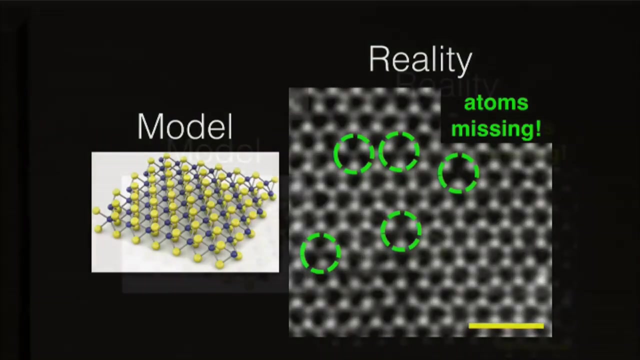 Sometimes you don't, Yeah. So there's some kinds that are kind of like- maybe not things you want in your crystal, And then there are other kinds that actually you are engineering purposefully to be there. Either way, you got to understand them right, And that's what we're doing today, isn't it? So you know, if you take this three layer- we talk about graphene- It's a one atom thick material. Pretty cool. Every atom is on the surface, All right. Here's another example of what's called a 2D material. Why It's not 2D, but it's called a 2D material? because it gets you. 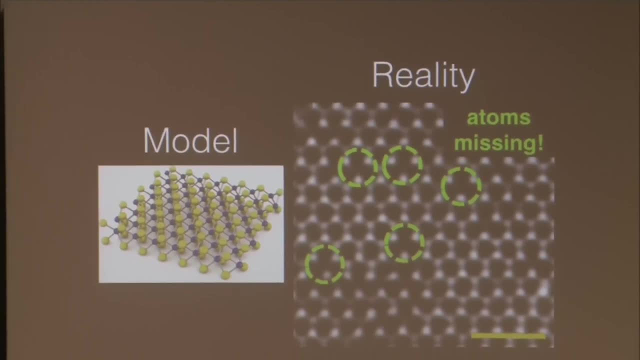 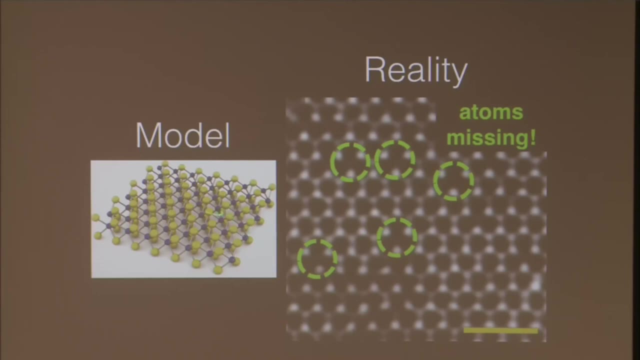 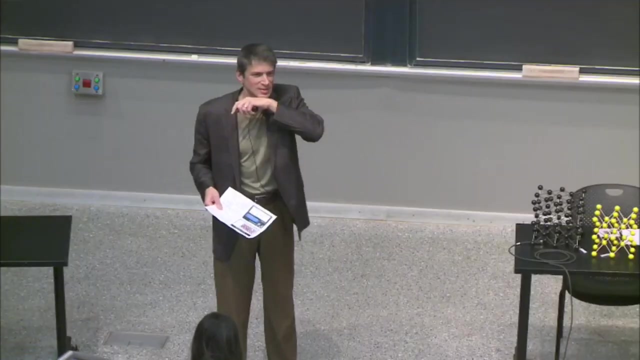 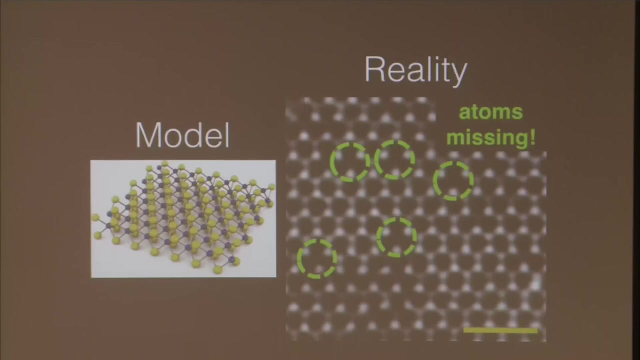 like you know more publicity on your work. This is molybdenum, but this is molybdenum disulfide. It's really cool material. It's three atoms thick, So it's kind of like 2D-ish. right Yeah, but see, that's the model. That's the model. This is reality. This is reality. How do you see? how do we see atoms like this? That's a real picture. Do we use x-rays? No, What do we use to see atoms that? well, Electrons. Electrons are our light, right. 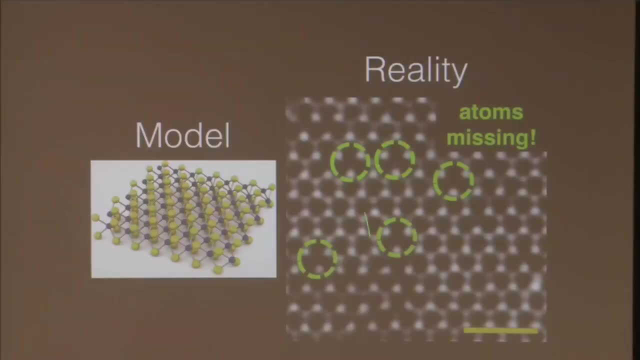 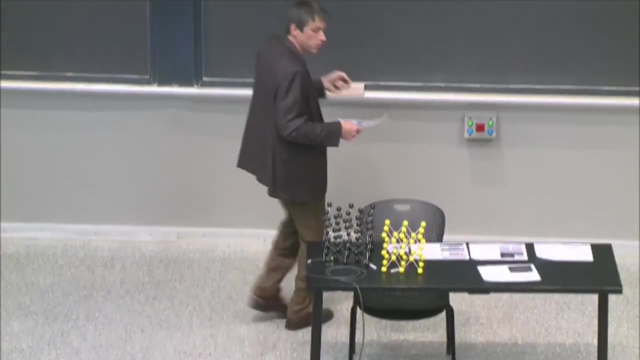 That's what we're using. This is an electron picture Electron And if you do that, you can see individual atoms. And look at that. There's places where atoms are missing all over the place. That's reality. That's reality. And those where you have one atom missing or where you have one thing that is localized and disruptive to the regularity of the lattice, that's called a point defect. So let's write that down. That's the one. 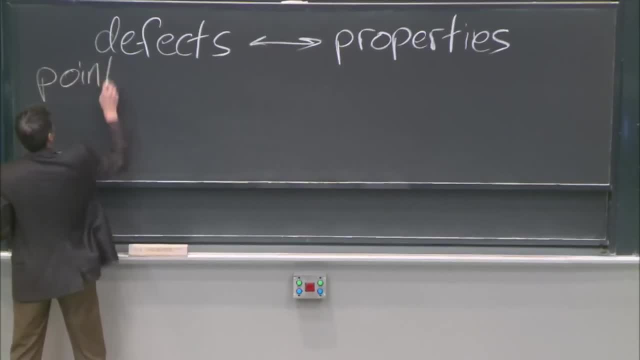 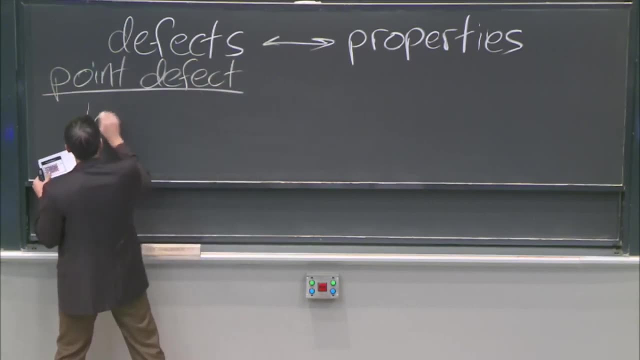 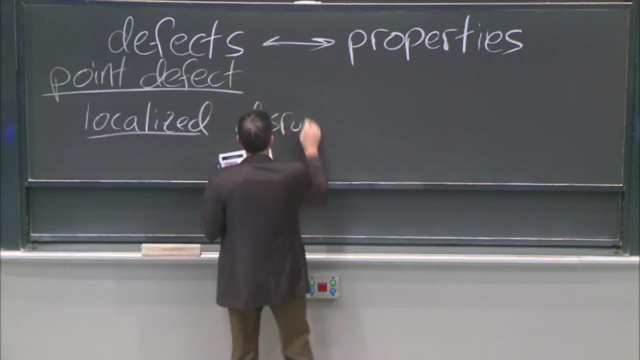 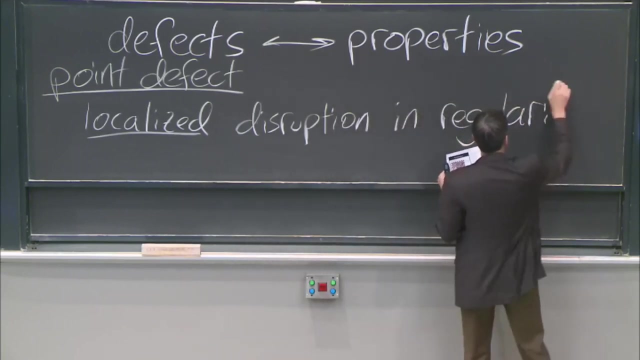 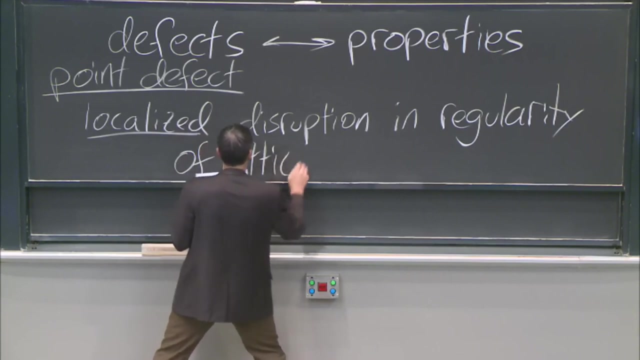 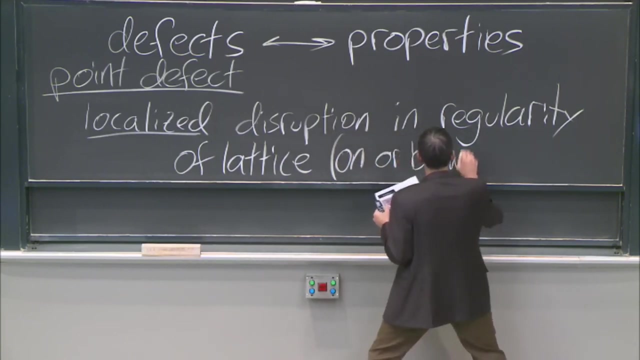 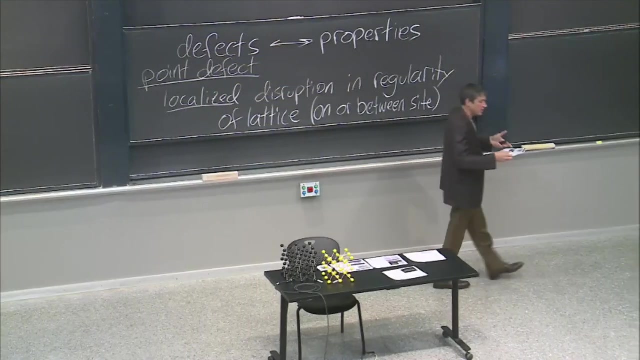 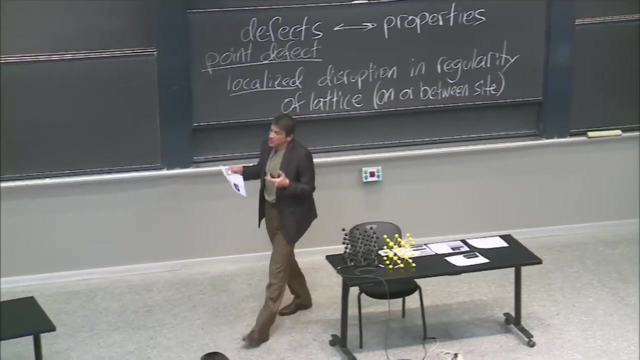 that we're talking about today. So the point defect, point defect is where you have a localized, localized disruption in the regularity, regularity, the periodicity, the repeating of the lattice, And it could be on or between- We'll see this- On or between sites, right, It could be a defect that is like you see, here There's an actual atom missing. It could be something that maybe got in there in between sites, But either way, it's a disruption that's localized to a point or almost a point, And so it is Gesundheit that you can see that if we do that, we're going to get a point defect, And that's what we're talking about. 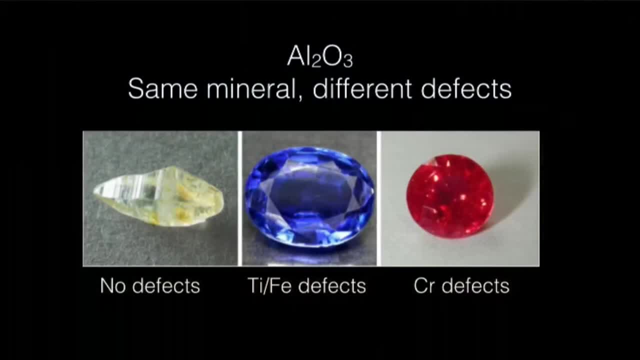 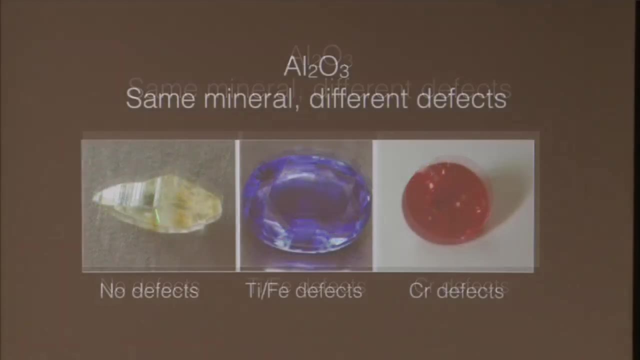 We just make these disruptions in something Illumina. we talk about Illumina, right. Illumina is really strong lattice energies, So it's like it's like sandpaper. Oh, it's also toothpaste, It's in a lot of stuff. Illumina is a great, but look at this. That's Illumina with almost no defects. It's got still got some. You can never get rid of them all, But here it is when I purposely engineer the defects in Illumina and I put a little titanium or iron, Or here's it when I put chromium. So there's one. 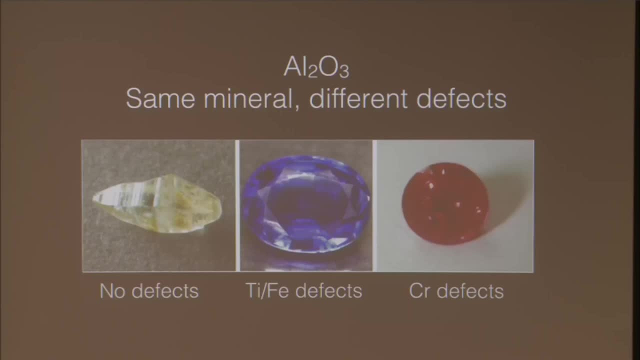 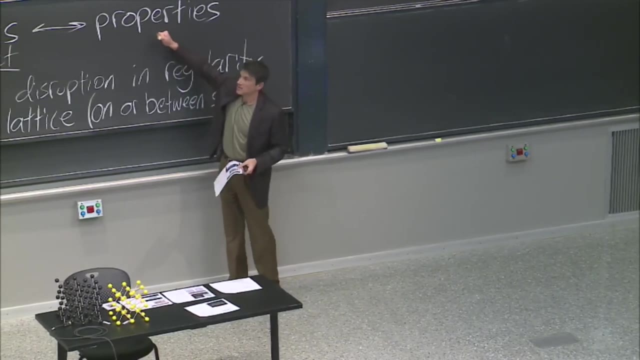 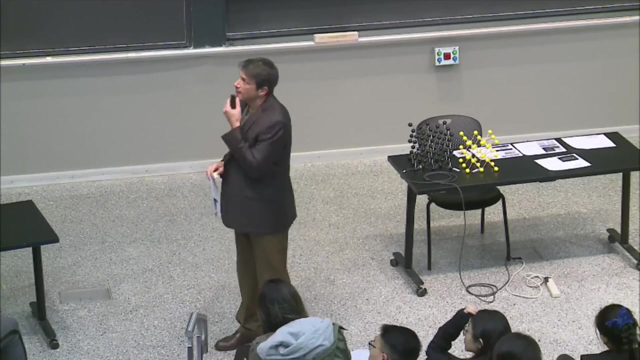 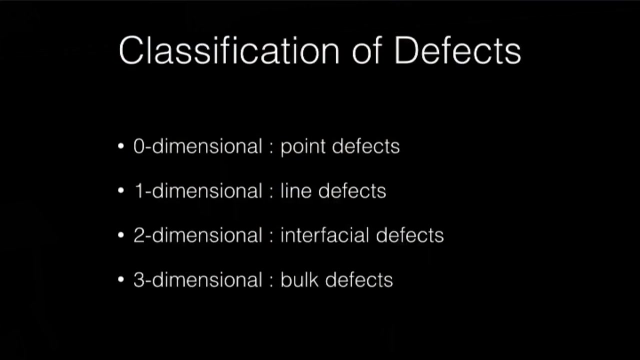 property where the localized disruption- and it's not a lot, as we'll see- the localized disruption changes the properties. That is key. That's just color right. This applies to most properties of materials, And so you know. so this, this first one, the point defects that we're talking about today, you can kind of think of those as zero dimensional because they're, they're localized. You know they don't really go off in a line, They don't go off in a plane. 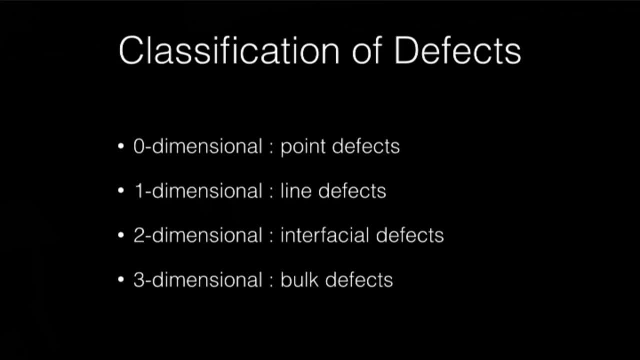 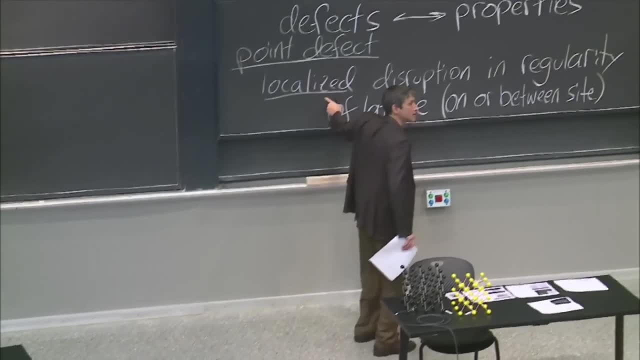 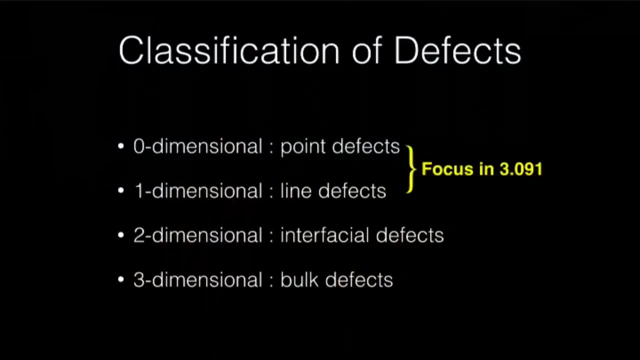 Or a volume, And you can have defects that are. that cover all of those possibilities. But these are points, right? This is this is what the word localized means here, Okay, Okay, Now, in this class we're not going to cover all of them, but we will cover these two Today, this one, On Wednesday that one, And that'll give you enough of a sense of the role of defects and how to think about defects in crystals, right? So this is how we think and classify. 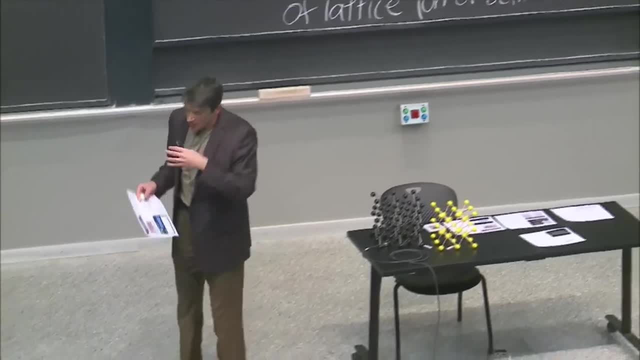 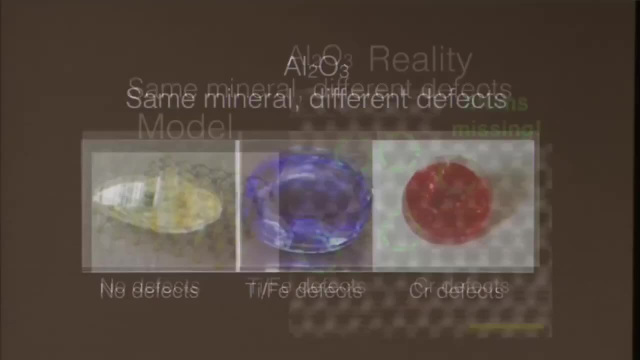 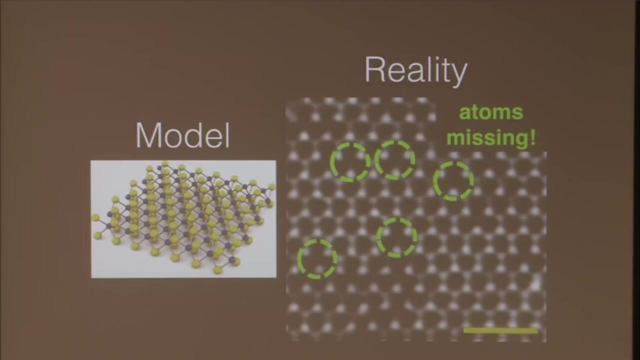 Defects. Okay, Now the four. so now we're going to point defects. Now the four. there are different types of point defects that can happen. The one that you saw here is is a certain one That's called a vacancy. It's because there's an atom that's vacant. So you literally just lost an atom somewhere in there. Okay, Now, that that's a vacancy And that's that can. that always exists. But you could also have taken something like one of the atoms that's already in there, maybe an aluminum or an oxygen atom. 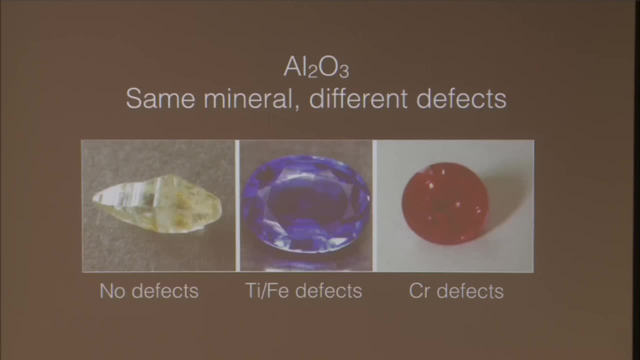 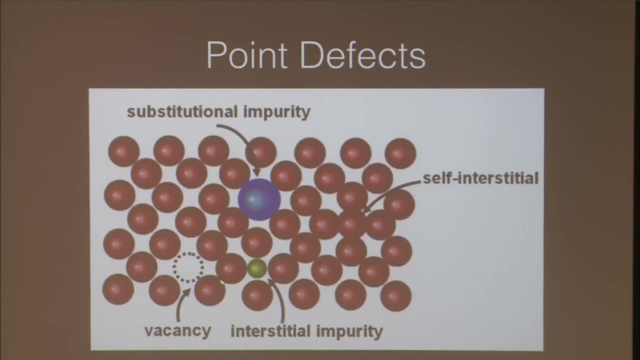 That's in the lattice And you could substitute something in place of that. That's another. Why is that a point defect? Because I didn't like. I didn't like tear something out. No, but you changed the regularity, localized disruption and regularity, So I put something else in for aluminum. That's a point defect, Right, And again now go back to here. You can see it here, So we classify these right. There's a vacancy, which is an atom missing, There's. there's what's called an interstitial, which is an atom that goes in between the atoms. 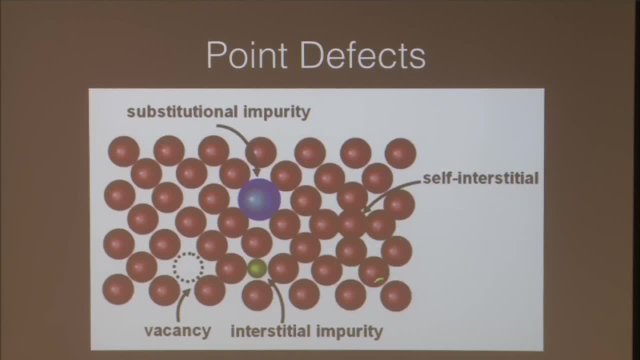 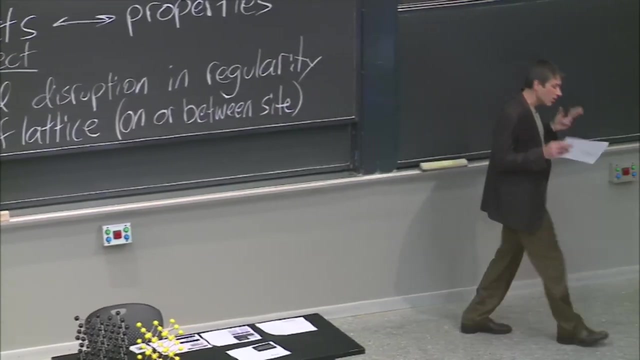 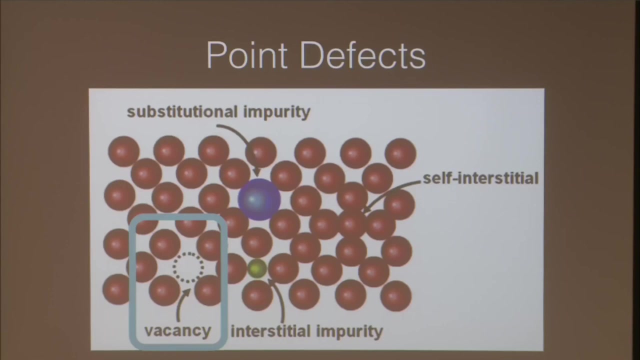 Here it's a self interstitial, So it's the same type of atom And these are: this is where you have a different type of atom in between, And this is where you have a different type of atom as well. Those are both called impurities, And I will talk about those all. today, We're going to start and focus a lot of our attention on the vacancy, And that's what I want you to use this goodie bag to understand- is the vacancies. Okay, Vacancies. Why do vacancies happen? What are vacancies? To understand vacancies: 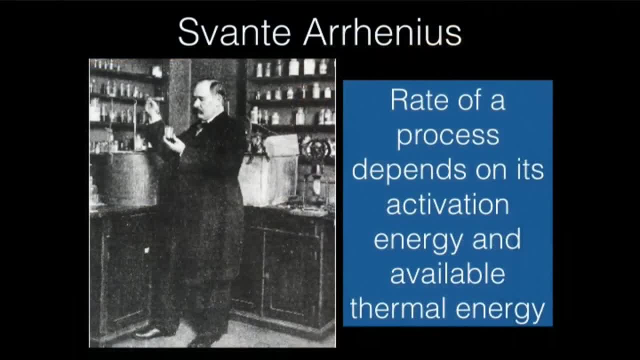 In crystals. We have to talk about this guy, And this guy was brilliant. This I'm sure you know. his name is Svante. Yeah, it's written right there: Svante Arrhenius Arrhenius studied in the late 1800s so many different things and made so many contributions that it's almost hard to catalog. He was brilliant And, and you know, he won the Nobel prize in chemistry for his work on electrolytes. 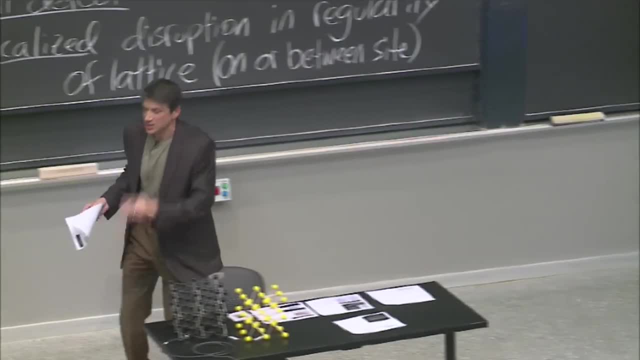 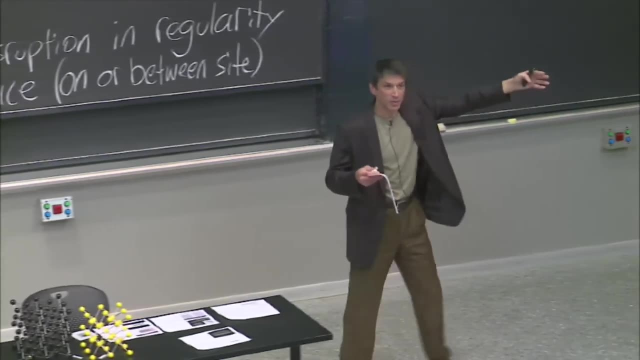 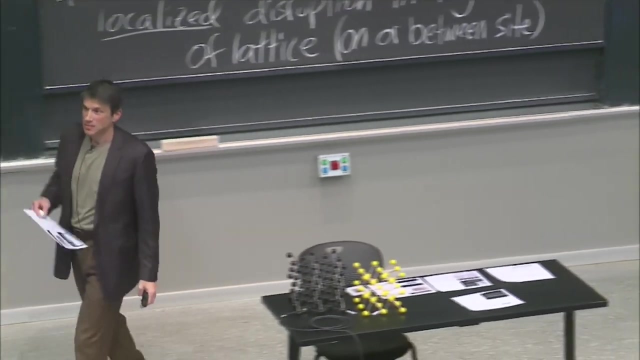 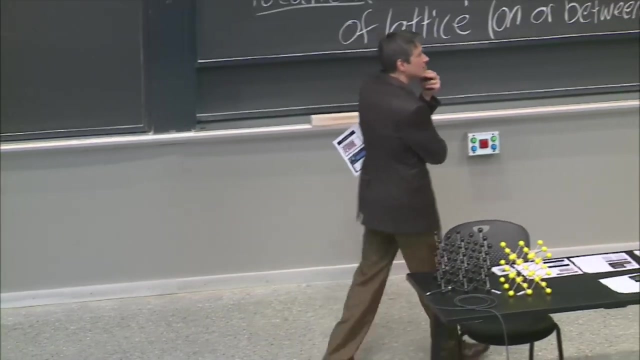 But he also worked on immunology. He was the very first person in the late 1800s to come up with a model for global warming and the role of CO2 in the temperature change of the planet, And his predictions were actually pretty darn good. He was brilliant, And one of the things that he did is he observed what were called activated processes and how they depended on temperature. 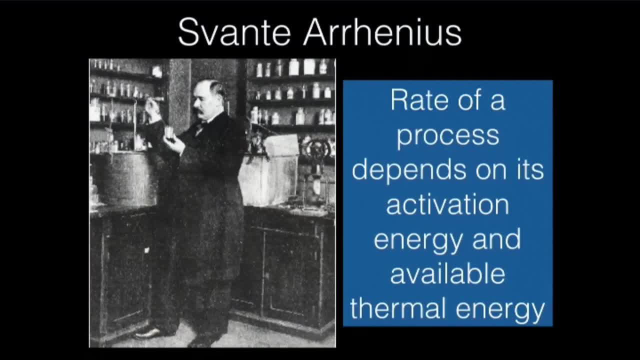 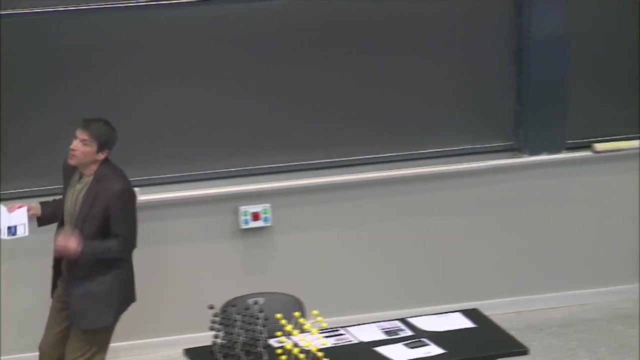 And so we have this equation that I need to talk about today and it's going to come back. So we're going to talk about this equation, which is the Arrhenius equation, that relates the rate of some process to the temperature and the activation energy for that process. So we got to talk about what all that means. All right, Now we will. we will be using this Today. we're going to use it to think about concentrations of vacancies in a crystal, which, for example, is a crystal. 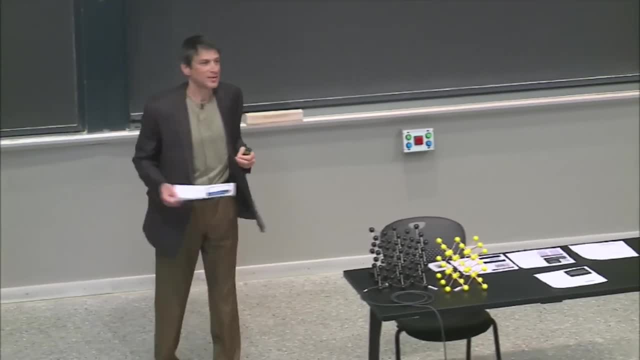 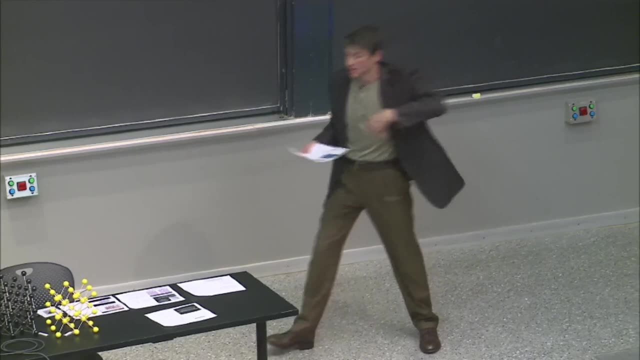 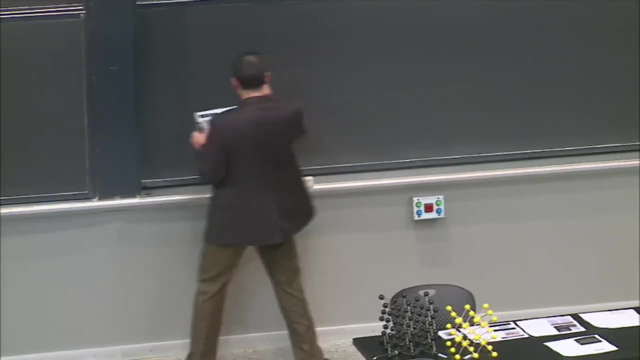 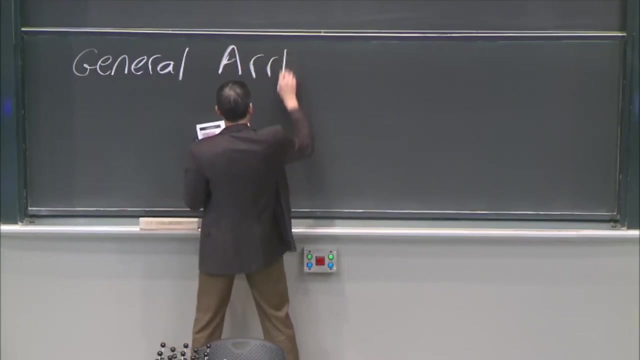 So we're going to follow Arrhenius-like behavior, right And. but then we're going to come back to it when we go into reaction kinetics in a couple of weeks where we talk about reaction rates. So we'll be using Arrhenius multiple times throughout the rest of the semester. So what is it? So the Arrhenius, so the general Arrhenius equation can be written like this: Arrhenius, he was not in the army, but this is just the general equation. 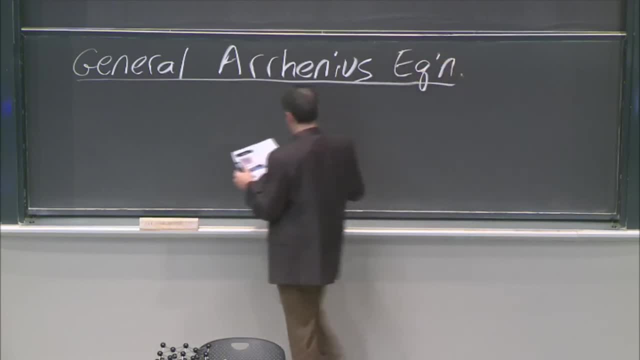 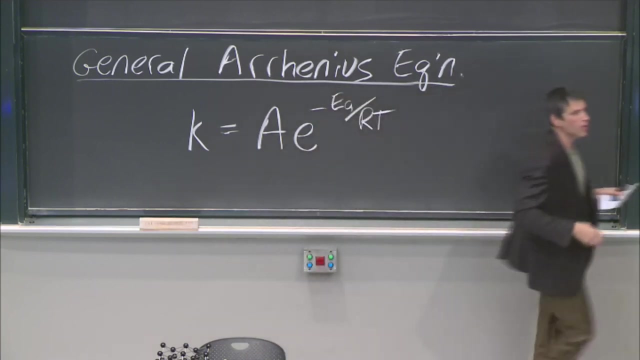 Okay, So let's put equation there, And, and so we have K, which is some rate, So equals A. I'll talk about each of these times. E, the exponential of E to the minus EA over RT, What are these things? So this is the general equation for the rate of some process. As we're going to see, this applies to many, many processes, including vacancies. Okay. 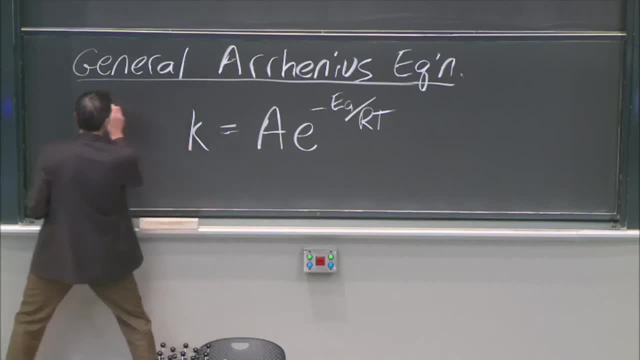 But this is sort of the rate, So you can think of this as: okay, let's just that's the rate of a process, rate of some process. Okay, I mean you could think about it as the number of times something happens per second. That's a rate, right. It doesn't have to be those units, but that's like a rate, right. How often does this happen? The rate of the process. 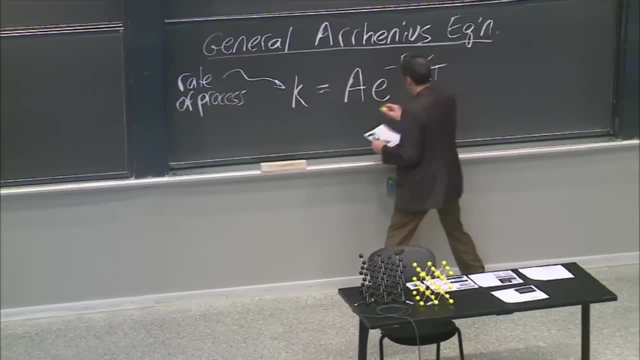 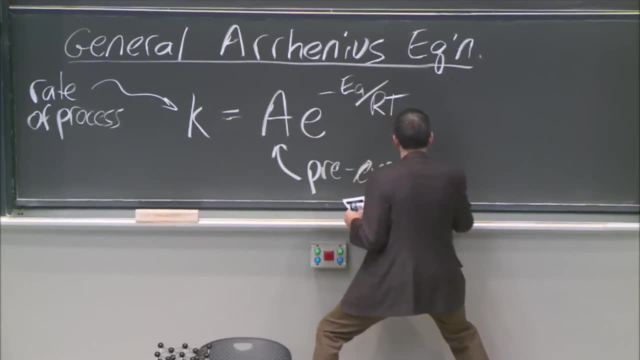 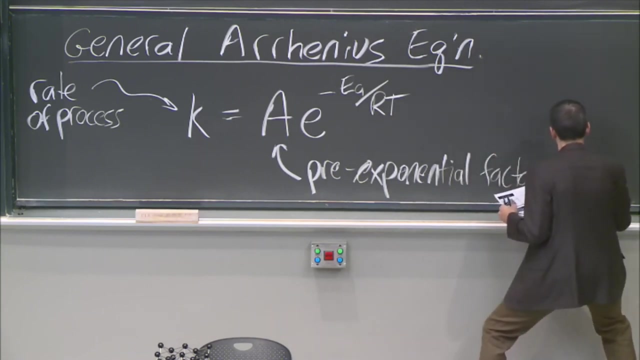 But now, so that's dependent on some thing called the pre-exponential that I will talk about. Pre-exponential exponential, that is a factor, that is a constant, And here we have this exponent, and this is such a beautiful expression. 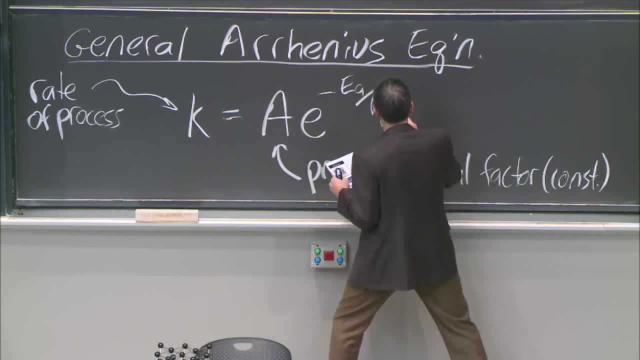 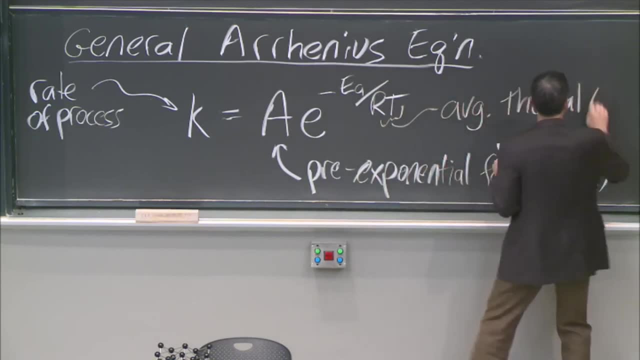 So this is the average thermal energy, average kinetic energy, average thermal energy. right, It's taking temperature and it's making an energy. It's taking energy out of it. Now remember- we've already talked about this before- that you know you don't get. what you get are distributions. 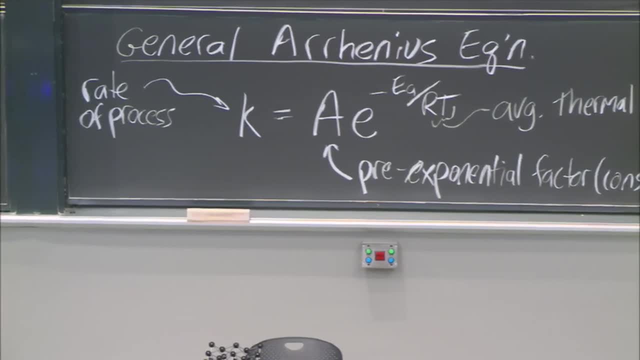 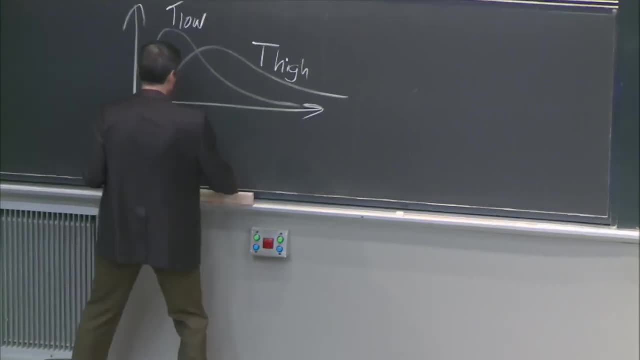 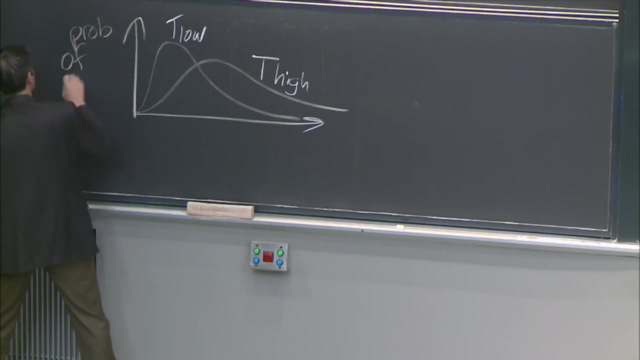 So you know this would be T high. Remember, I've drawn this exact thing and this might be T low and this might be. you know this, this might be the, you know the probability of something happening, probability of occurring. 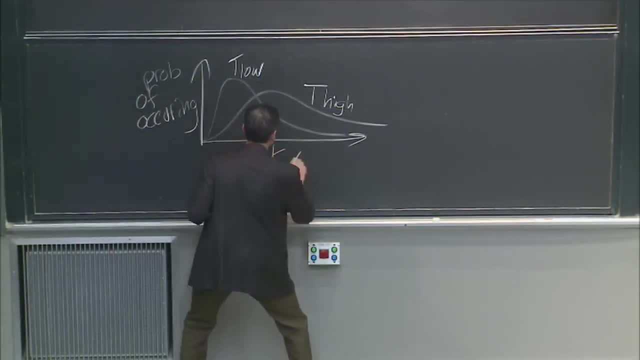 And then, in this case, we talk about this as the kinetic energy, And then, in this case, we talk about this as the kinetic energy of the molecules. That's a graph we showed already, But so, but this RT is an average. 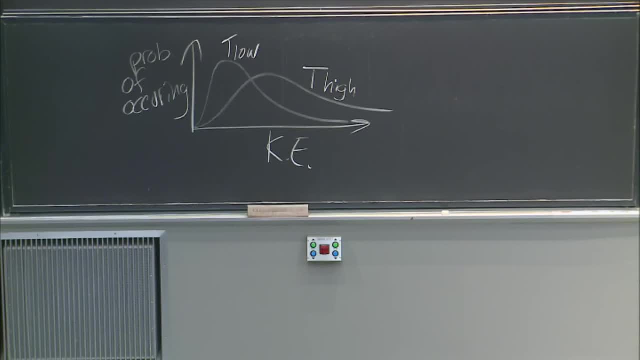 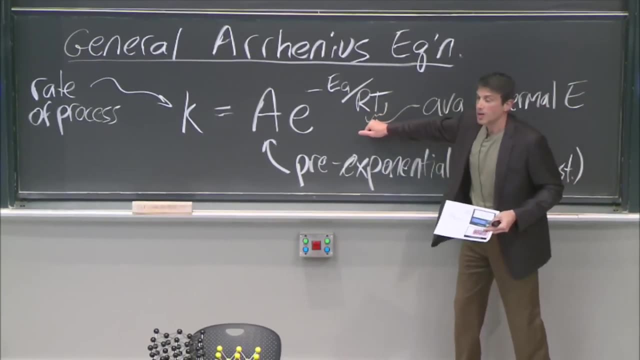 So I just want to make sure you don't forget: this is a number, This is a number You've got at 300 degrees, at 1000 degrees. you calculate a number here, But whenever you're talking about temperature, you're talking about distributions. 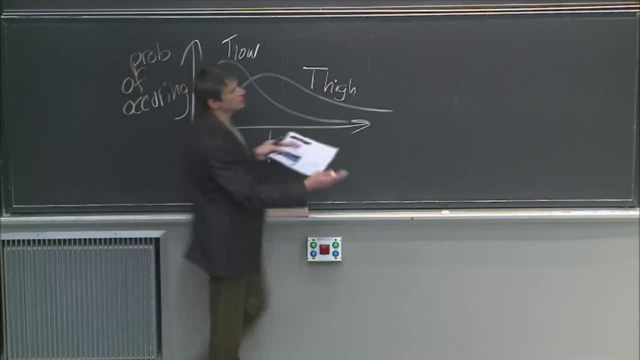 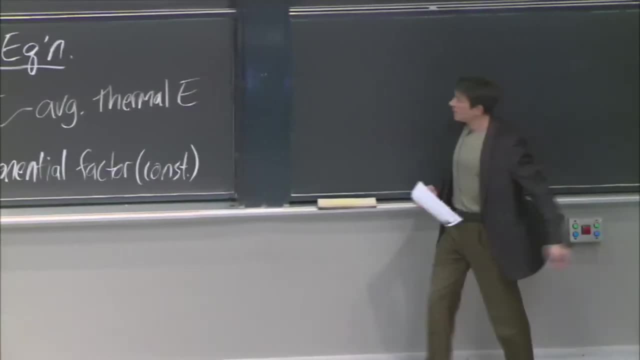 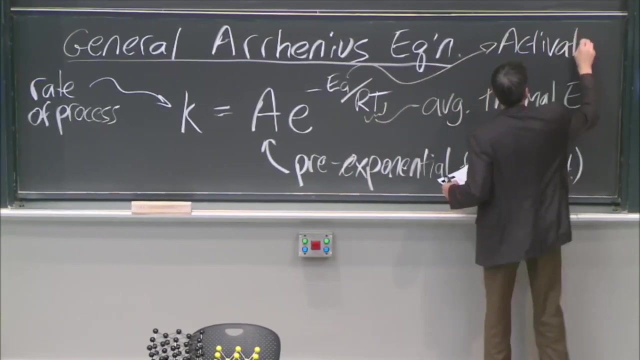 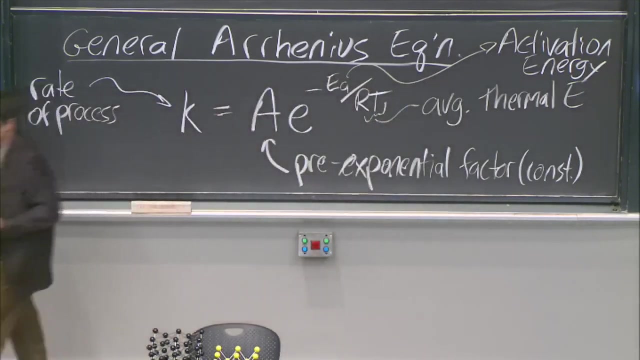 There's some average of the distribution, but you're always talking about distributions. That's important for understanding Arrhenius. That's important for understanding Arrhenius. Okay, Now, this thing here is called the activation energy. Activation energy, And that is the energy that you have to get over for something to happen, for the thing to happen. 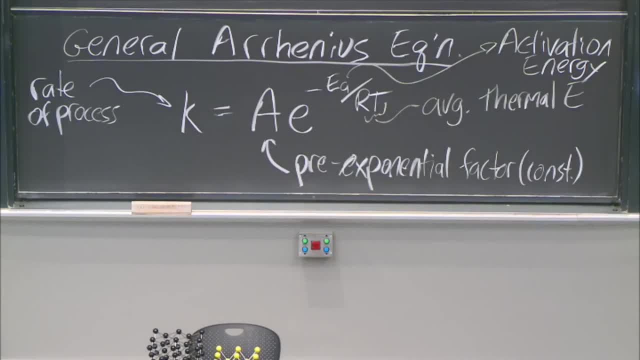 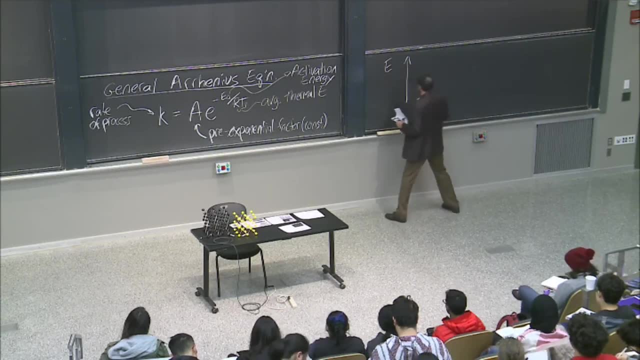 Let's take- I love this analogy of the bookcase. I'm going to draw that now. So let's suppose that you have energy like that. Okay, So maybe this is like potential energy. Yeah, let's go ahead and say potential energy. 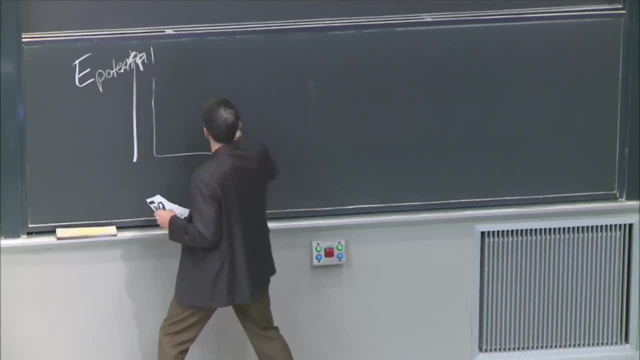 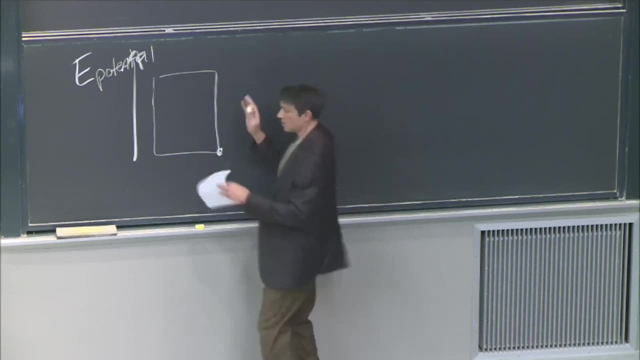 Then if I've got a bookcase and it's very, very heavy And I want to push it over on this hinge, So I want to rotate it and push it over, Then you could imagine that at some point it's going to look like this: 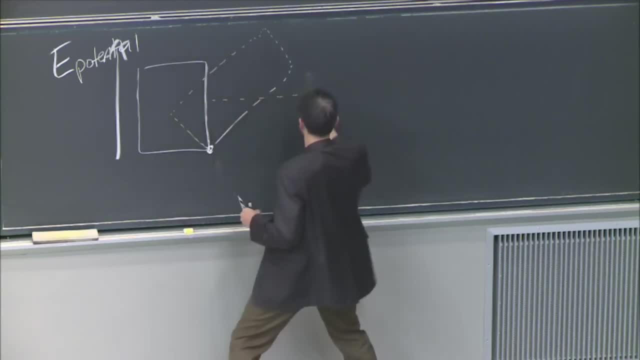 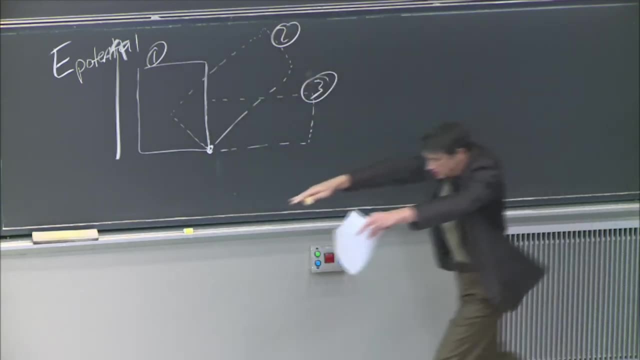 And then at another point it's going to look like this, Right? So if this is like step one and that's step two and that's step three And I'm pushing this thing over, Well, this is the activated state. 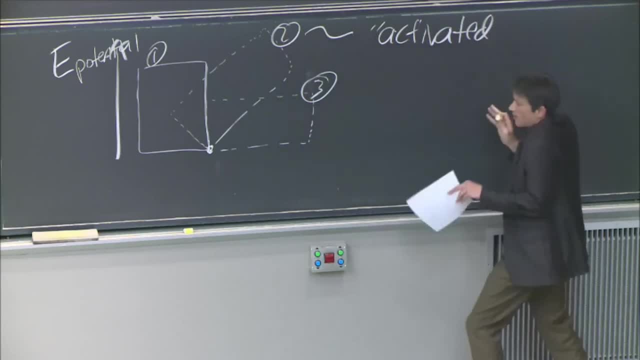 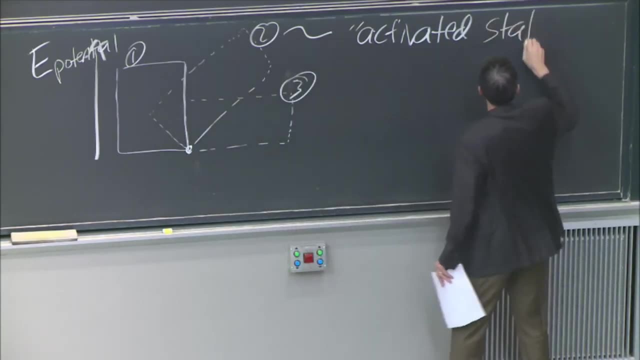 Why? Because it's where I've gotten to the highest energy And that's where this energy graph is important. This energy axis, This is the activated state of the bookcase Right. So if I plot the energies Right, You can say one, two, three. 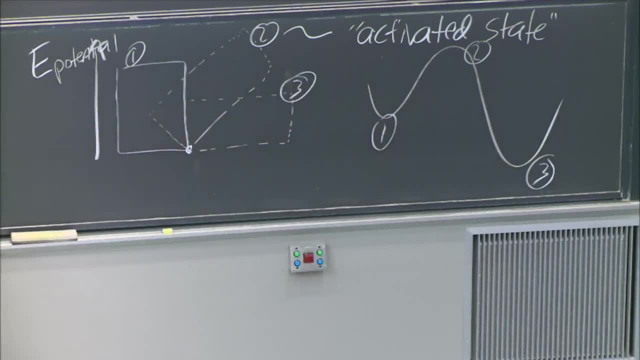 You can think about it like that, Right, I've literally So, because it's a potential energy, Right. So it's like: here's the gravitational, Here. it went up a little bit, Right. So you can think about it just like that. 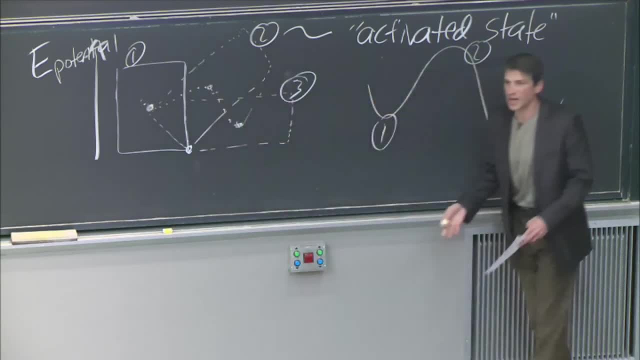 And here it came back down. That's why I like this analogy, Because it really gives you intuitive feeling for what's happening here. There's a process. The process is pushing the bookcase over. That bookcase has some energy associated with it. 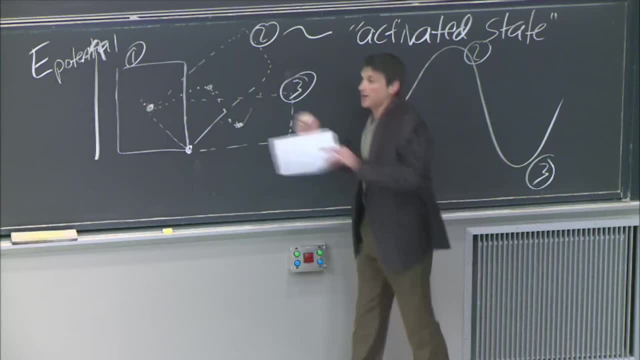 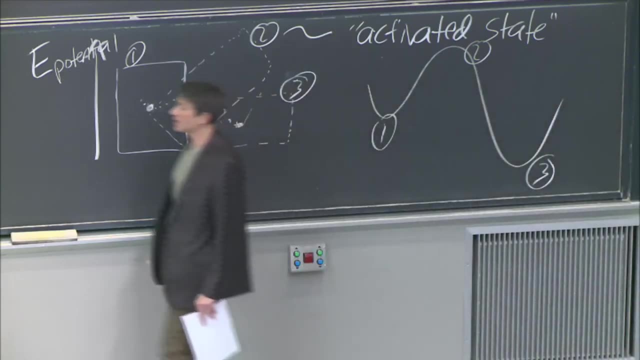 Here and here Potential energy And it's got some energy I got to put into it to activate it to go from here to here. Right, That's why that's called the activation energy. That's what this EA means for the general Arrhenius equation. 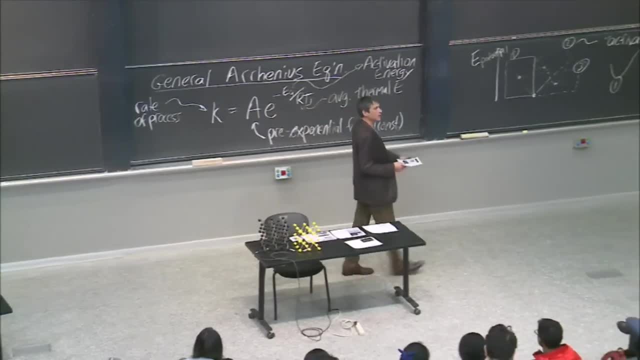 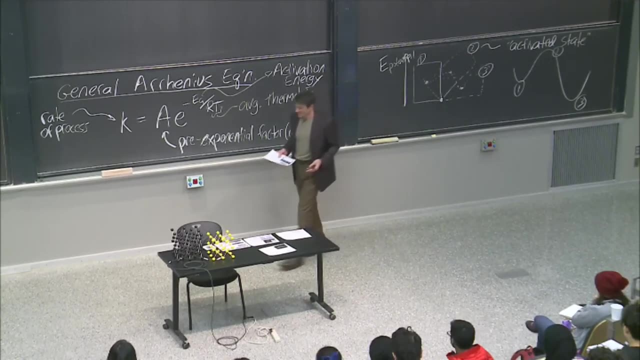 You're pushing the bookcase over. Yeah, but how are you going to push it over? Well, clearly you're going to run around the room and accidentally knock into it, Because that's temperature. Maybe that's not a good, But if you had a lot of people running around a bookcase, 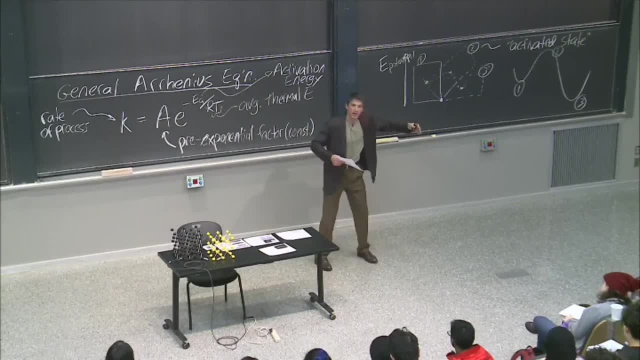 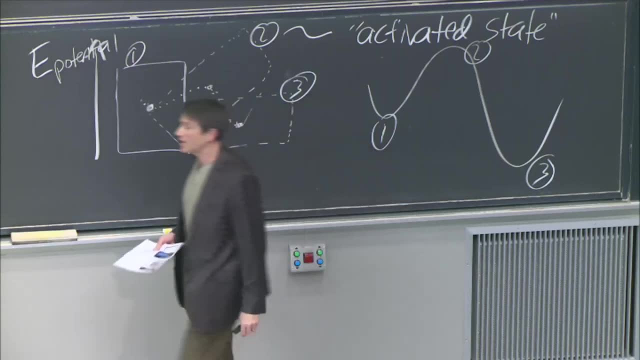 Maybe once in a while They'd kind of bang into it- Thermal energy, Right- And then maybe another time you increase how fast everyone's running And you give them more energy. So now not only are they hitting it more frequently, 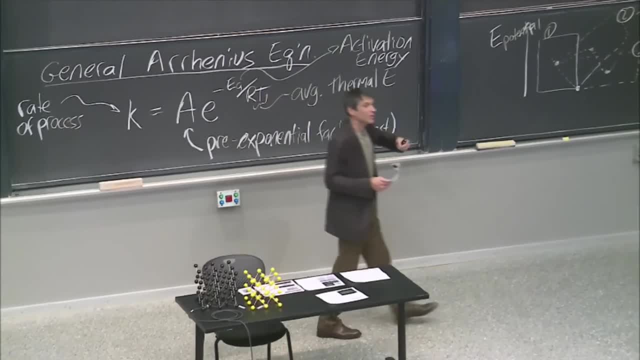 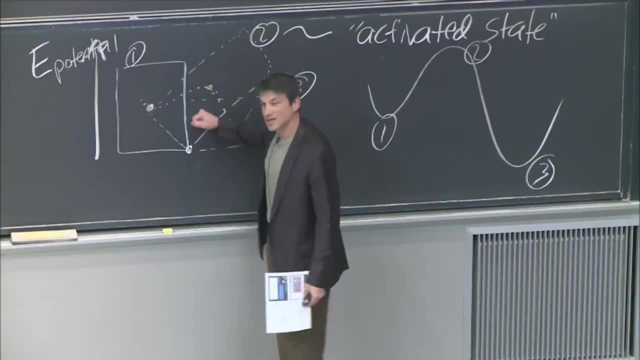 But they're actually hitting it with more energy. They're able to give it more energy. Now you make everyone run really fast And the chances that this thing goes through that process are higher. That's why That's what that is. That's a probability. 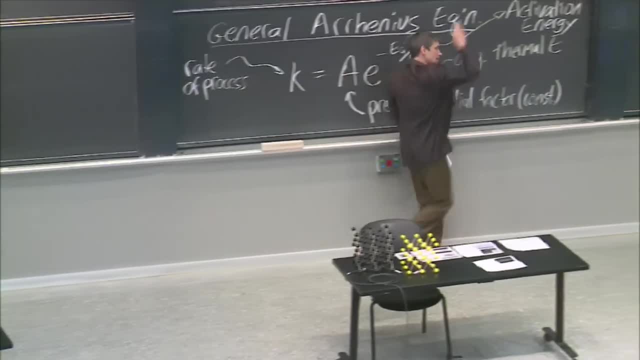 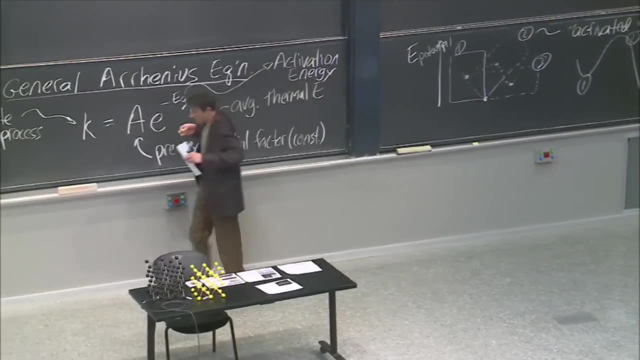 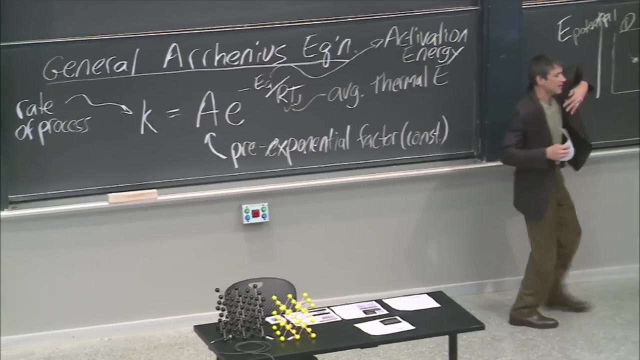 Right. This is what this exponential is. That was the brilliance of what he did, Right. So this thermal energy is like a probability. That's why it goes into an exponential, Because when you increase temperature Again, it's not just that you're increasing how much energy over here. 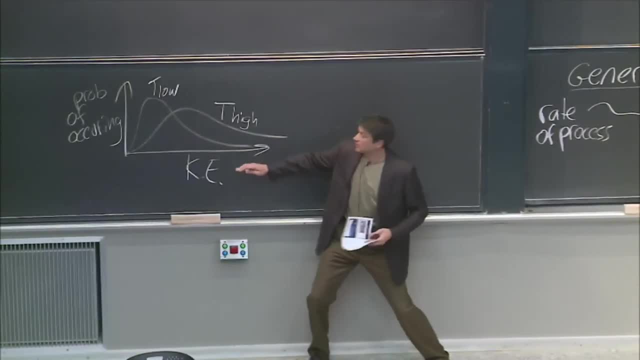 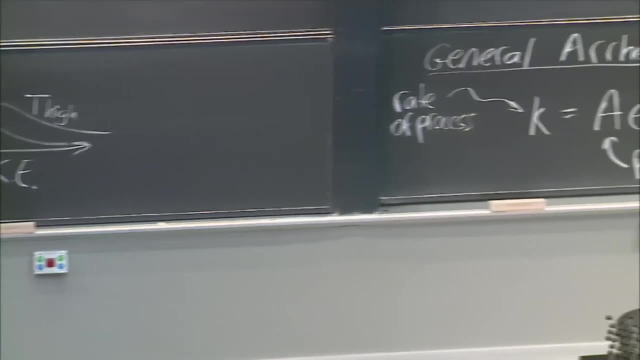 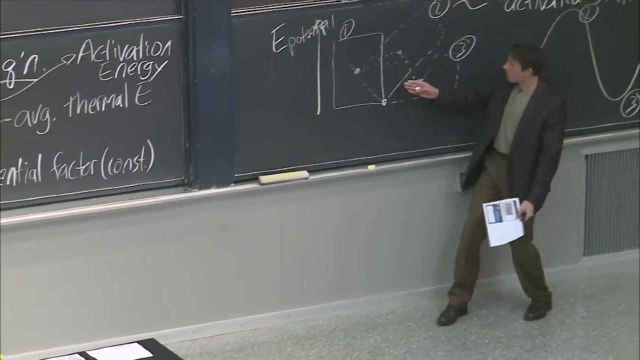 Right, This is like kinetic energy of some molecules. Maybe You're increasing how much energy those molecules have, But you're increasing how many of them are above some threshold. So your chances go exponentially higher. You think, if it was harder and harder to push. 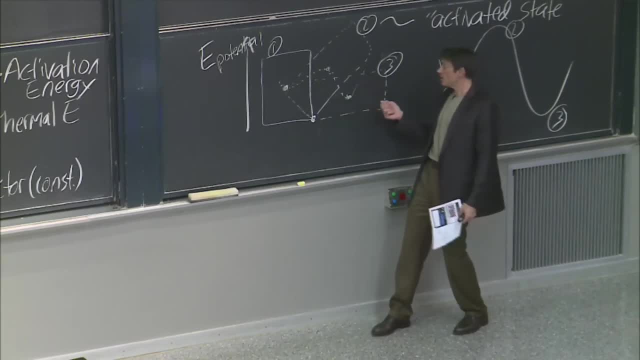 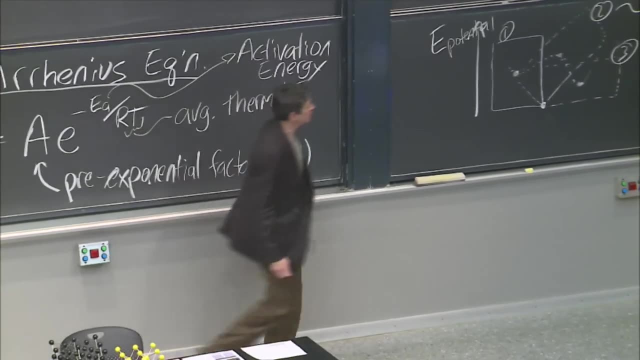 But it's going to go the other way too. You can have. Sometimes somebody might knock it the other way. It looks kind of hard from this picture, But there's a chance. It's just that the activation energy going this way, Right. 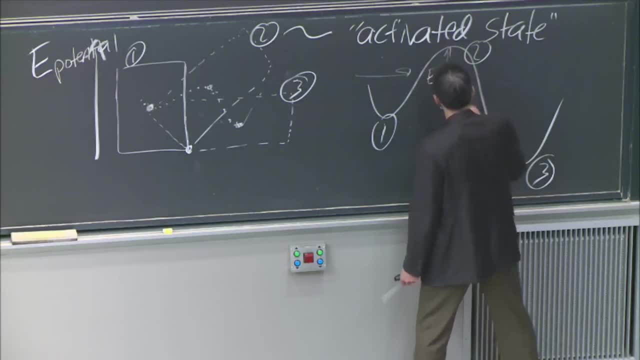 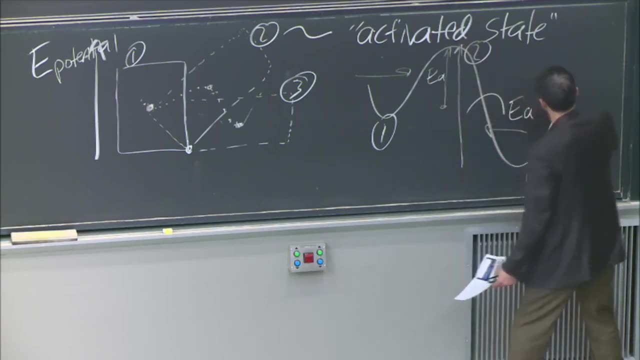 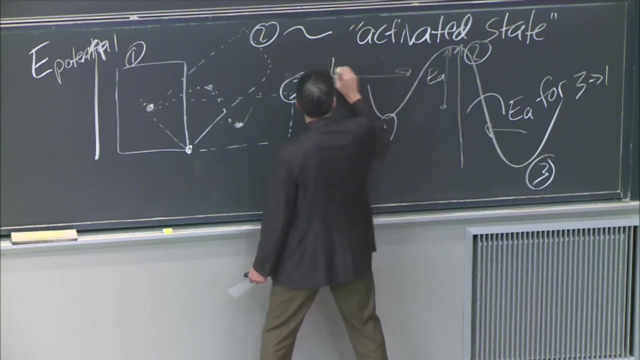 The activation energy is here, Ea And going this way, the activation energy would be here. So this would be Ea for, let's see, 3 to 1. And this would be Ea for 1 to 3.. Now again, I am giving you the general Arrhenius. 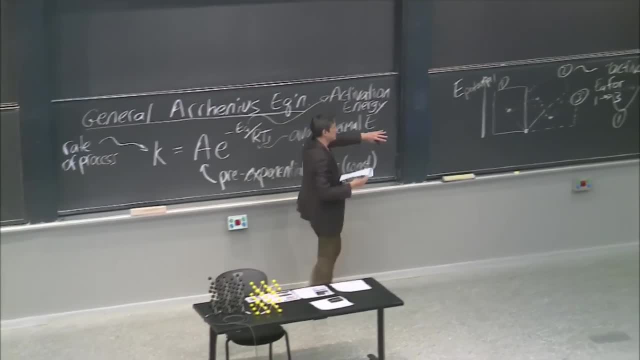 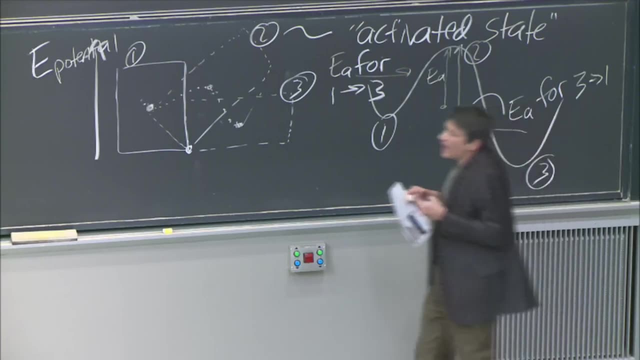 We will be coming back to this when we do reaction rates. We will be coming back to this picture And we will be talking about reactions And then we'll be using that and going to equilibrium. Today I want to give you a sense for what Arrhenius is. 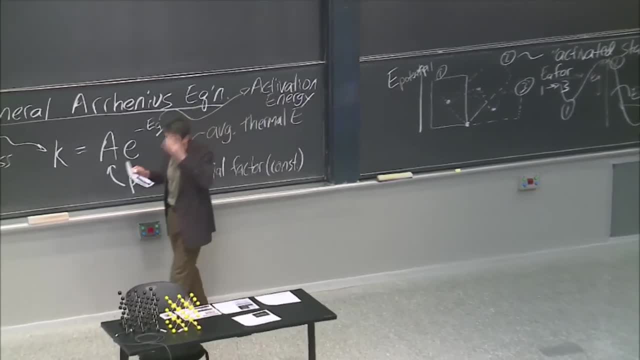 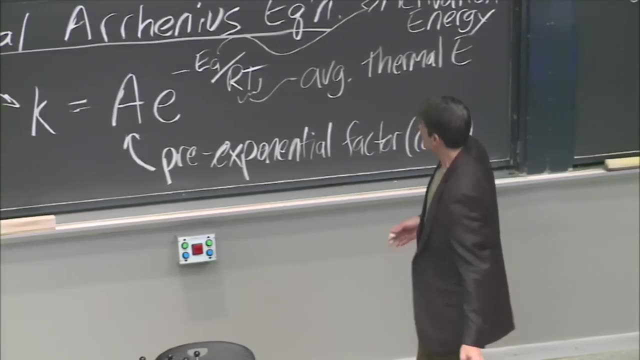 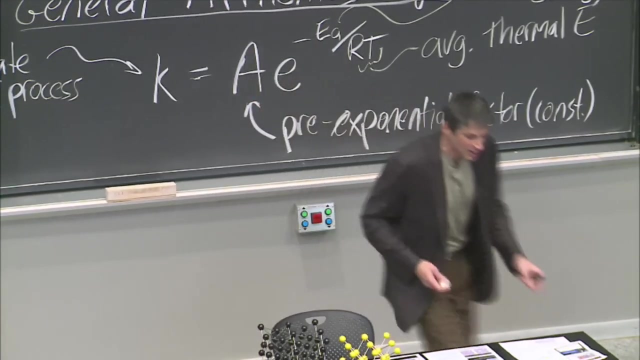 Because this is where the equation comes from, Because, if you think about now defect formation, Defect formation is a thermally activated process, But that's exactly the point. So that's why, if we write this down- I've said this now multiple times- 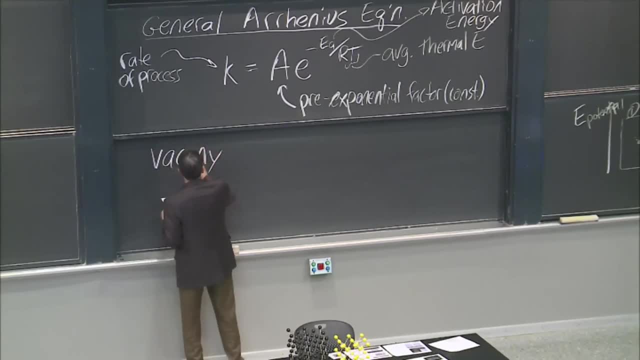 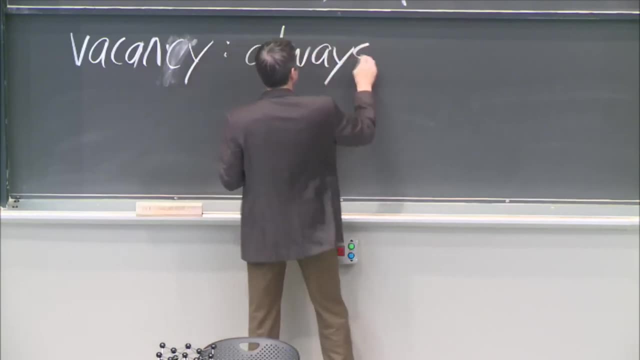 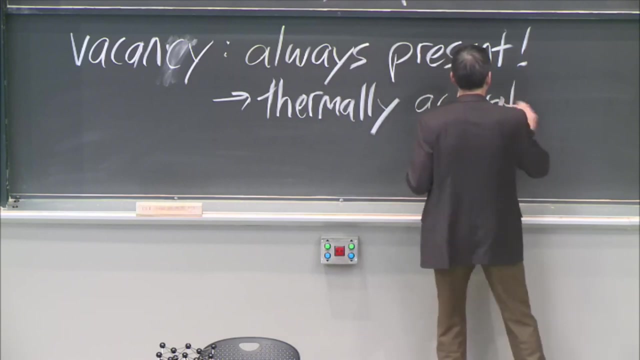 The vacancy Vacany. No Vacancy is always present, Always present. Why? Because it's thermally activated. So unless I can get to, t equals 0, thermally activated, There's always a chance that I push a vacancy into the material. 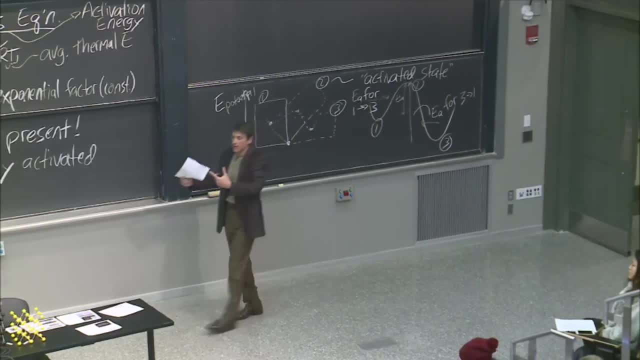 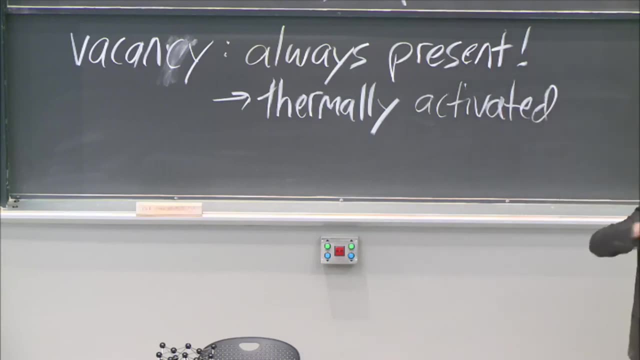 There's also always a chance that the vacancy gets pushed out. So those are happening because of temperature. You can think about that. It kind of makes sense, right? Atoms are moving. Those are the people, right? Those are the people in the room. 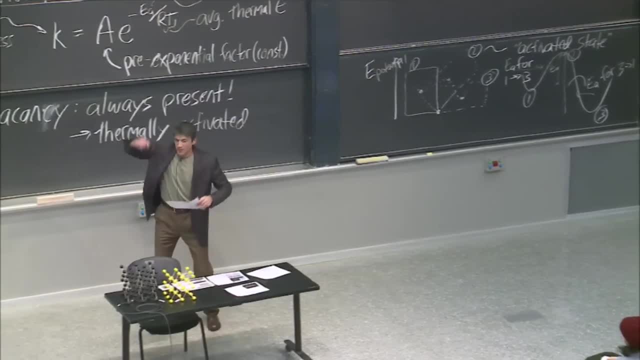 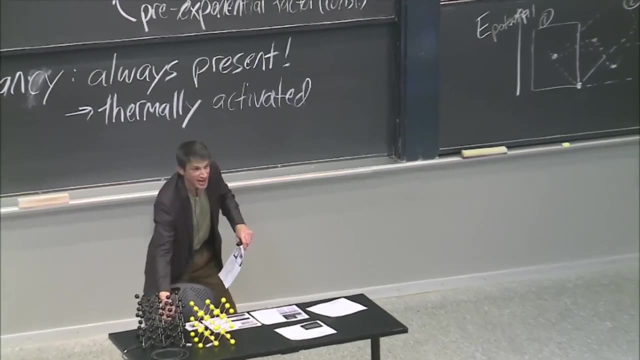 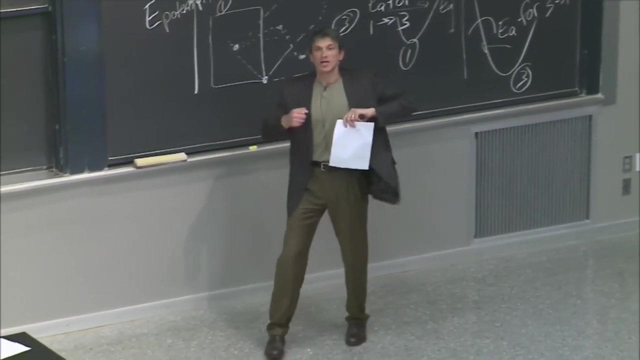 And now, all of a sudden, something happens somewhere that allows an atom to come out- We'll talk about that in a second- And create a vacancy. Now there's a chance that it can go back too, And so at some point there's an equilibrium concentration. 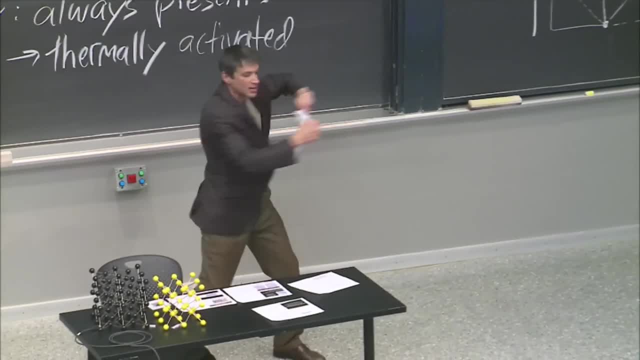 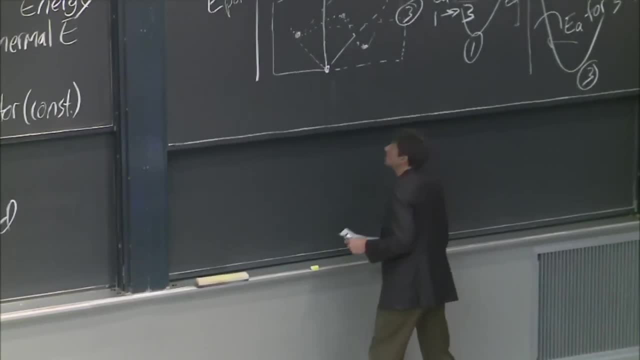 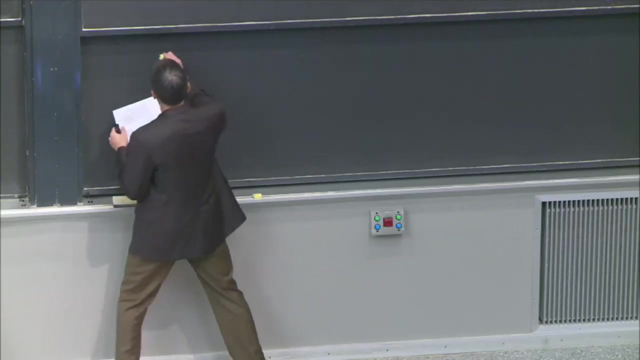 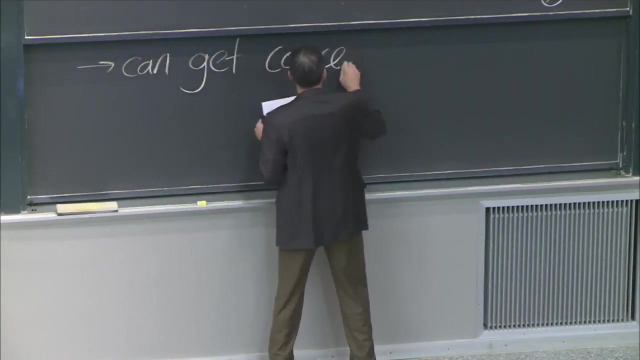 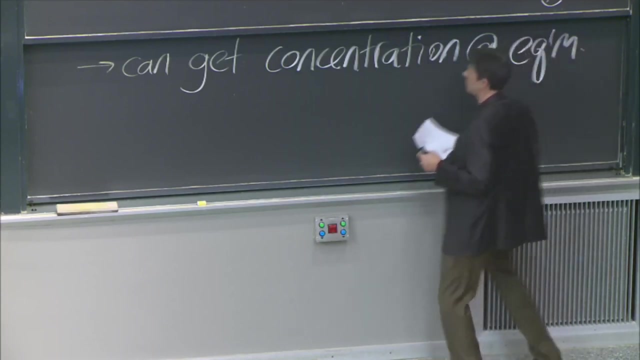 Both of those are thermally activated processes that have an Arrhenius-like behavior, And so you get to the very nice expression for concentration. So you can get concentration. So the concentration at equilibrium since vacancy formation is thermally activated and it's thermally deactivated. 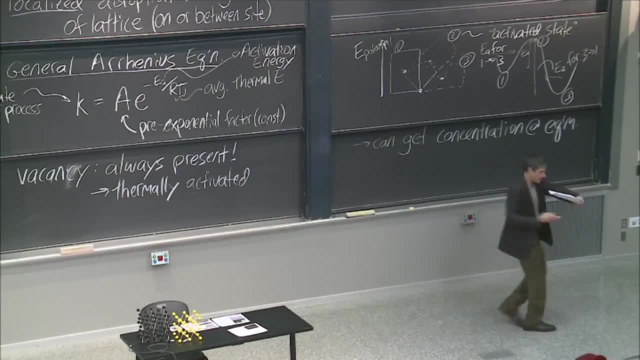 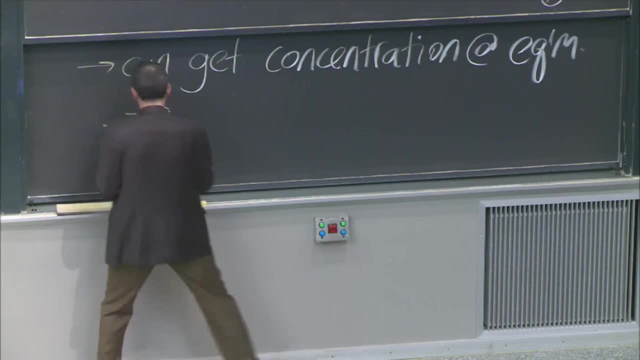 you can say: well, when it's activated and deactivated in the same rates, you're in equilibrium. That's how you get a concentration And I don't need you to know the math, But I need. This is where it comes from. 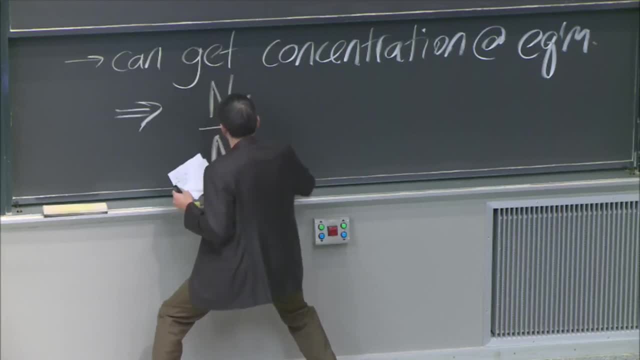 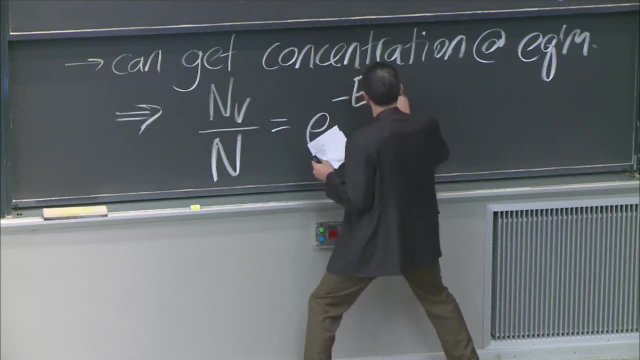 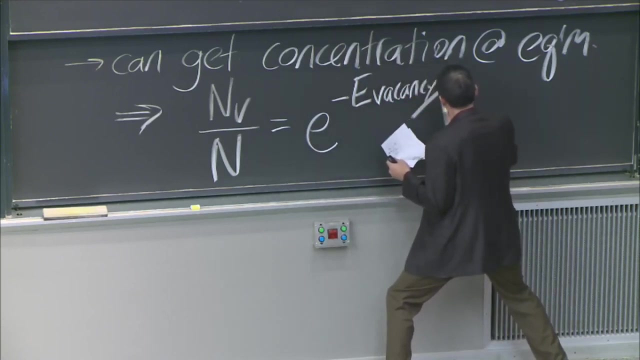 The number of vacancies divided by the total number of sites is equal to e, to the minus e vacancy. I will talk about this Vacancy divided by. Let's use RT, still RT. Now, here's the thing about RT. Let's write this down because this is really important, right? 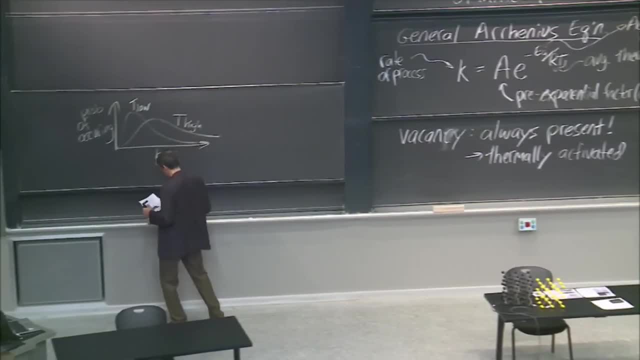 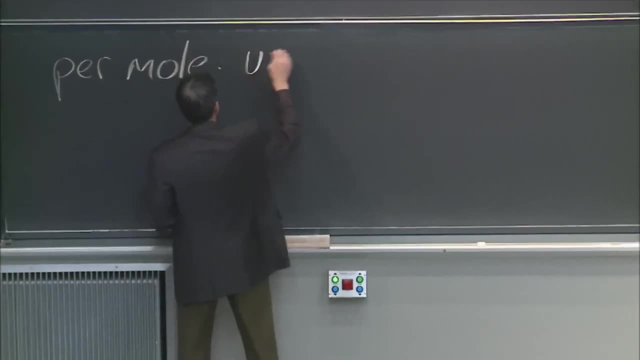 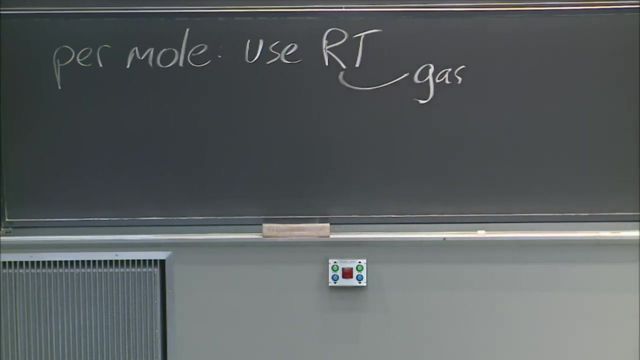 We talked about this before. If I'm using RT, then If it's per mole, Per mole, use RT. This is the ideal gas constant right. That's not just used for ideal gases, It's used for a lot of things. 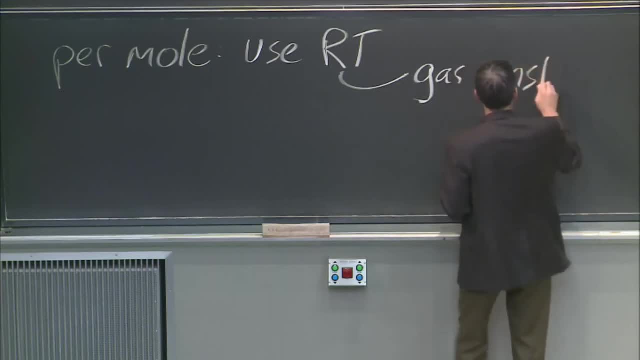 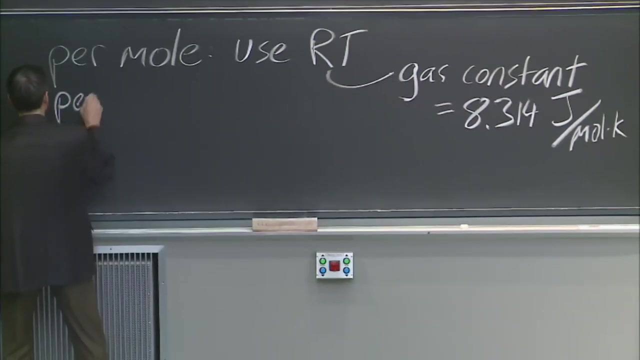 That's the gas constant. Gas constant, That's equal to- Let's see if I have it down here- 8.314 joules per mole Kelvin. So you see, if I'm working in per mole, Then I use R. 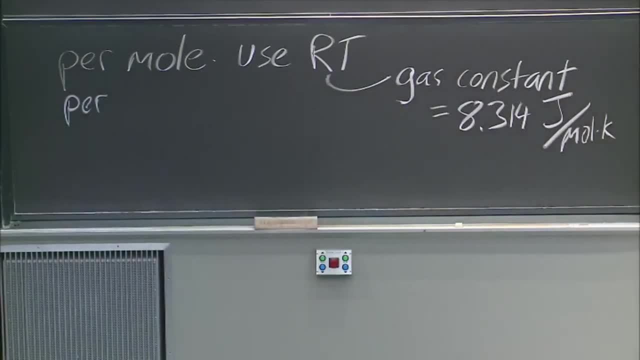 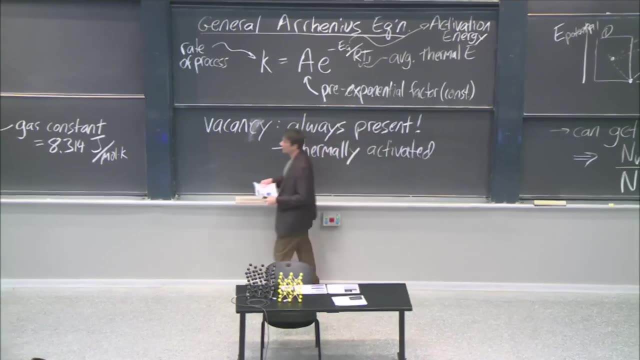 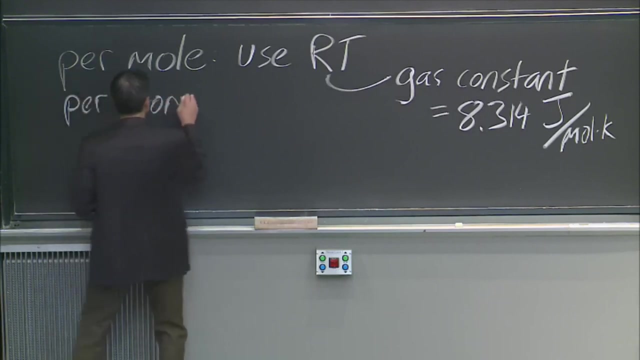 This is in the energy unit. Those energy units have to be the same. They got to. So if my activation energy is in per mole, Fine Use the gas constant. If the activation energy is in per atom, Then we just use the Boltzmann constant. 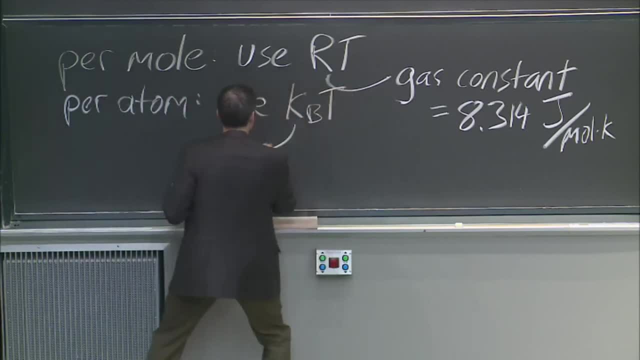 KBT, Where the Boltzmann constant is something We have seen. It is equal to the ideal gas constant Divided by Avogadro's number. Remember that Avogadro's number goes in and out Atomic, Macroscopic worlds. 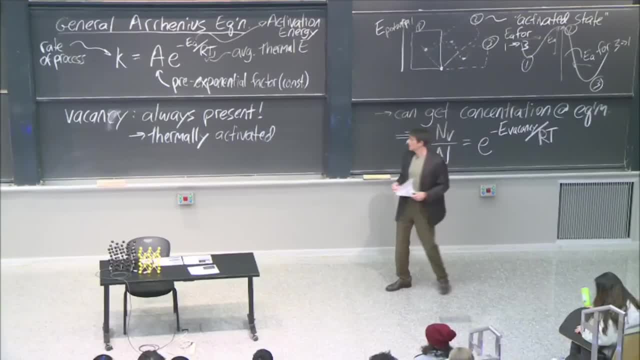 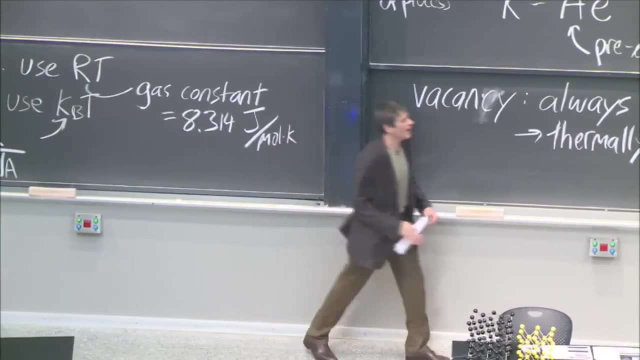 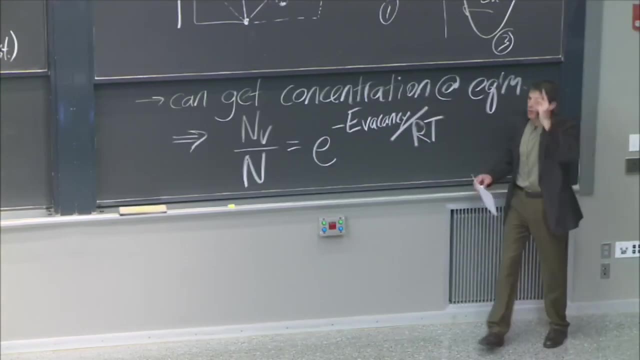 So R and KB: Same thing. Okay, One thing Notice: that's per Kelvin. Whenever you have equations like this, That come from thermodynamics, Which is where these things come from. There is only one temperature unit, There is no other. 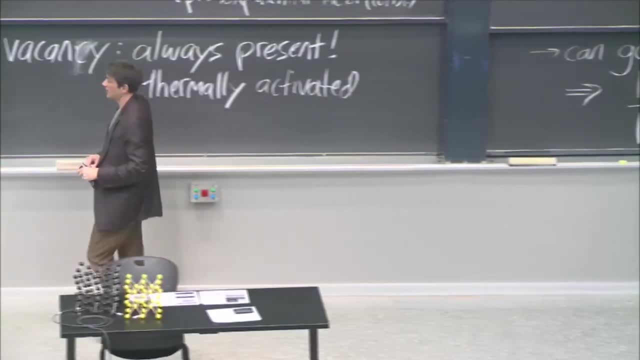 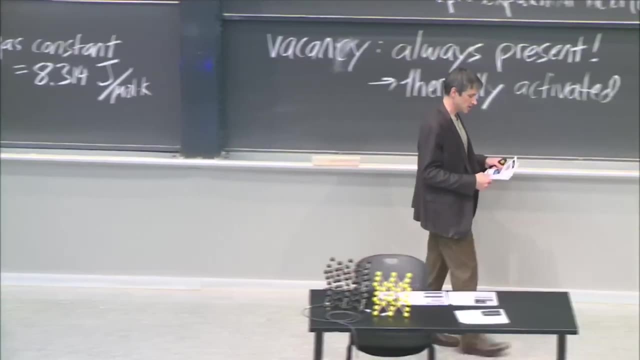 And it is Kelvin. You have to be aware of that. If you see something in Celsius, It's not going to work, It's got to be Kelvin. All of these equations Have to use Kelvin. Okay, So that Now you can see. 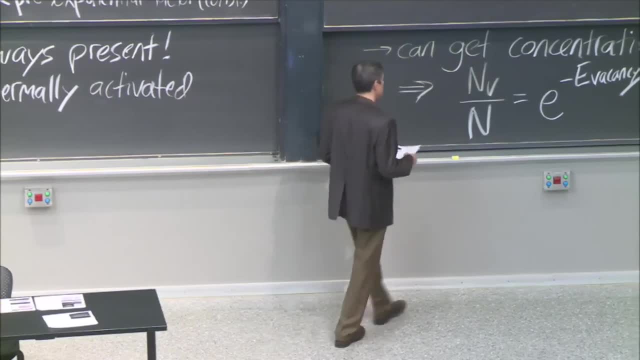 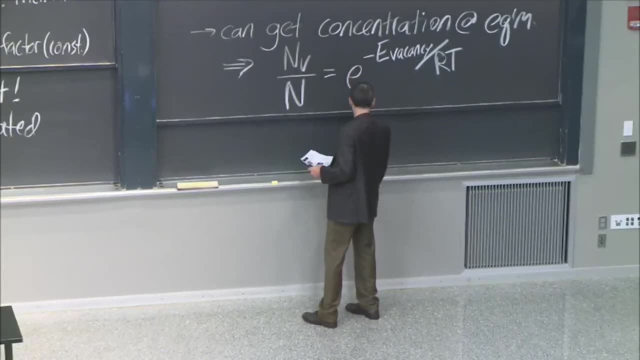 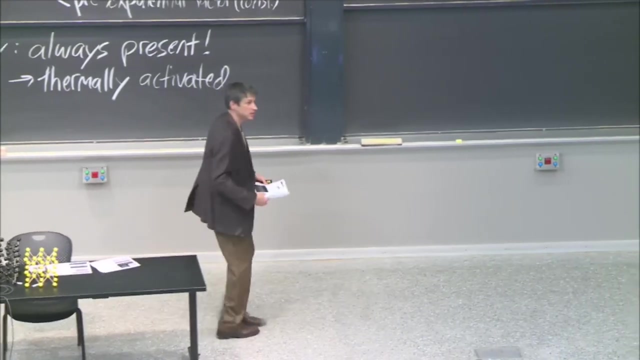 Any time, You know, Any time you see An equation with an exponential, What's the first thing you want to do? I mean, It's like, It's almost like a, An instinctual reaction. You see an exponential. Take a log. 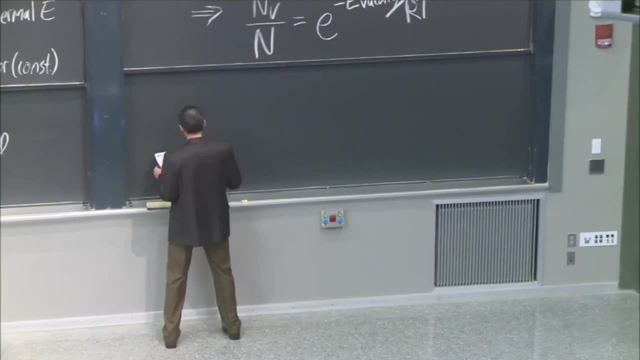 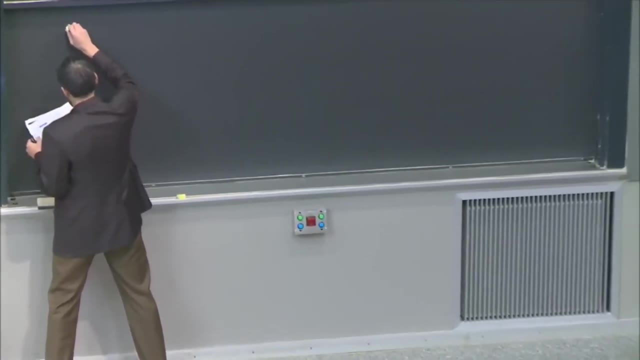 Don't say anything Until you Take a log. Right, So that's So that. So we're talking about Energy, of the vacancy in a minute, But if you take a log of this, Then you get that The log. 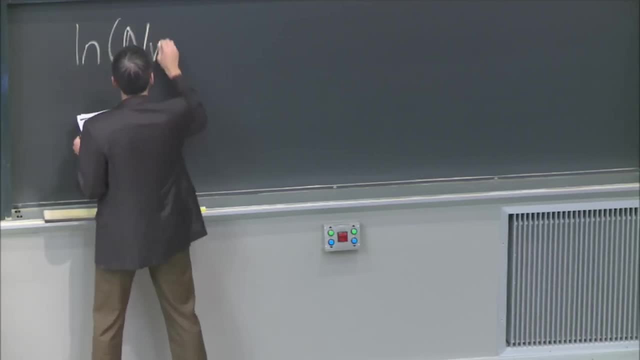 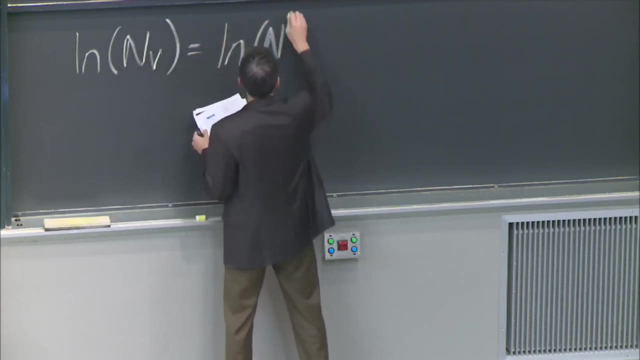 Of What Are NB and N. Well, I'll talk about that. Equals. Log Of N. Let's do it this way. Okay, Let's do it this way, Minus: Log Of N. 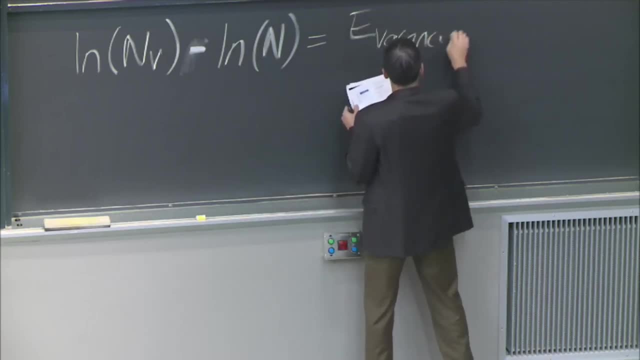 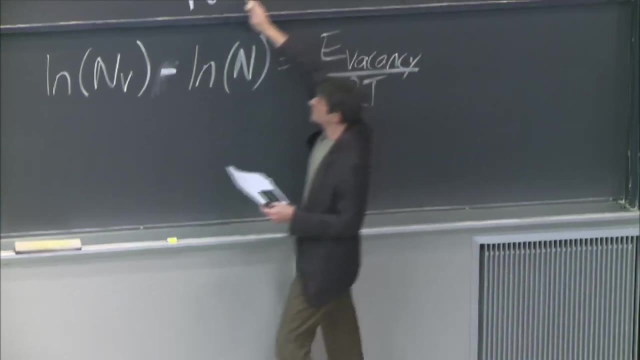 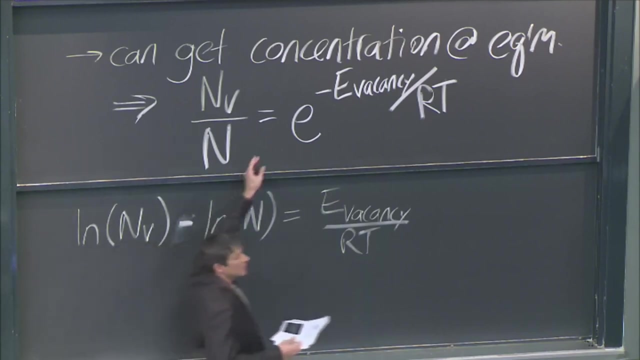 Equals E: Vacancy. Okay, Divided By RT. That's Just Taking An Exponential, A Log Rhythm Of This Equation And Now I Can Talk. 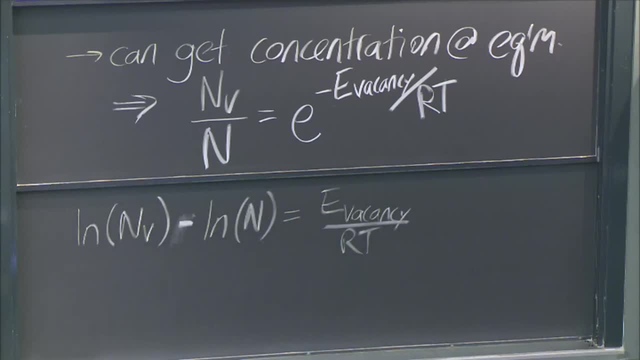 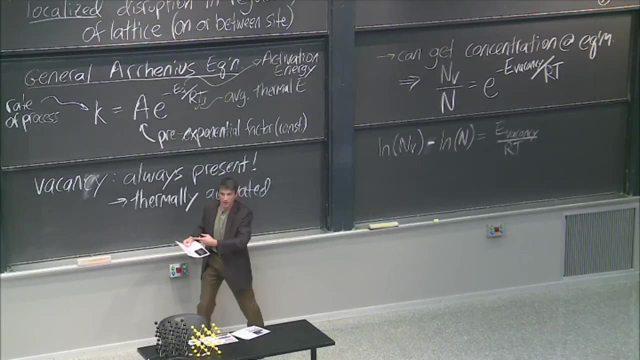 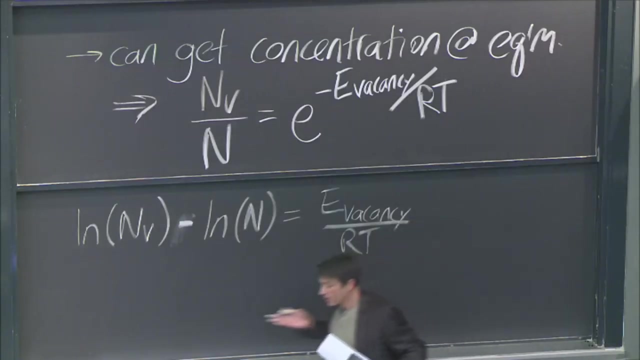 About The Constant. Canceled This Pre-exponential Factor, Canceled It. Canceled Because I'm Taking A Concentration, I'm Looking At The Rate Going One. 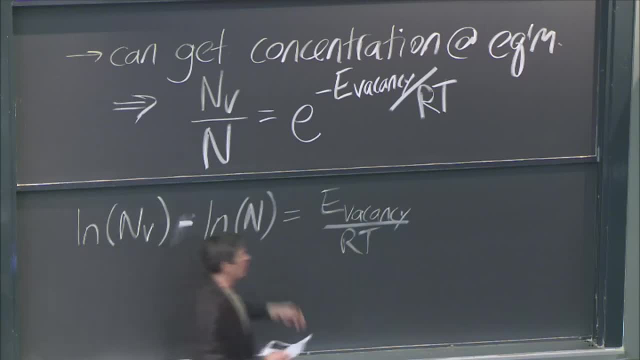 Way And The Rate Going The Other. And It's Not A Rate, It's A Concentration. It's Okay, It's A Concentration In Equilibrium. 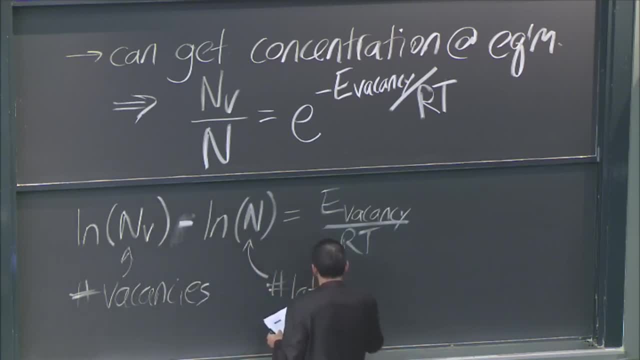 So This Would Be Like The Number Of Vacancies. Number Of Vacancies And This One. Okay, Here's My Crystal And Here It Is I. 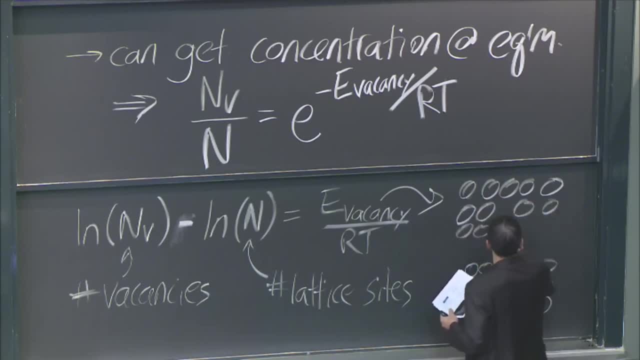 Think I'll Stop Here, And Now I Did This. We're Going To Go Graphical And This And This. That Energy Is, Yes, There Is. 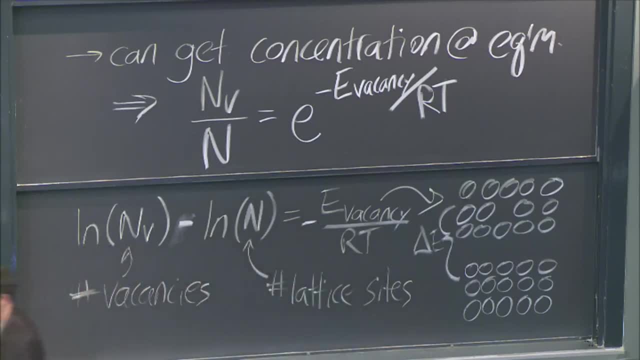 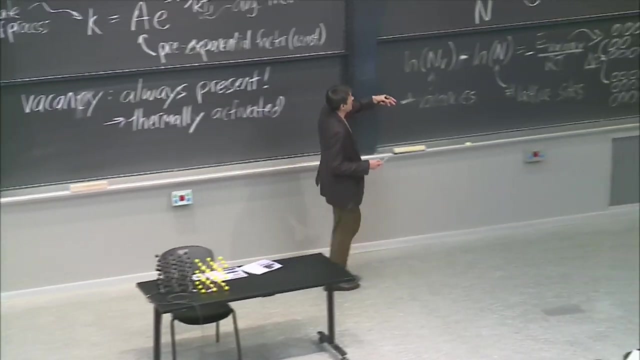 Yes, There Is. Thank You Very Much. Yes, So That's Okay. So Now, The Energy Difference Between Having A Vacancy And Not Is The Vacancy. 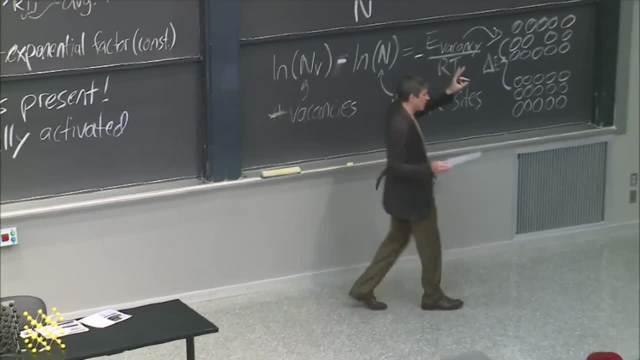 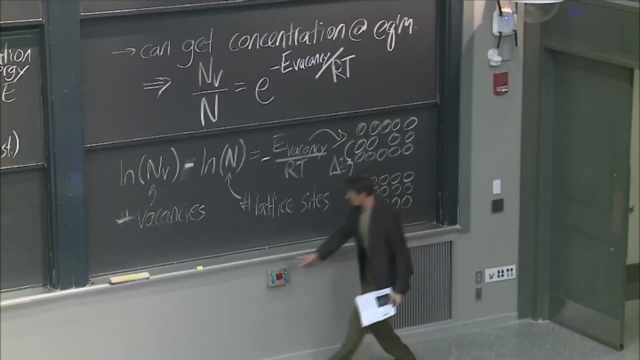 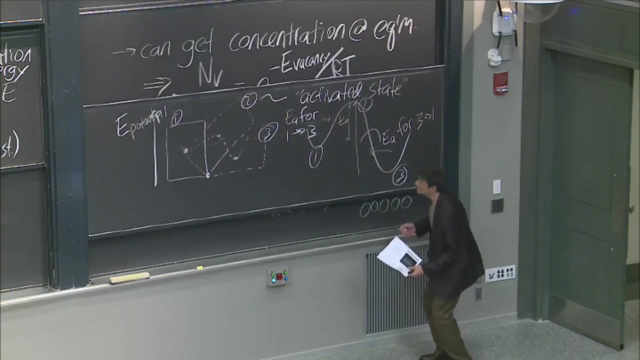 Formation Energy. That's Fine, I Mean It. Just It's Written That Way To Get Across The Point That It's An Arrhenius Like Behavior. 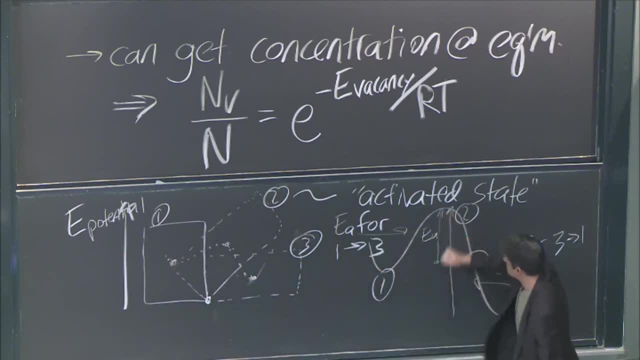 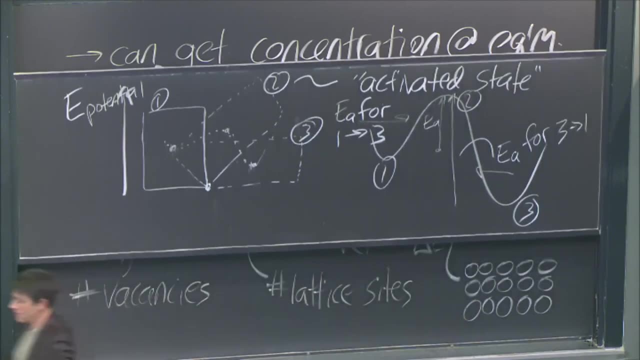 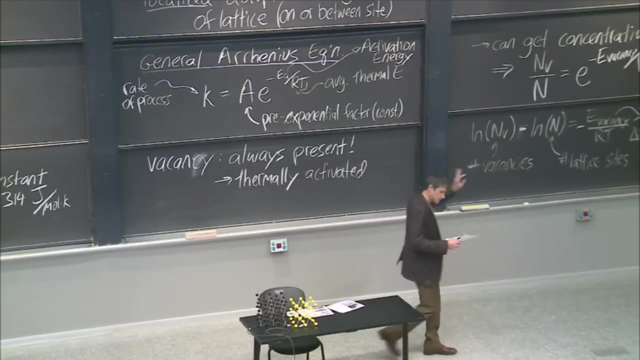 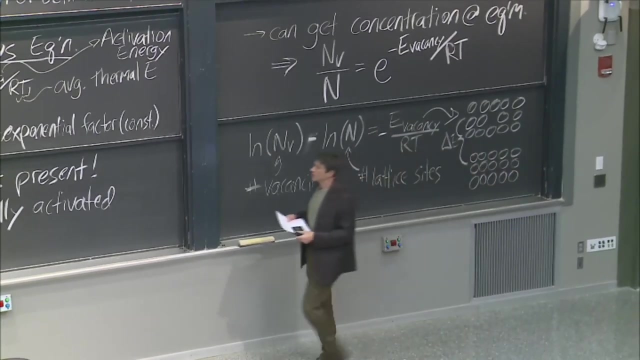 But Actually The Act, If You're Clear. So So The Formation Energy Between Having A Vacancy And Not, Is What Goes Into Our Equation All. 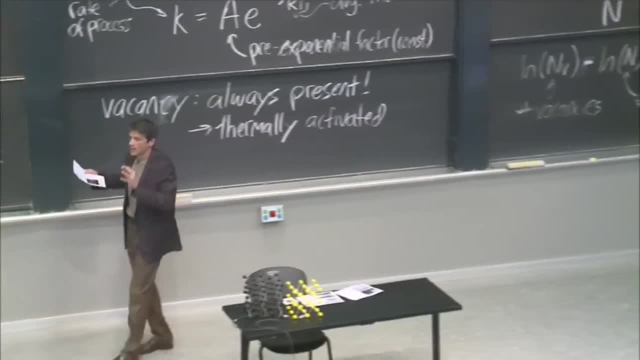 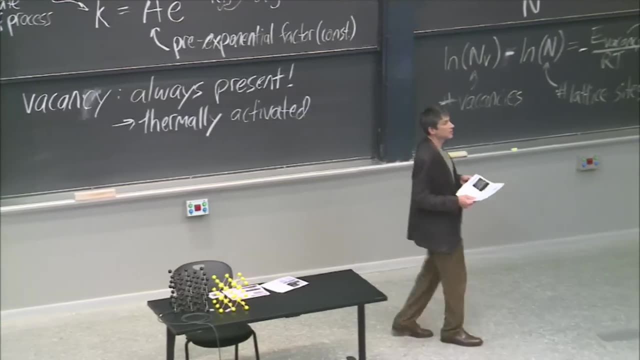 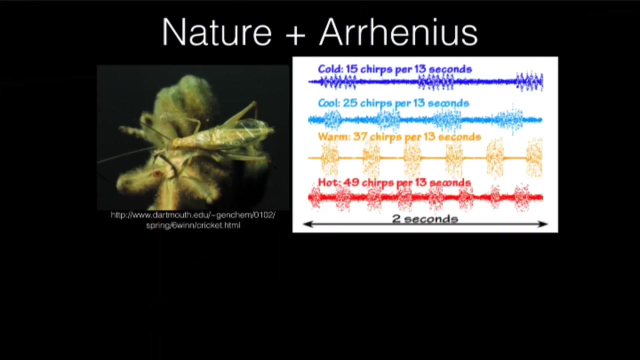 Right Now We're Going To Use This, So So We Will Do This With Live Crickets- And Actually I Really Hope Not, But This Is. 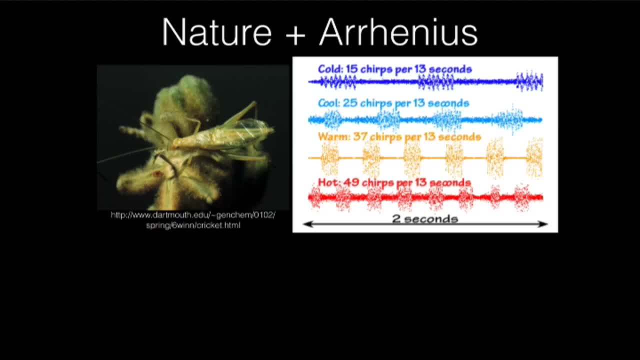 One Of The Labs That They Have, Where They Take Crickets And They Measure The Cricket They Do. Well, They Didn't Know About Arrhenius. 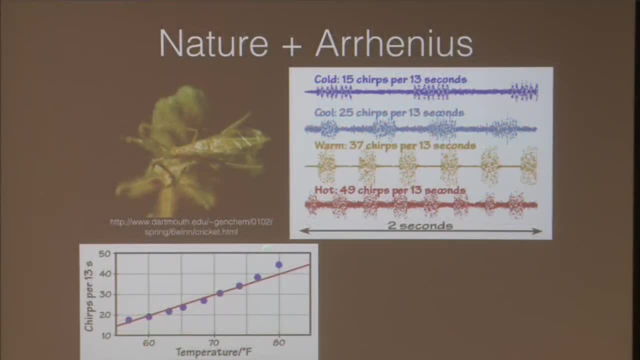 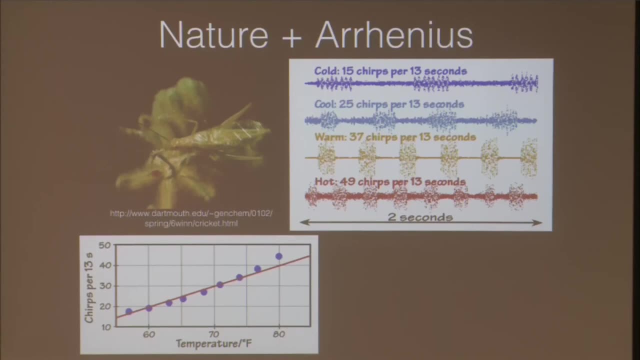 Yet Until Somebody From MIT Went And Visited. So The First Thing They Did Is They Plotted The Data. Look At The Cricket Tripping. 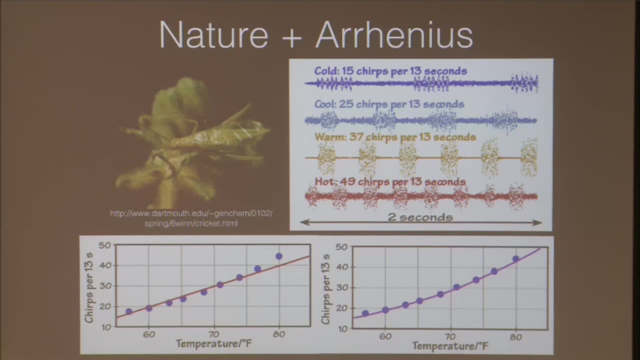 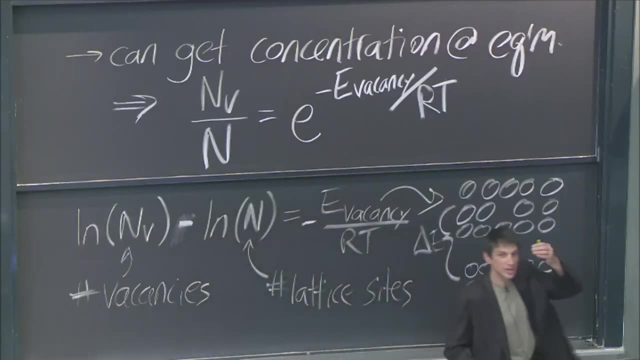 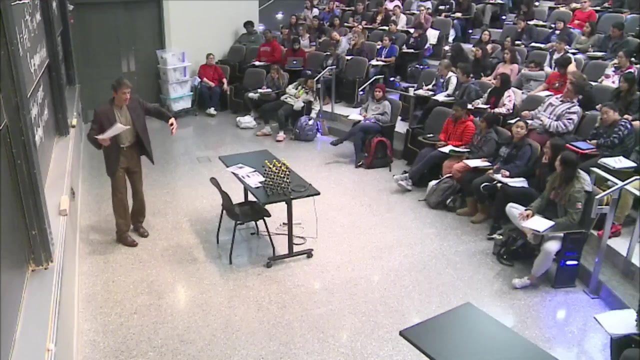 Beautifully, And You Can Go Even Further Because You See If You Got This Far. Well, Now You See, This Is A Line, This Is. 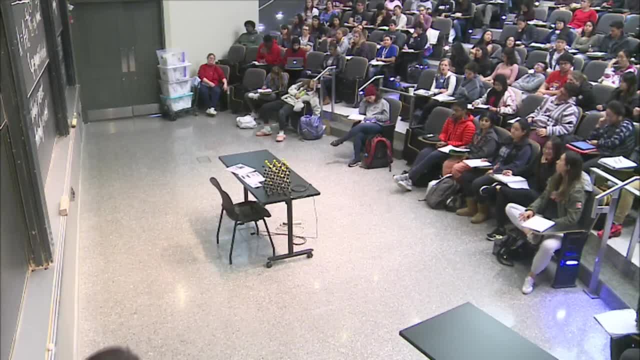 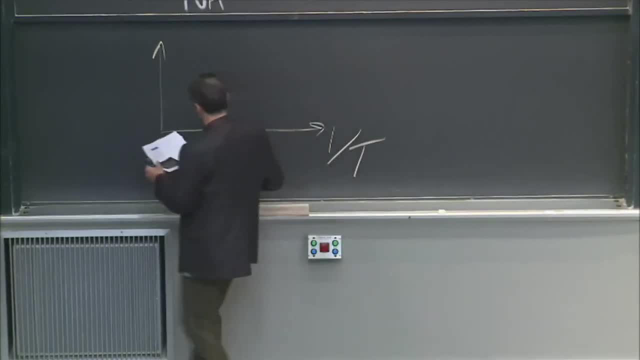 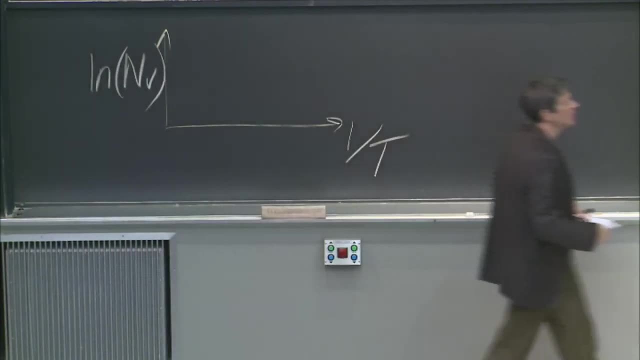 A Line And You Can Do It There. But You Know, You Could Plot. For Example, You Could Plot One Over T Versus The Log. 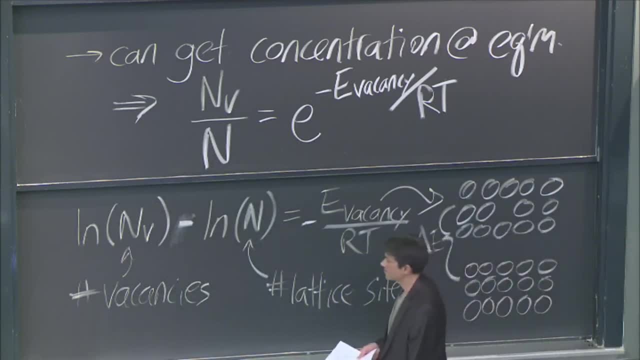 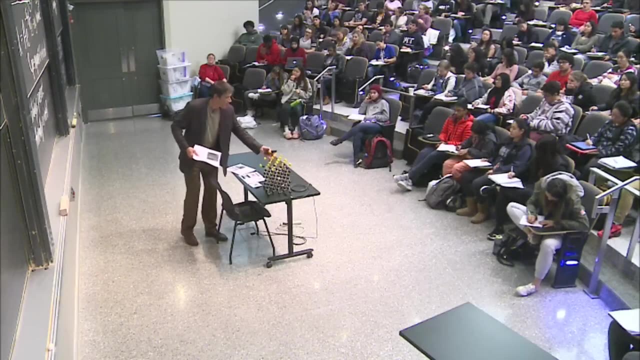 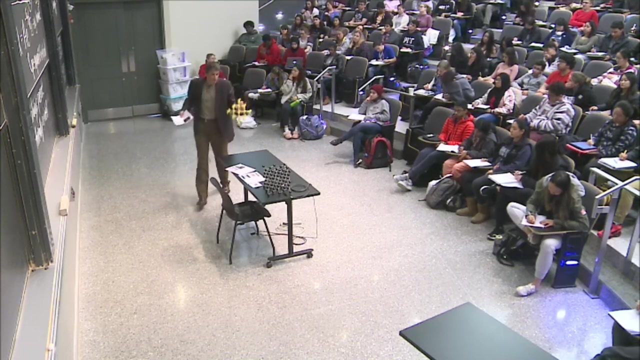 Of The Number Of Vacancies, But The Number Of Lattice Sites Is Simply How Many Lattice Sites You Have, In Whatever Volume You Have. 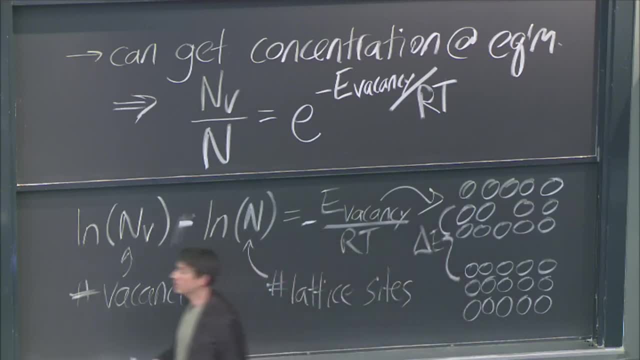 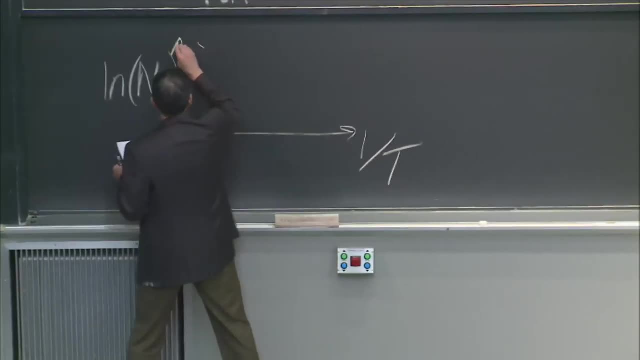 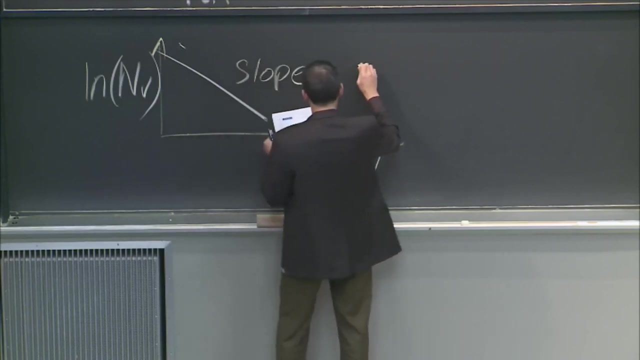 For Whatever Crystal Structure You Have, For Whatever Element, You Have A Linear Line And The Slope Of That Line Is Equal To Minus E. 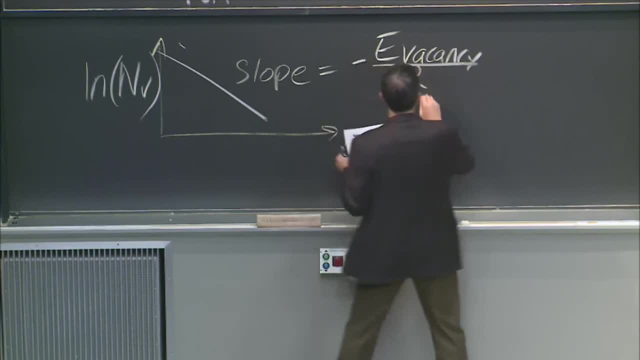 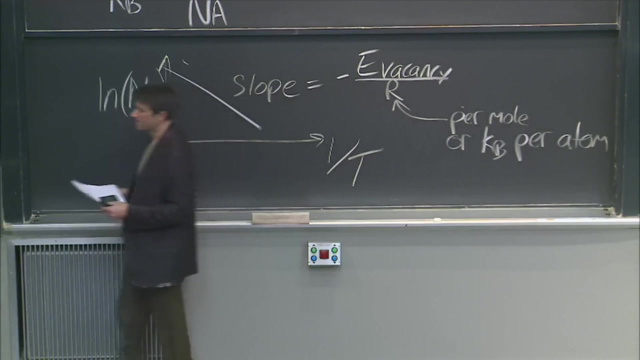 Vacancy Divided By R, Or It Could Be Kb R. Let's Write This Again, Per Mole. Let's See Both And This, This Intercept. 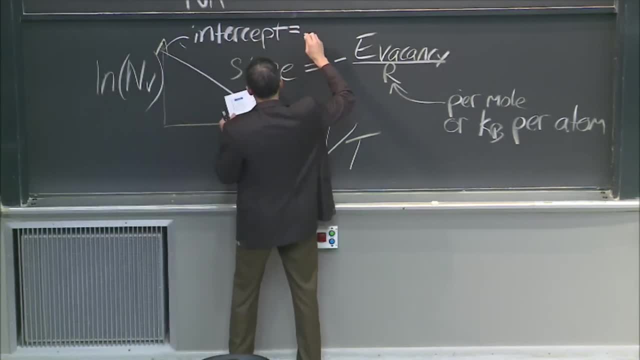 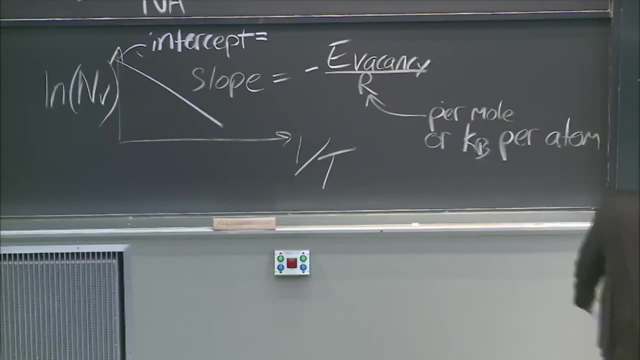 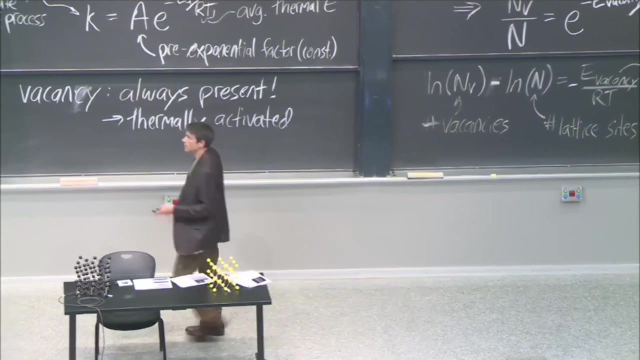 Intercept Is Equal To The. Let's See, The Intercept Is Equal. What Do I Have Here? The Log Of N? Did I Write? What Can? 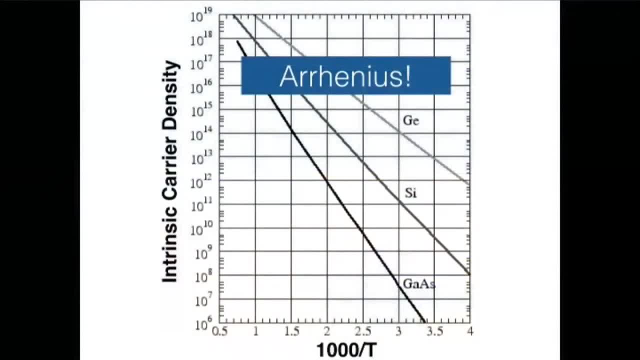 You Do Well, Before We Go On To The Defects, This Explains The Doping- I Kept Calling The Doping In Semiconductors. 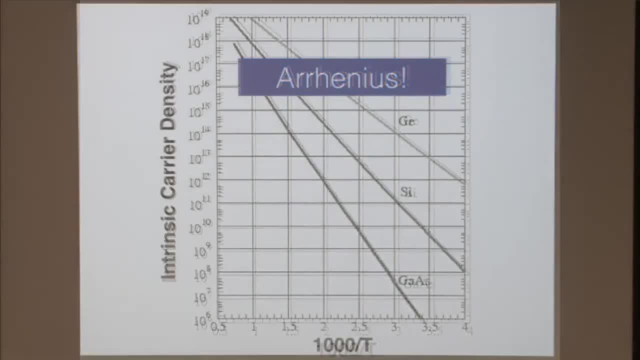 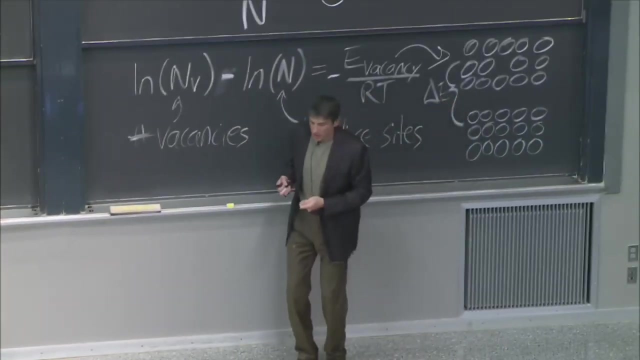 A Thermally Activated Process. But Look, And The Reason Is Because It's A Thermally Activated Process And, In Fact, In This Case, What? 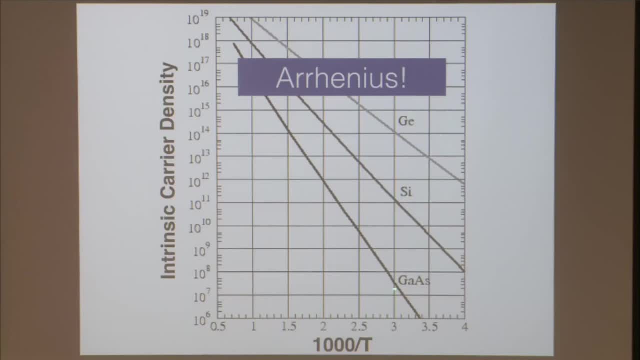 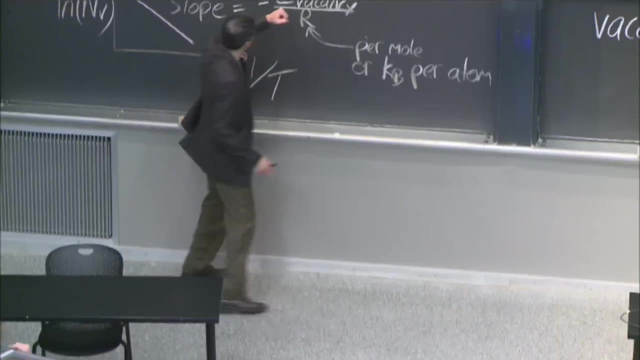 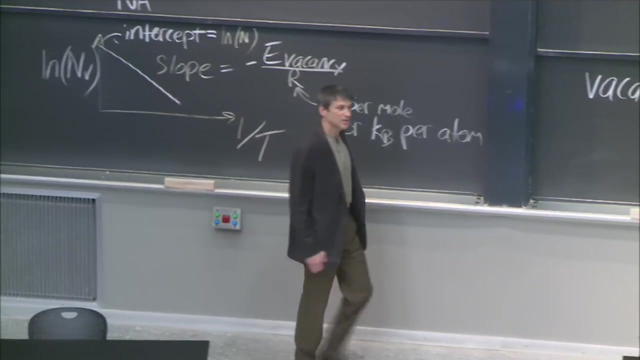 Is The Activation Energy Right. The Activation Energy For Getting An Electron In That Activated Process Is The Gap. That's Why The Slopes Are. 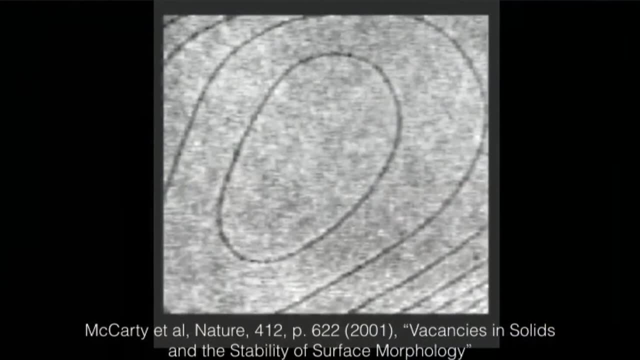 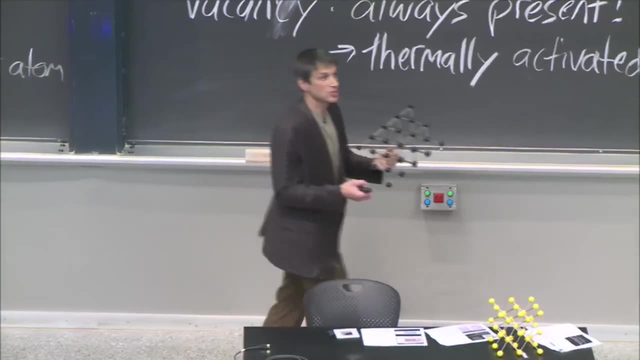 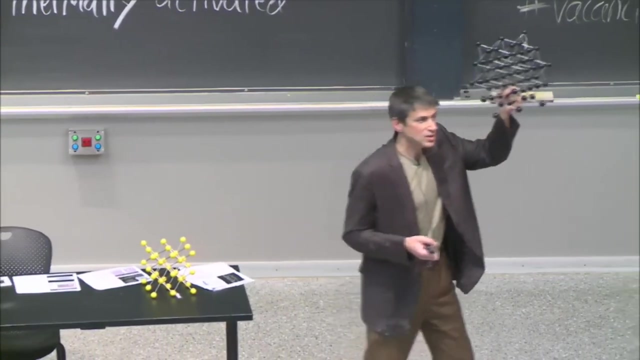 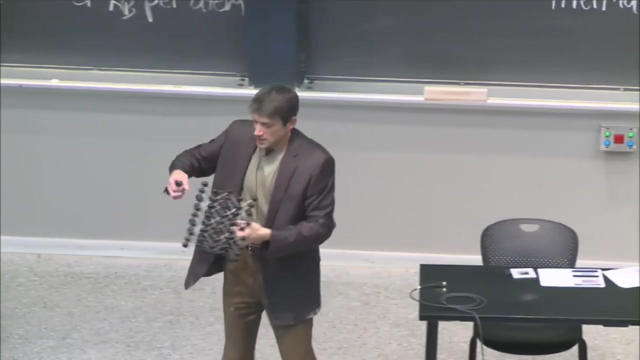 Different Right. Okay, All Right Now On To. Oh No, I Didn't. I Did Want To Mention You. It's A Call Out To The Surface. 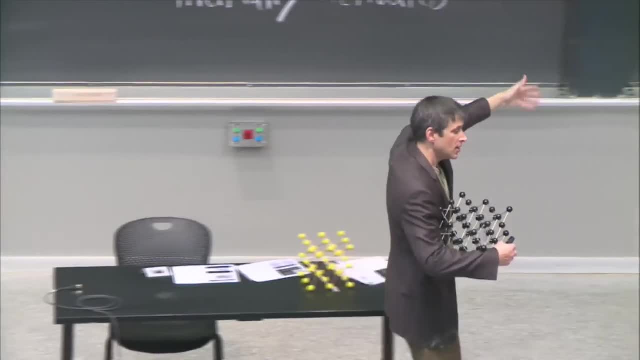 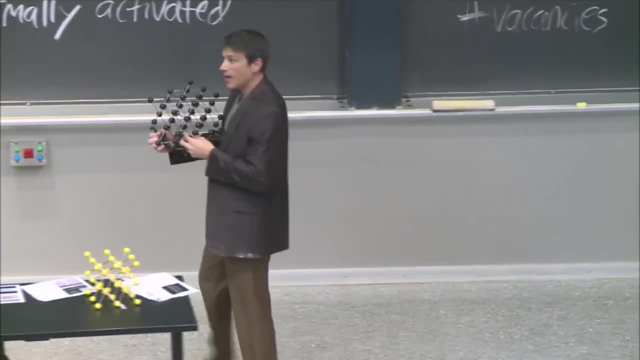 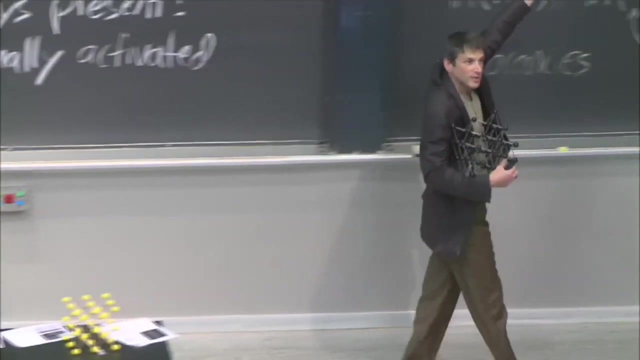 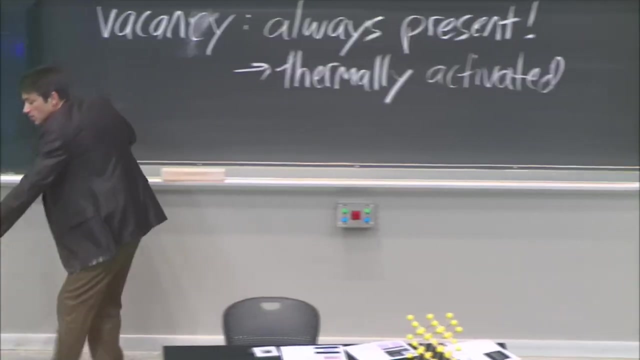 Or Maybe The Surface Calls In. It All Has To Happen On The Surface, So What Ends Up Happening Is A Surface Atom Could Go. 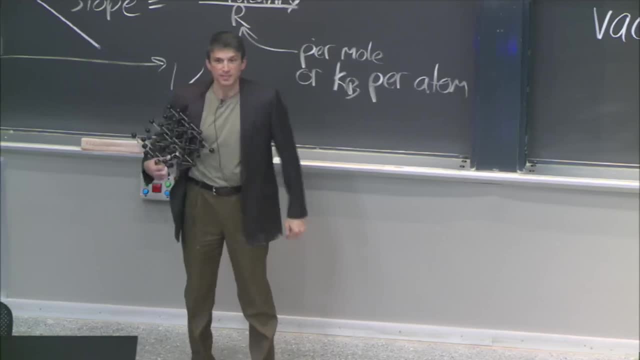 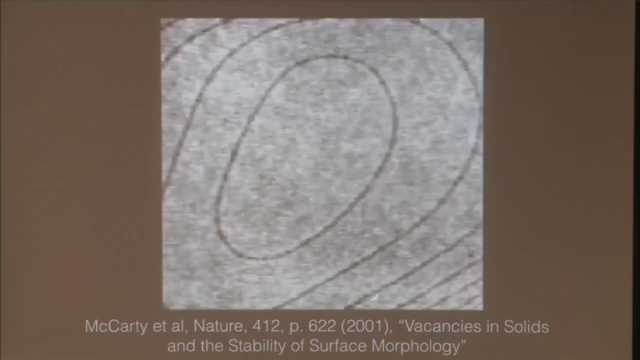 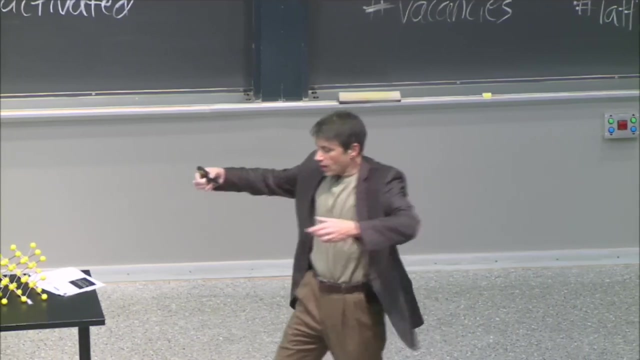 In To The Crystal So That Some Atom Inside Is Able To Fill A Vacancy. It All Comes From The Surface. This Is A Beautiful 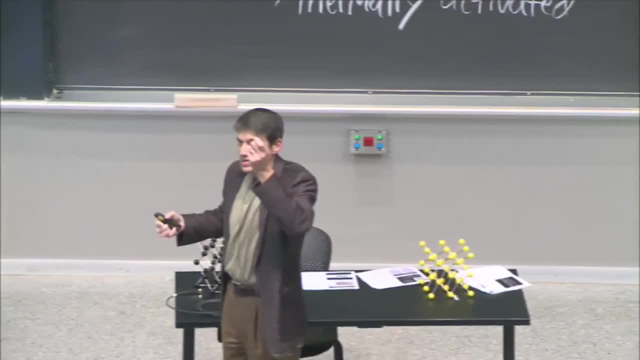 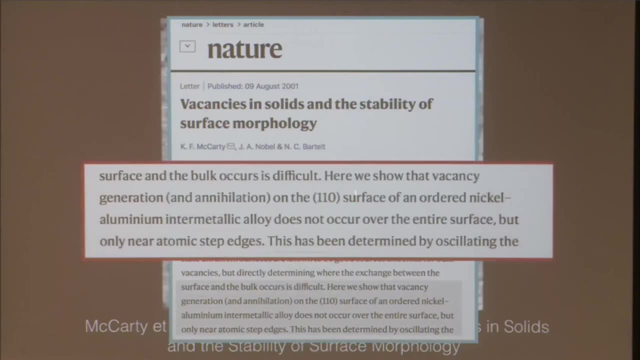 Island Going And Where Are They Coming From? Vacancies? It's All About The Vacancies, Right, And One Of Things I Loved About This Is: 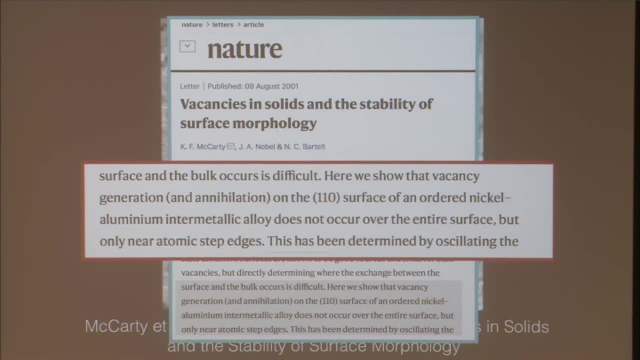 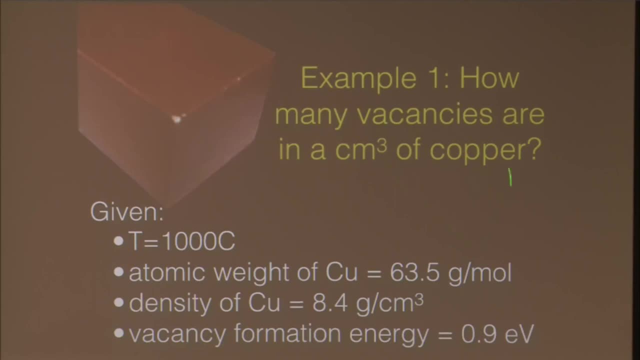 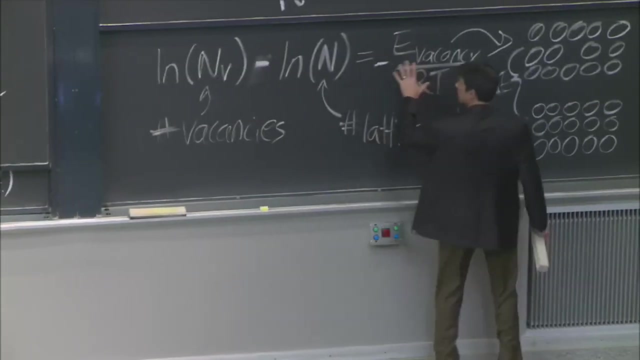 The Abstract Of This Paper. Okay, And Now We Got To Make Vacancies Right, And So This Is The Kind Of Problem You Might Get. 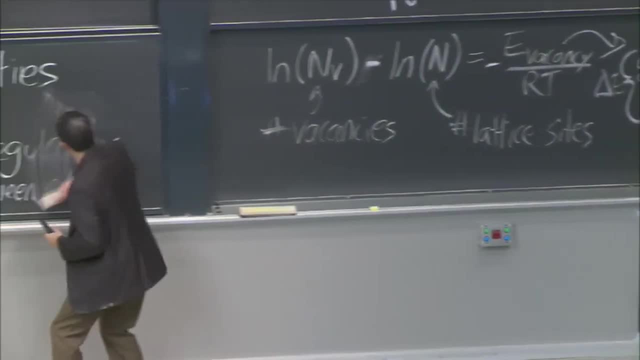 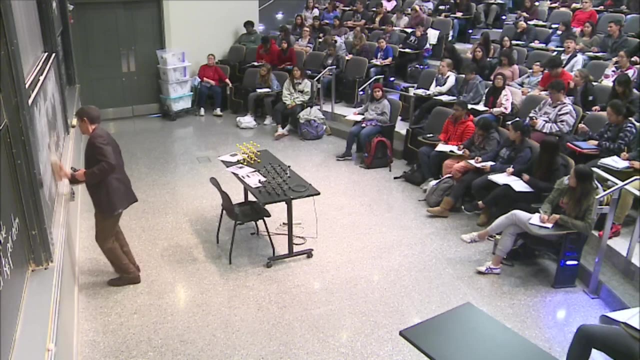 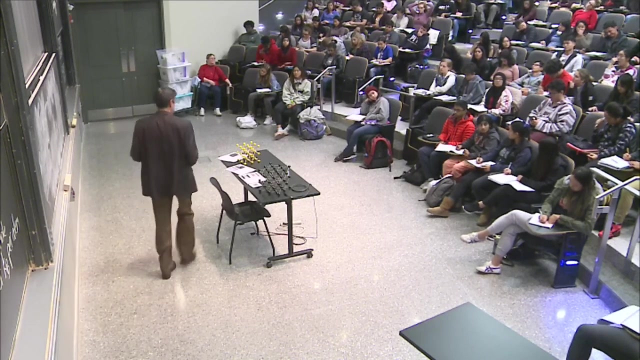 How Many Vacancies Are In A Centimeter Cubed Of Vacancies That You Can Now Answer, That You Know How To Think About Vacancy. 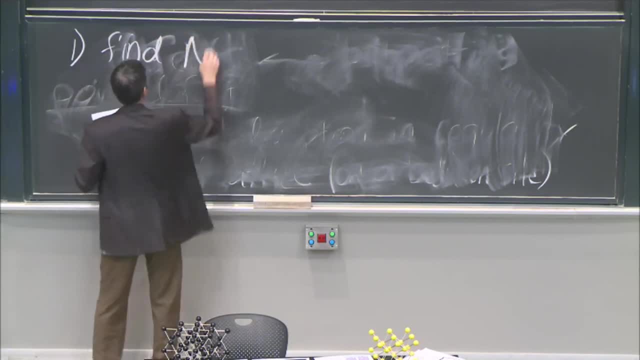 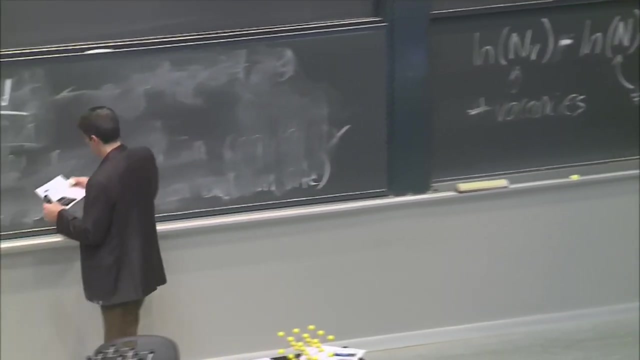 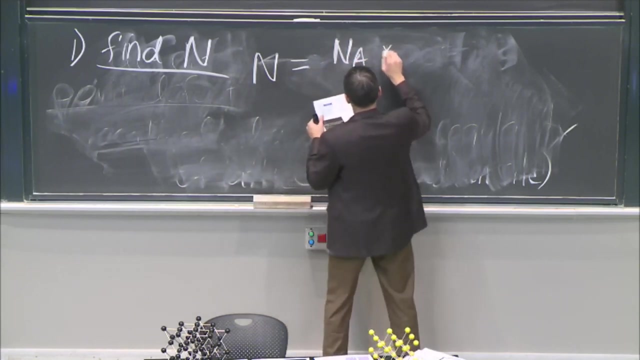 Formation. So For Example, In This One You've Got Step One. Step One, You Would Find, And So Step One. Well, So Step One, You'd. 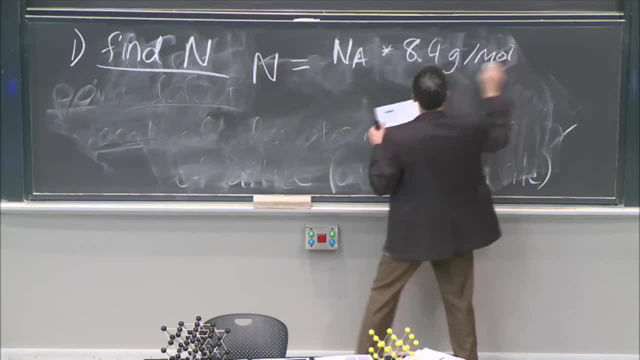 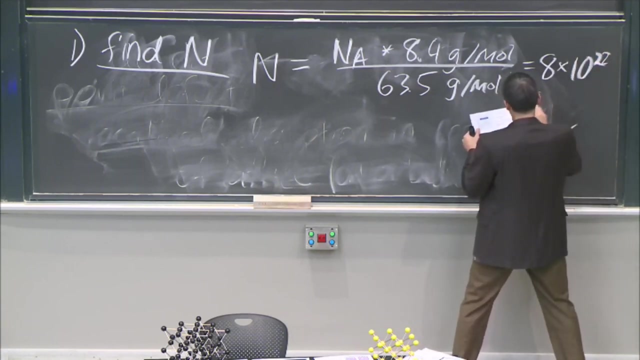 Say N Equals Avogadro's Number Times Eight Point Four Grams Per Mole Right Divided By All. This Is Such Old School. Why Am? 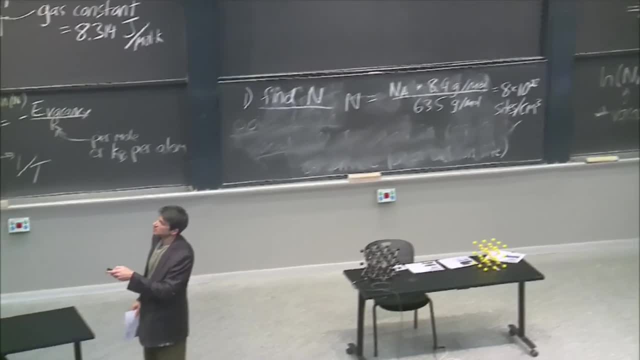 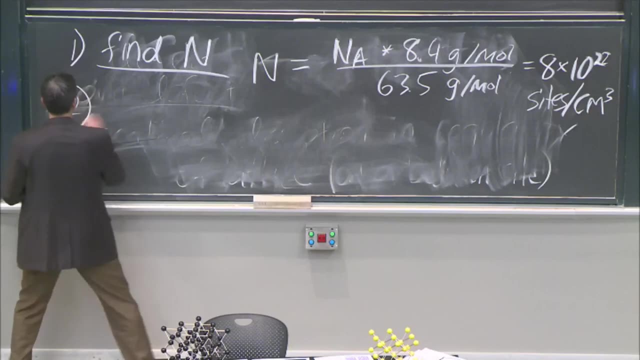 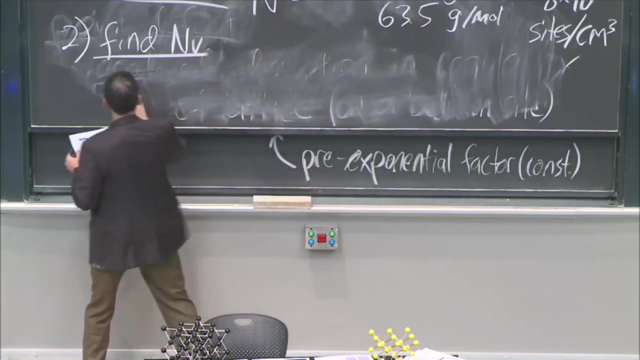 I Using Centimeter Cube Well, Because That's What I Was Given The Density In, So I'm Just Leaving It In Those Units For Now. 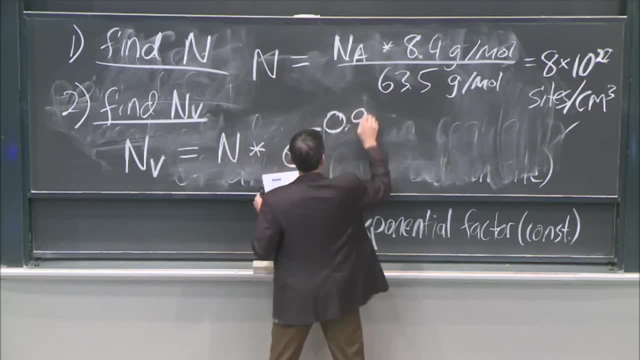 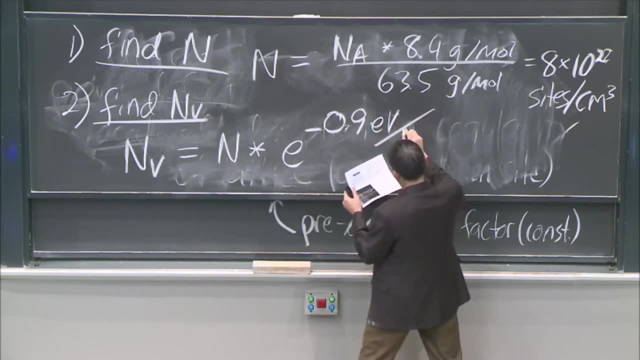 Right, And Then My K B Instead Of R. So It's Nine Point: Nine Electron Volts Divided By, And Then This Is K B. 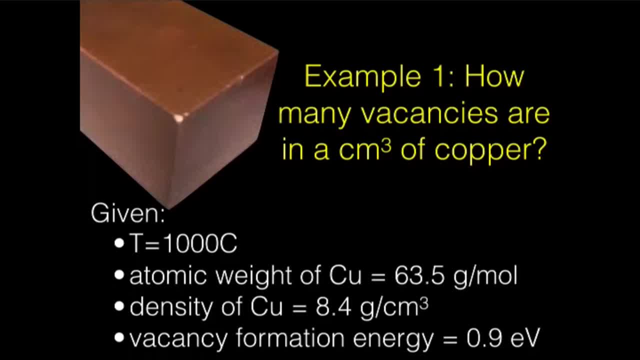 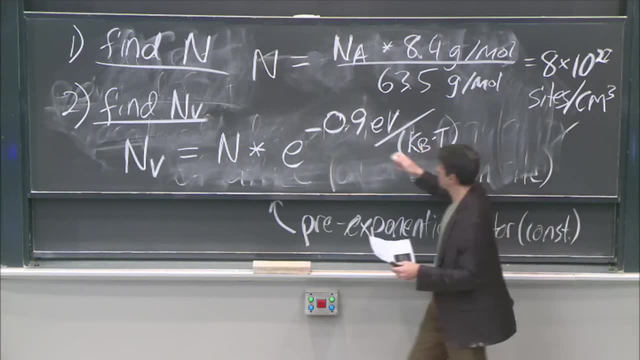 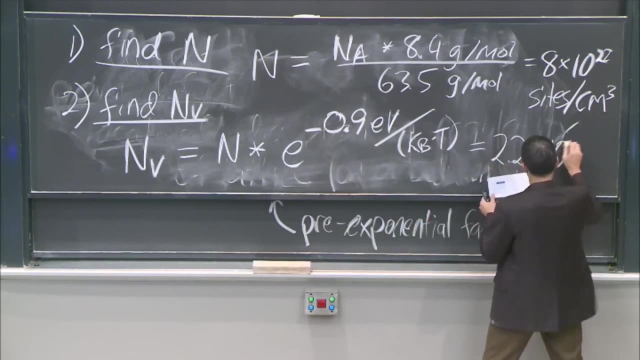 T Now I Can. So I'm Given That T Is Always In Kelvin For Any Of These Thermodynamic Equations And I Won't Go Through. 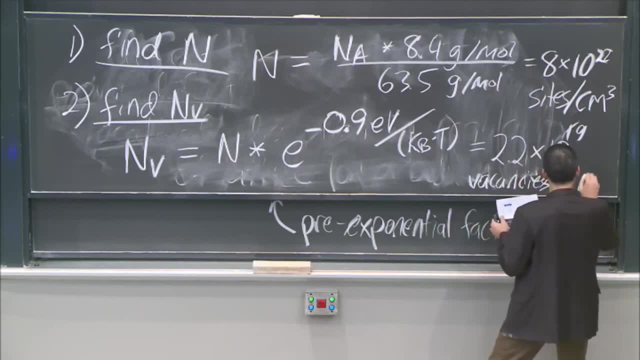 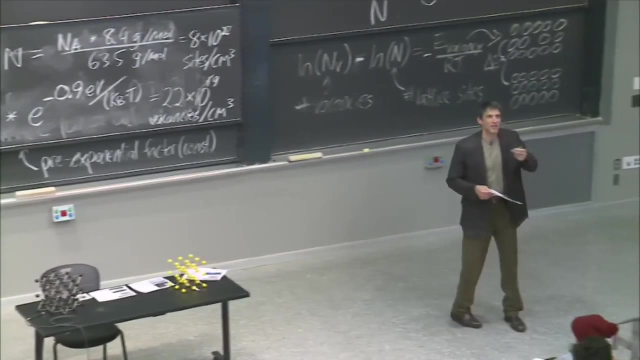 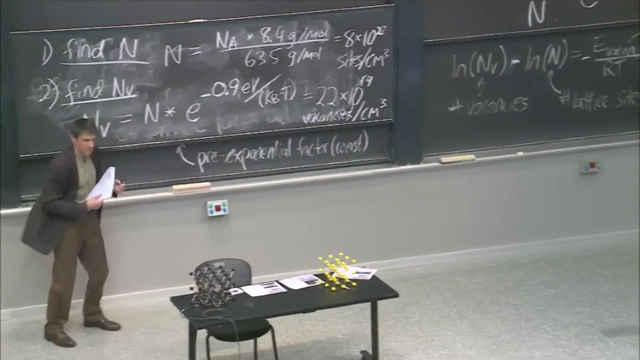 The Math, But It Goes Something Like Two Point Two Times Ten To Temperature. If I Were At Then. This Is The Power Of What Arrhenius? 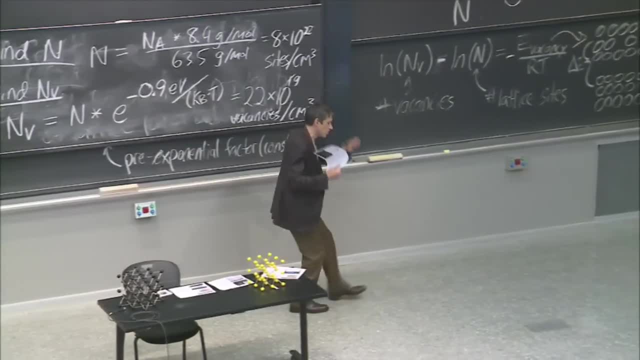 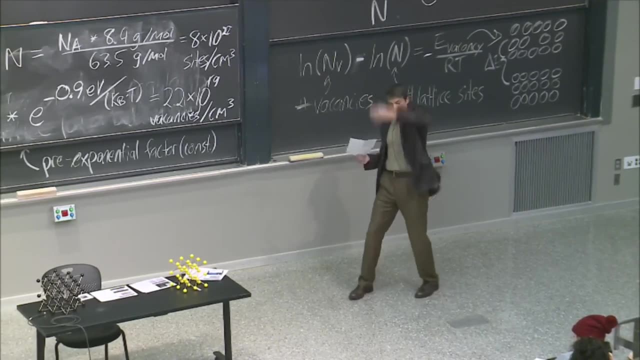 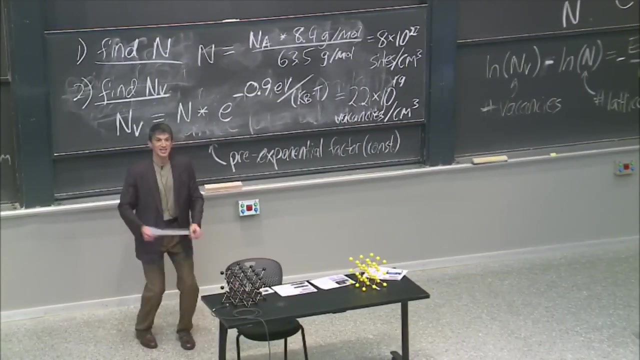 Gave Us If, Because It's Exponential, It's All About Probabilities And Sampling, And How Many Times Is Ten To The Seventh Instead Of? 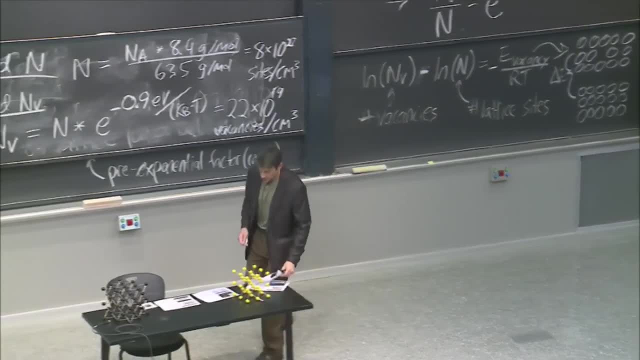 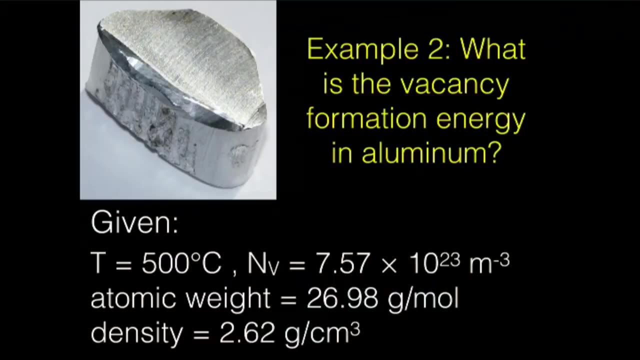 Ten To The Nineteenth Right. So That's The Power Of That Exponential. That's The Power Exponential. You Might Also Be Asked Questions Up. 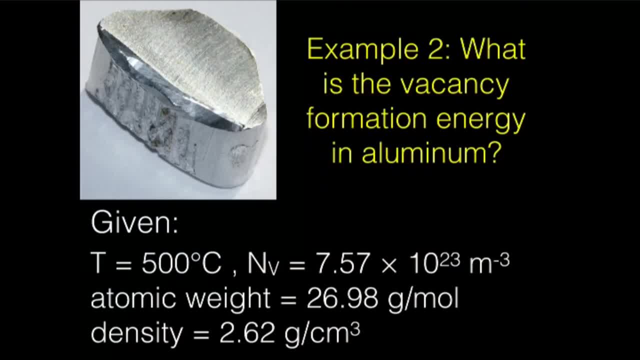 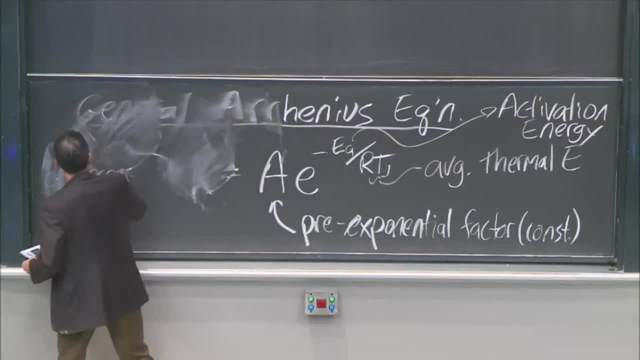 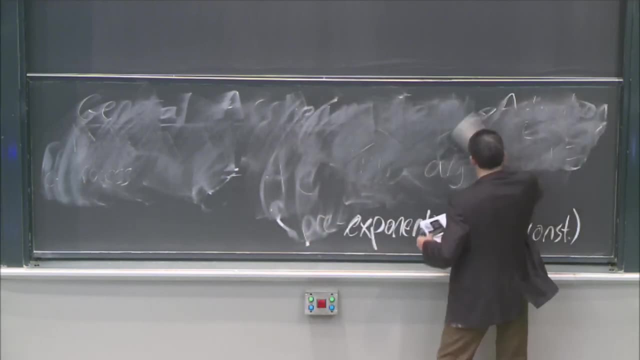 I'm Actually Giving You How Many Vacancies You Got At Some Temperature. Well, That's This, Just Going In A Different Direction To Say: Take. 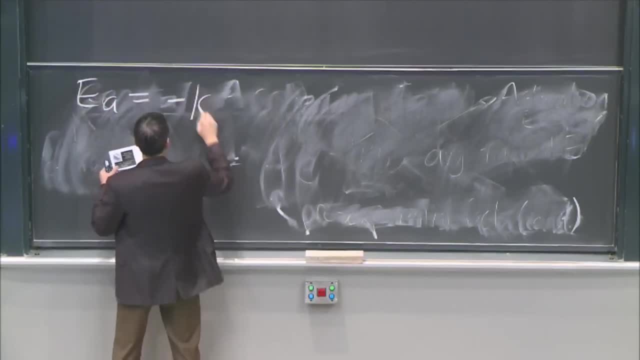 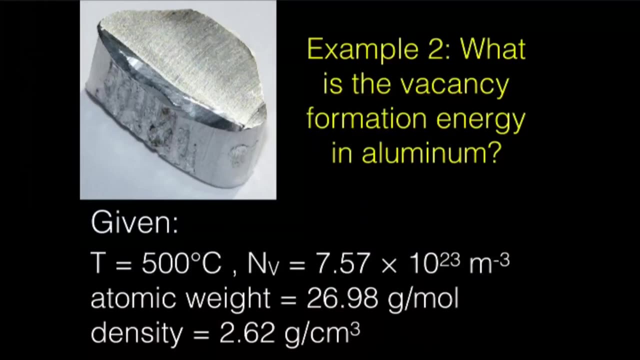 But It's Using The Kb. I'm Using Kb Because Look At That, The Formation Energy I'm Asked Is: What Is A Vacancy Formation Energy? 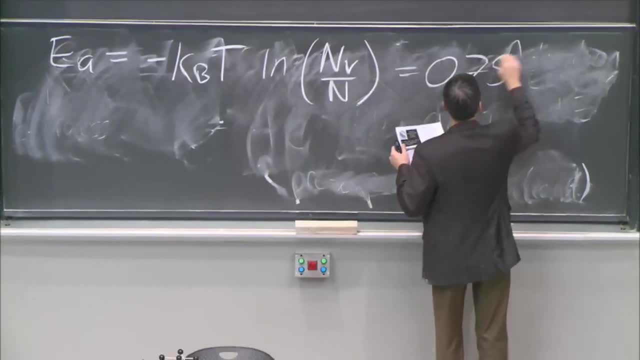 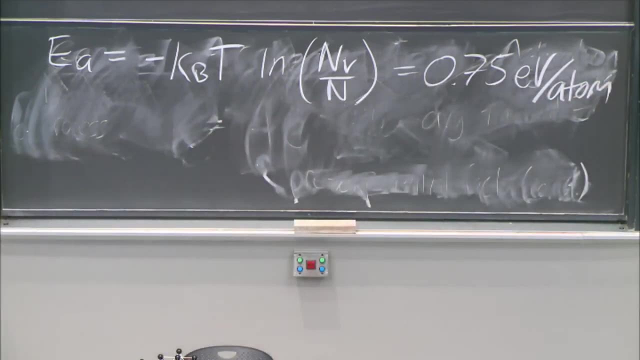 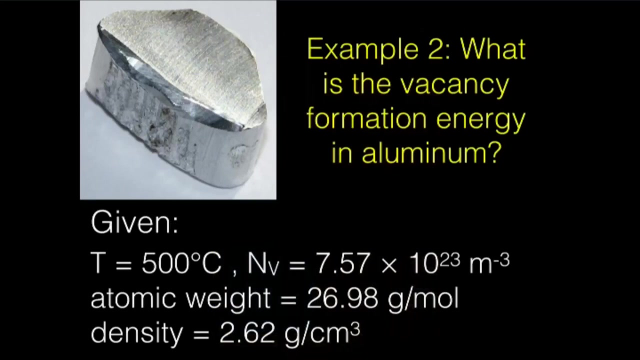 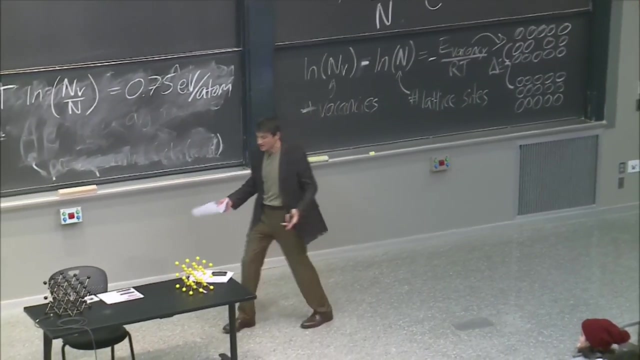 Okay, Well, Actually, Look At That. No, I Just Was. Copper Was Point Nine, Aluminum Point Seven Five. You're Going To Have A Lot More. 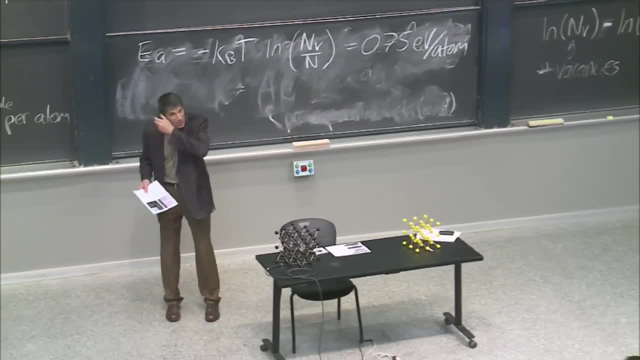 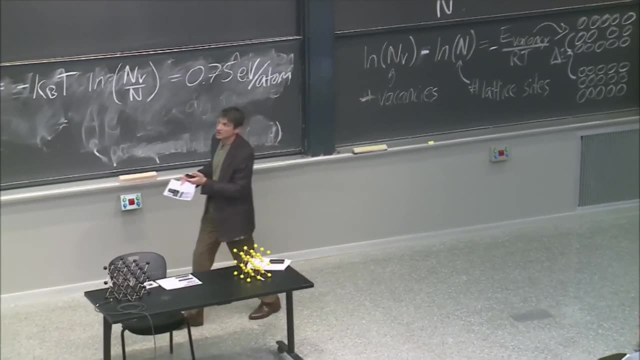 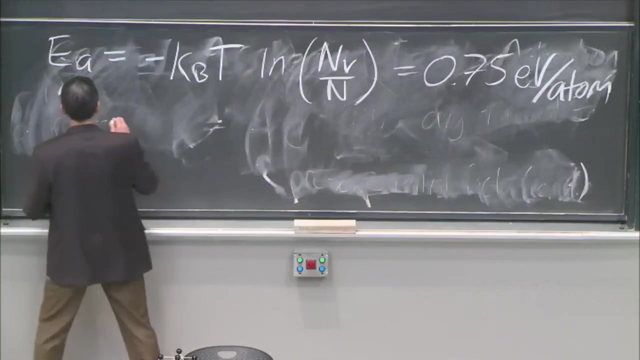 Vacancies, Because It's Exponential. This Seems Like A Point Nine. Point Seven. Five Is One Notice. I Did The Thing That I Said Other. 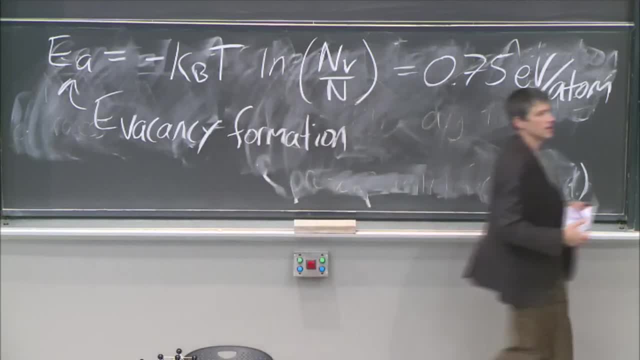 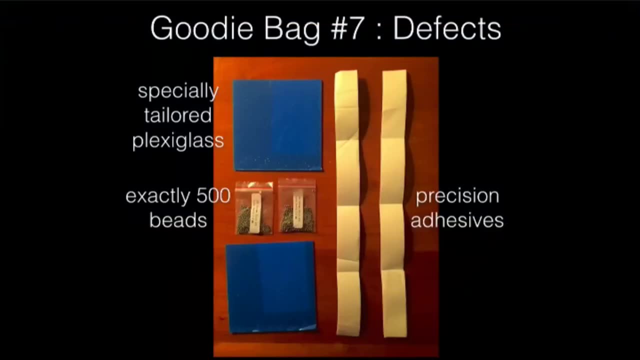 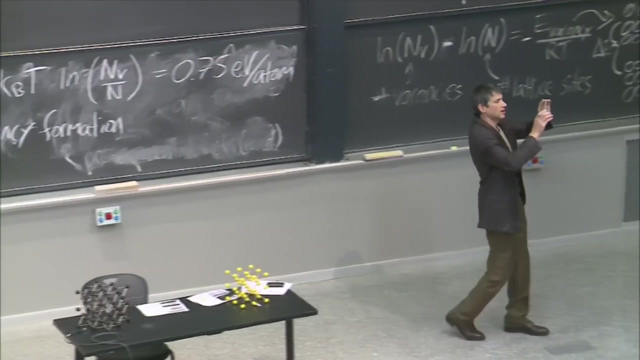 People Do And I Don't Really Like. That's The Energy Of The Vacancy Formation. People Call It Activation Energy, Exactly 500.. Beads In. 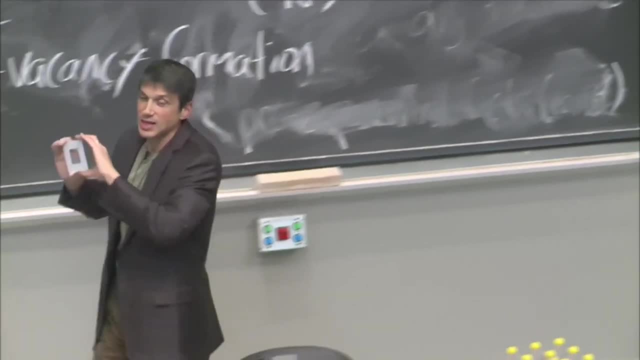 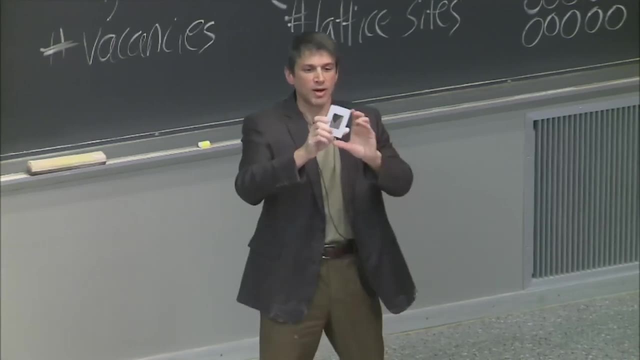 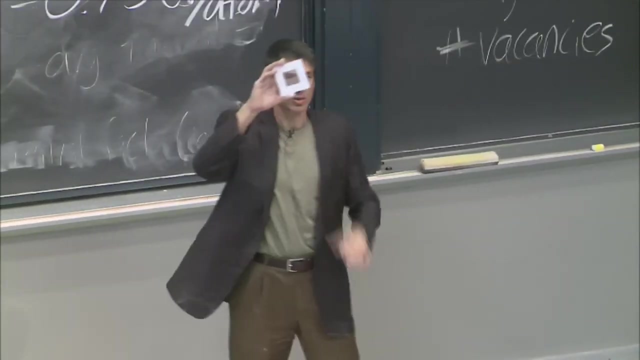 This Exactly. There Are Not 501.. There Are Not 499.. And You Know Why? Because Laura Has Spent 7,000.. Hours Counting Beads. 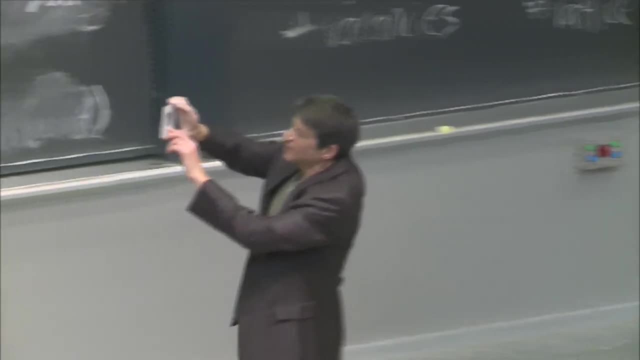 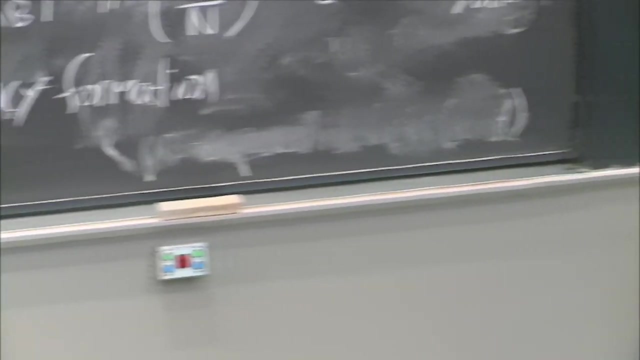 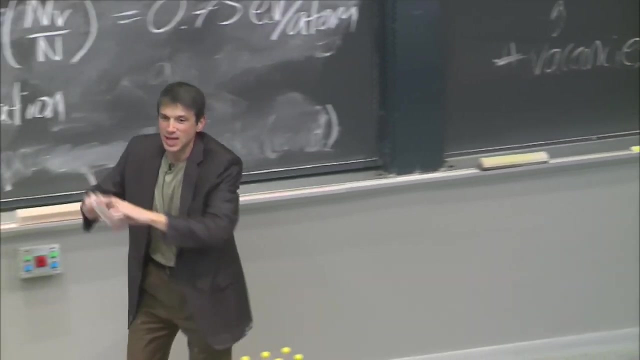 In Every Single Time. That Is A Big Vacancy There. I've Literally Made This Right In Front Of Me. This Is Here And Now. 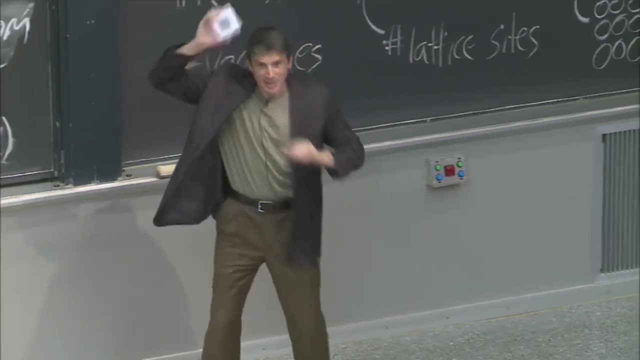 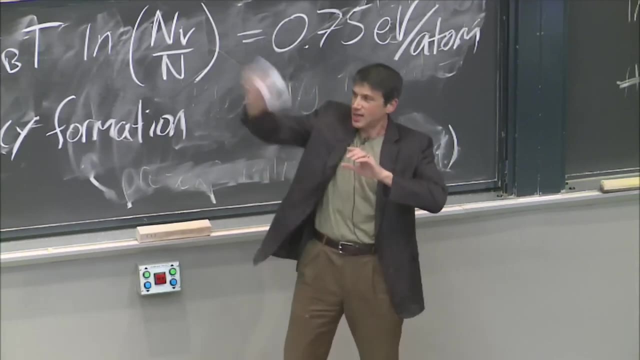 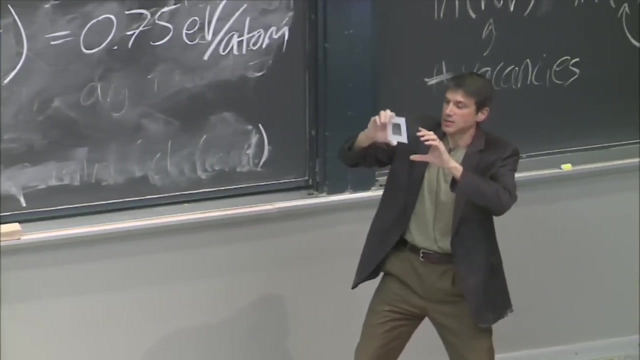 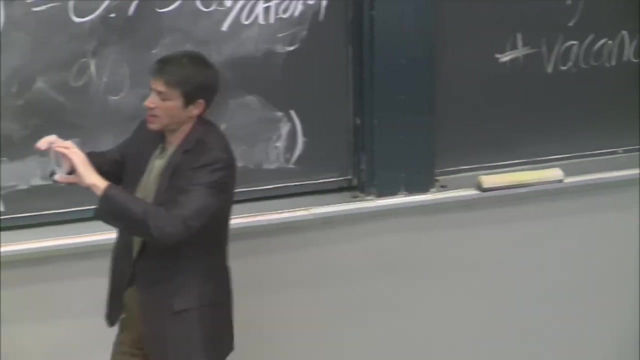 I'm Going To Say, Okay, I'll Use Temperature And You Can Shake It And All. You Bring It To The Dance Floor And And Then 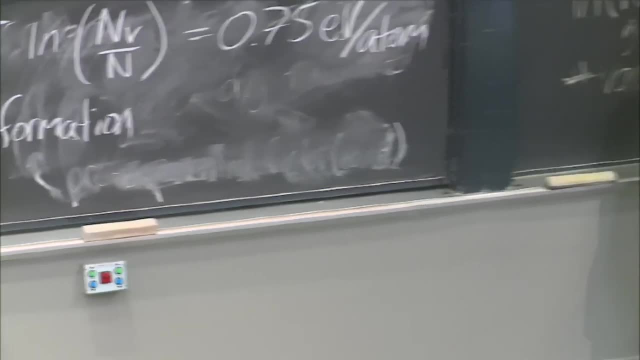 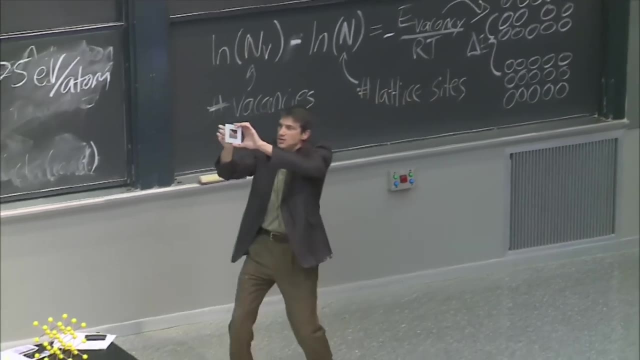 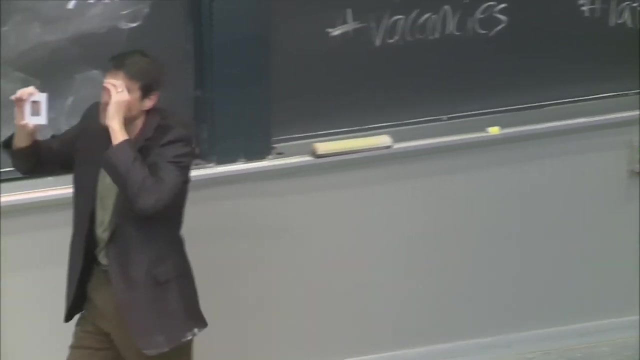 You're Like: How Can I Get? Whoa, Wait A Second, I'll Just See If You Can Get Rid Of The Defects. You Can't. 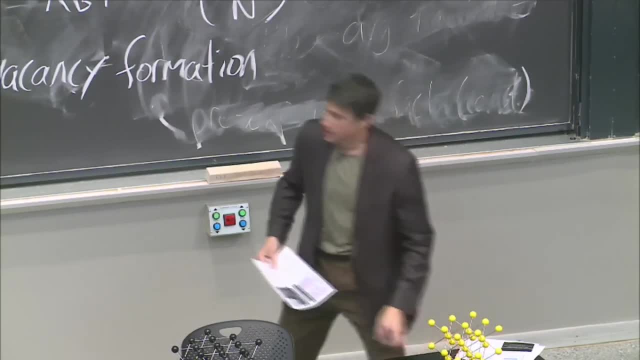 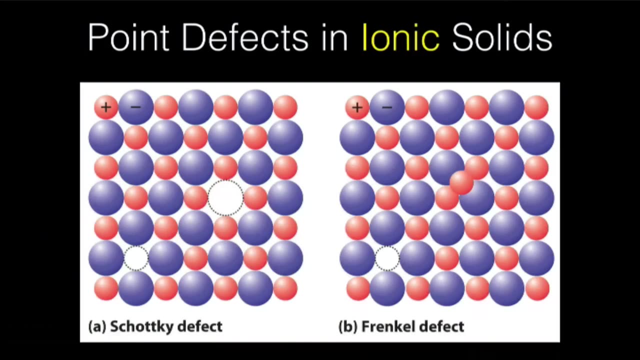 Luckily, That's A Good Thing, Because Defects Are What Make Everything Interesting Everything. This Is Your Goodie Bag, So Yeah. So If I Had. 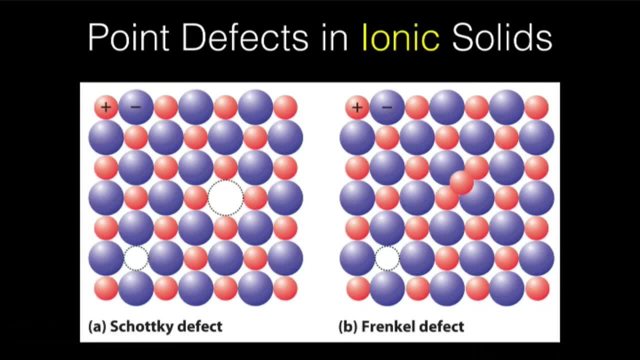 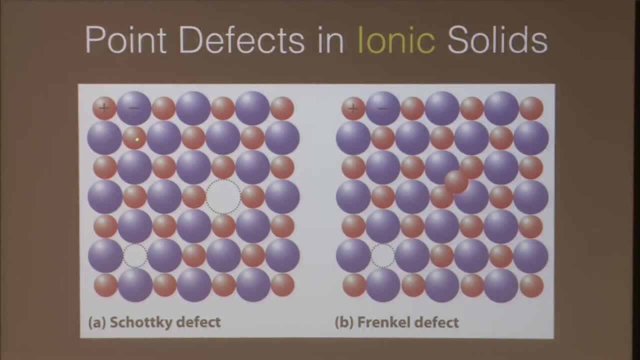 A Defect In An Ionic Solid. Well, Now You Got To Consider The Charge. I Can't Just Keep Pulling This Sodium Chloride I Have 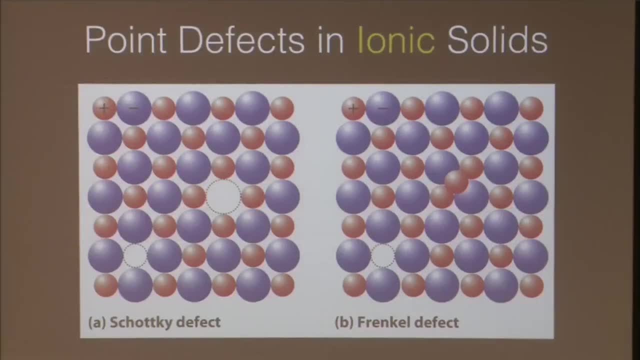 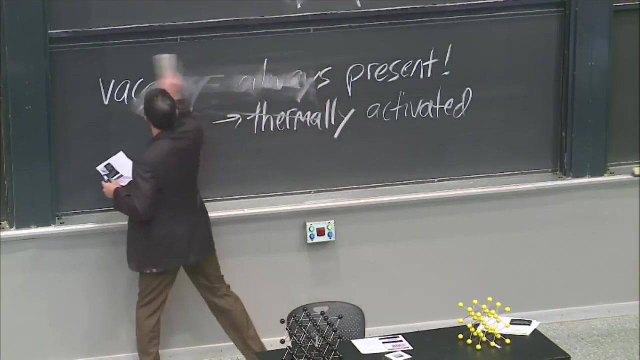 Charged The Crystal. You Can't Do That, It Won't Let You. So If I Take A Sodium At Amount, A Chlorine Is Going To. 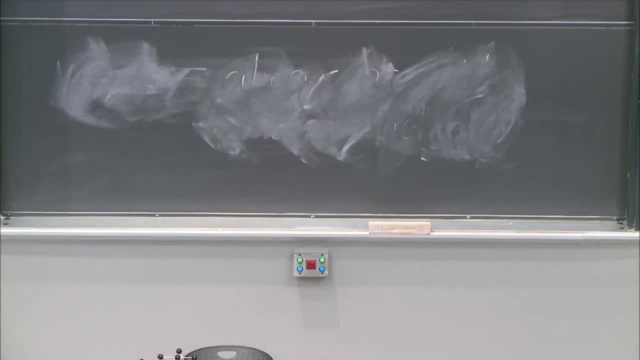 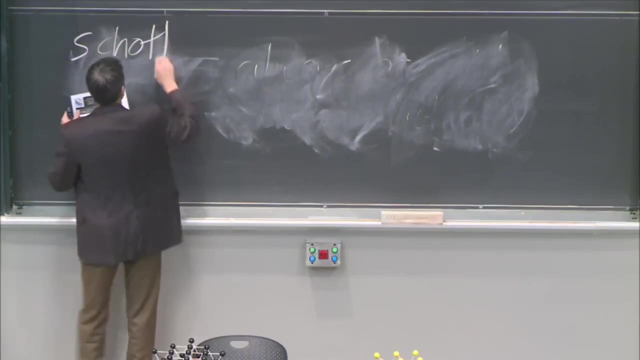 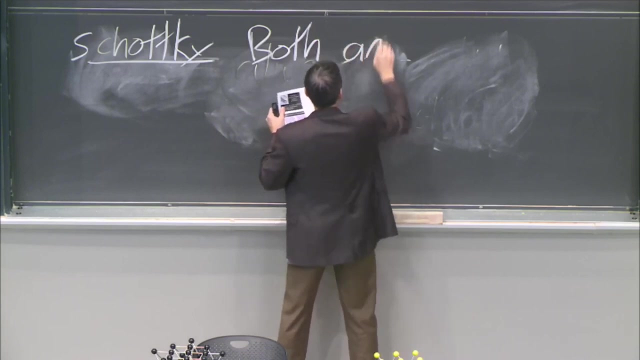 It's Got To Come In. You Got Both An Ion And A Cation. Are Removed Cation? Now Here's The Thing I Should Have Put. 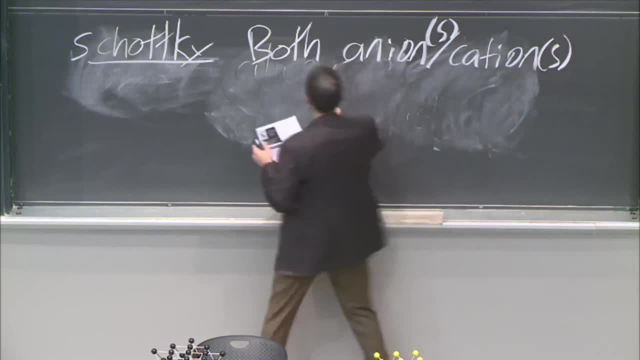 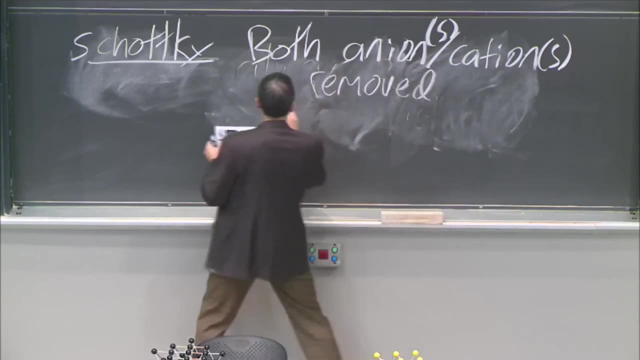 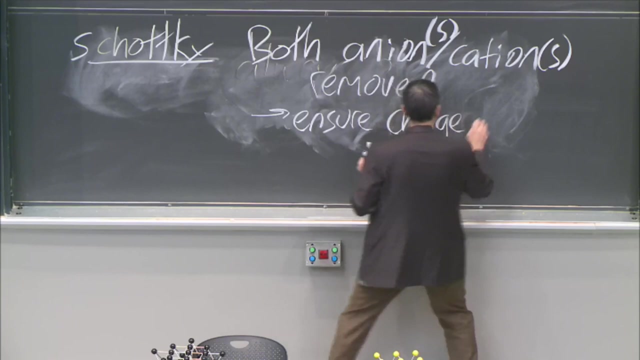 S Because You May Need To Take More Than One, And Sure Charge Neutrality, Charge Neutrality. So, Like You Know, If I Had So 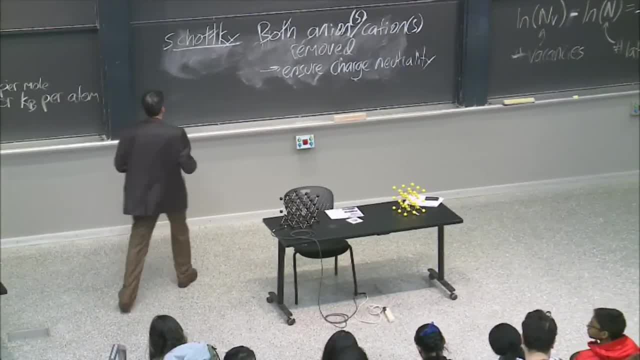 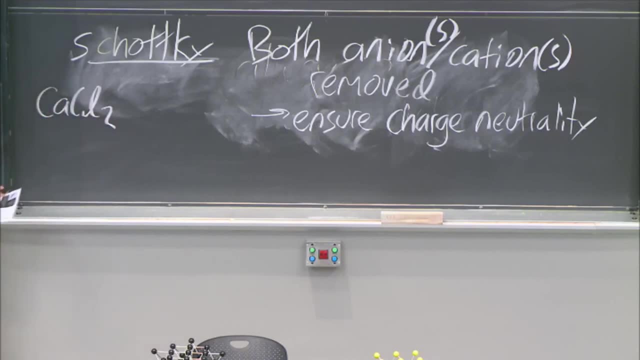 In Chlorine. That's Fine, But What If I Had, You Know, Something Else? What If Chlorine Is Only Minus One, So That Ionic Crystal? 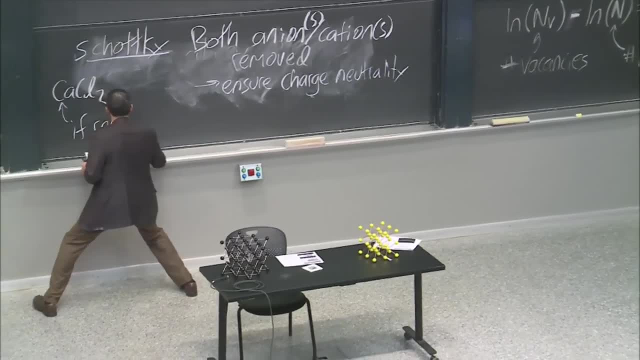 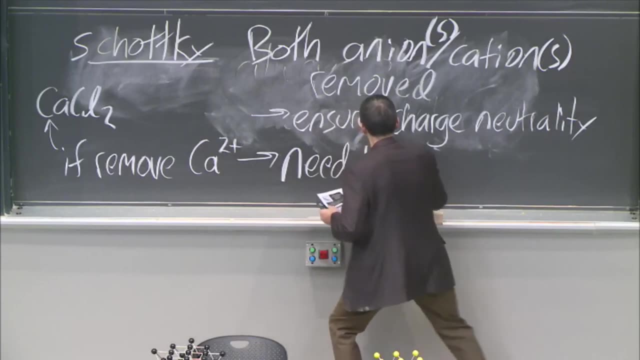 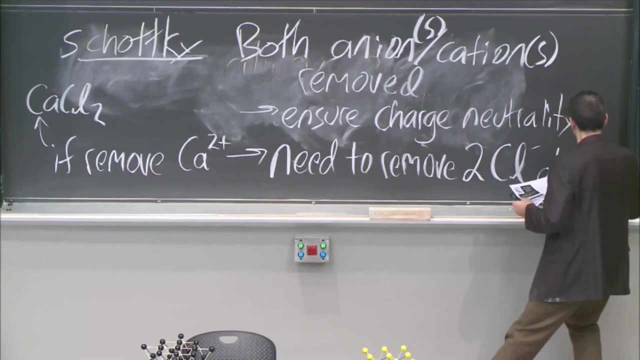 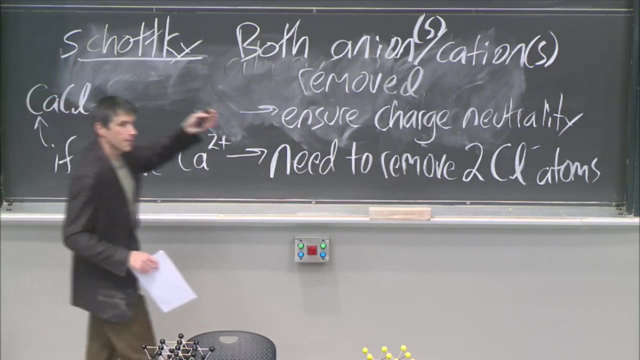 Is Different, And What It Means Is That If I Remove, If I Remove A Calcium, It's Going To Come Out. So So Now You? 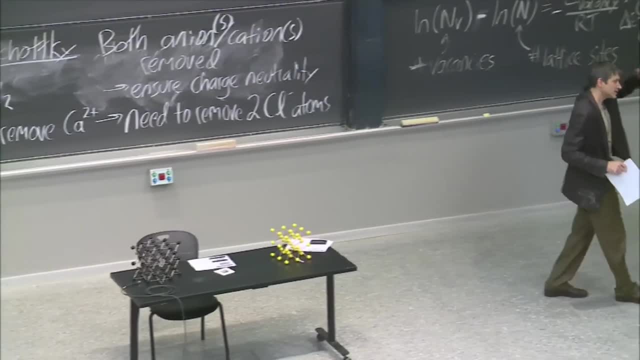 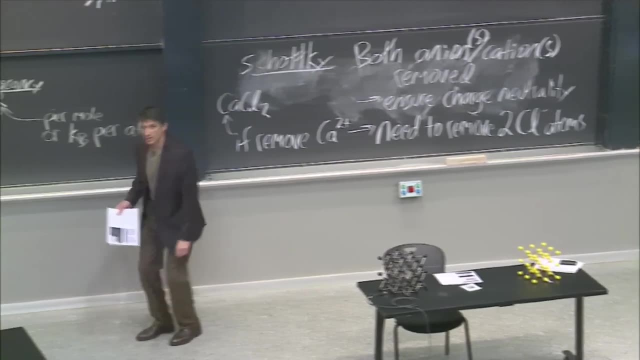 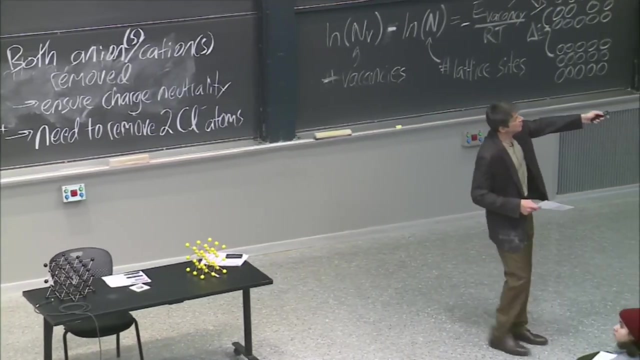 It's Not Just A One For One. This Could Actually Be A Way To Take Atoms Out. What If I Want To Take Chlorine? 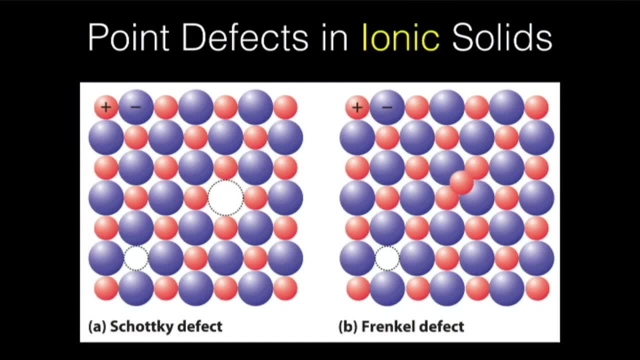 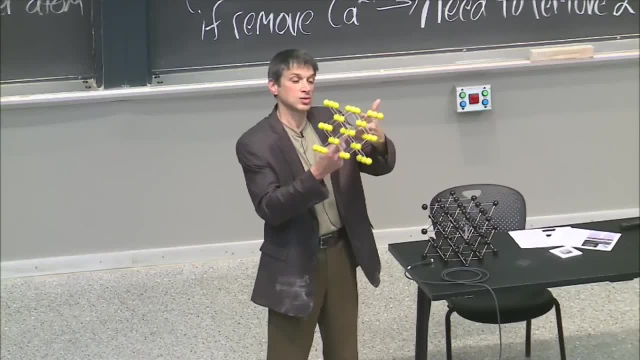 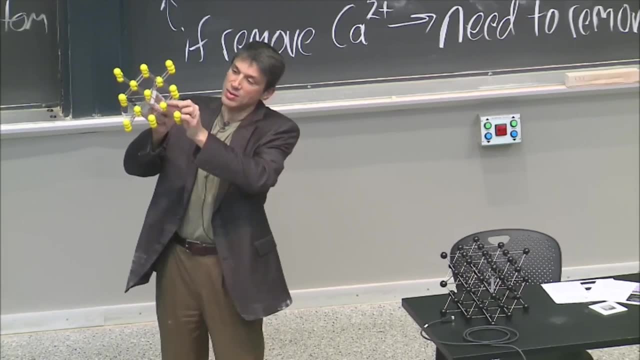 But It Just Kind Of Wandered Over Into Some Site. So, Like You Know, Here's BCC And I Can Have Like An Atom. So 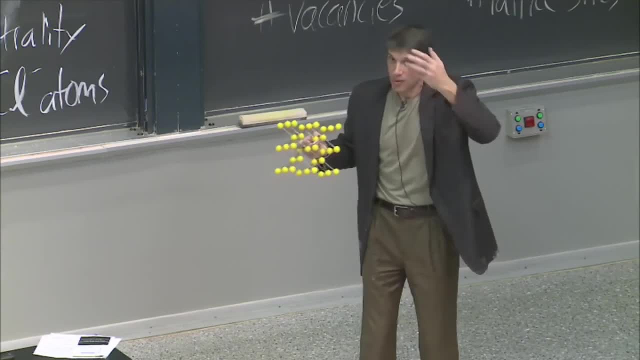 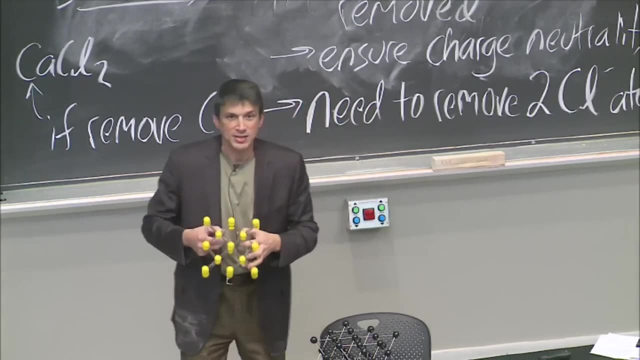 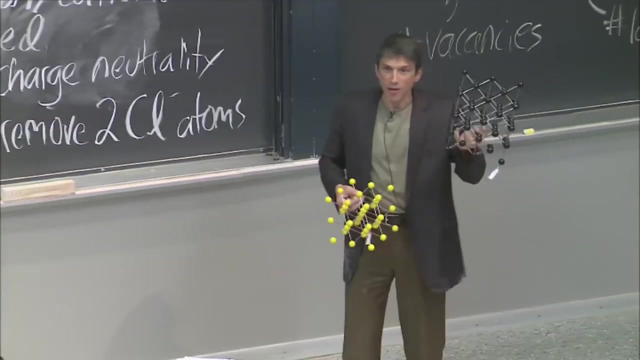 This. I Mean This Doesn't Have A Regular Lattice, But It's It's. It's Like A Hole Right. Remember The Packing Fractions? We Never. 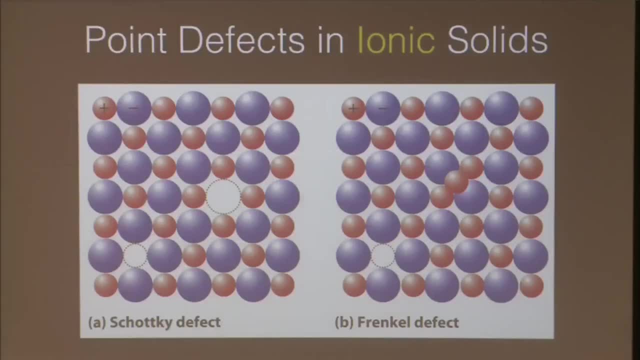 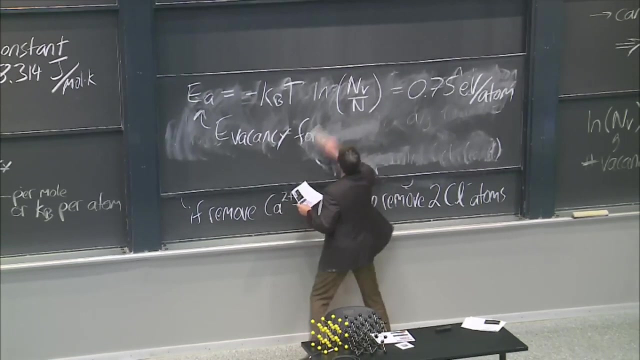 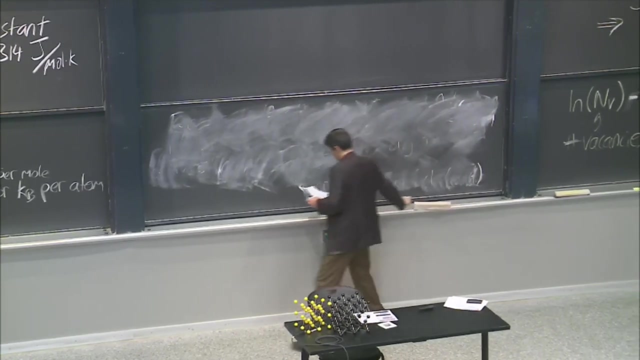 Got Above, Above Three Quarters. We Never Got About Three. Good, Okay, Yeah, We'll Do This And So. So That's Called A Frankel Defect. 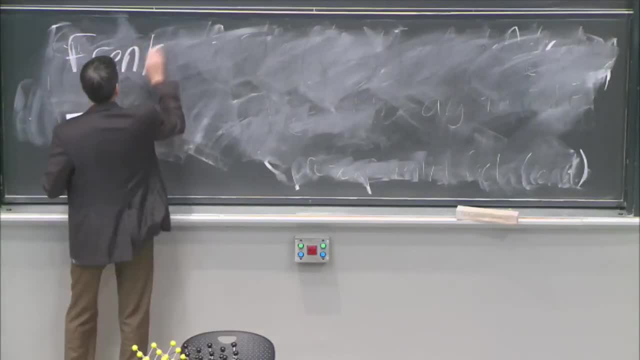 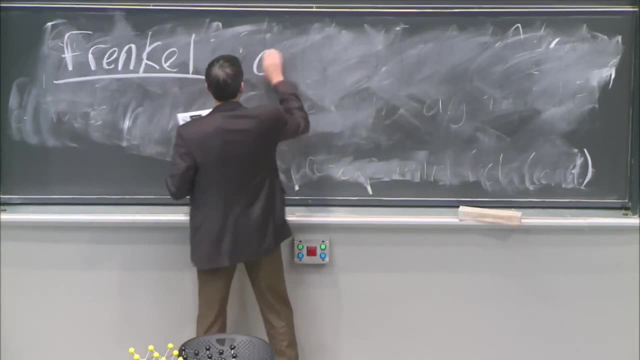 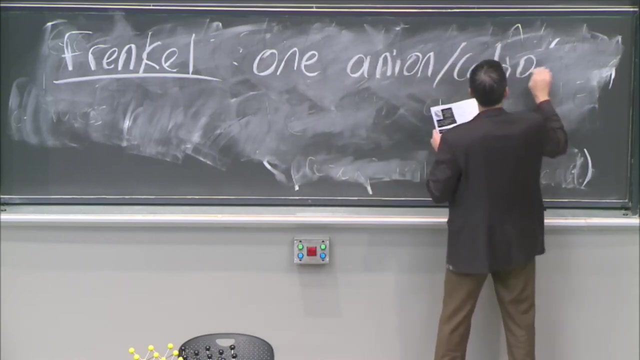 So Frankel Defect Is The Other Kind Of Special Name We Give To A Vacancy In The Land, Moves To Some Open Space, Open. 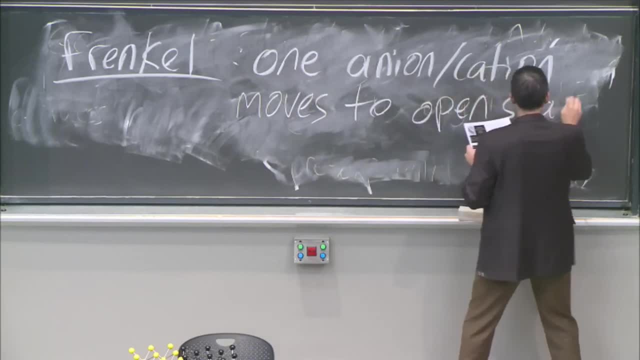 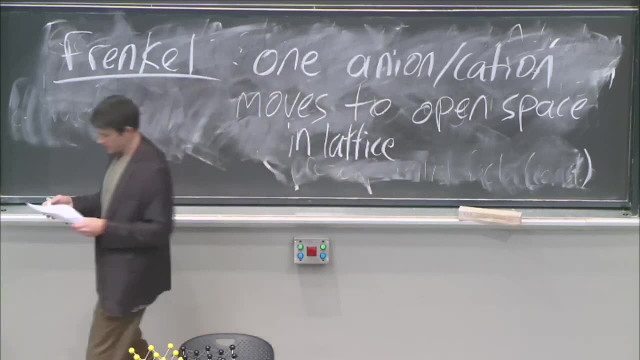 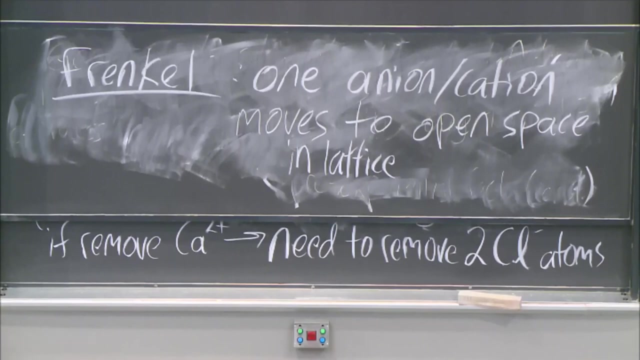 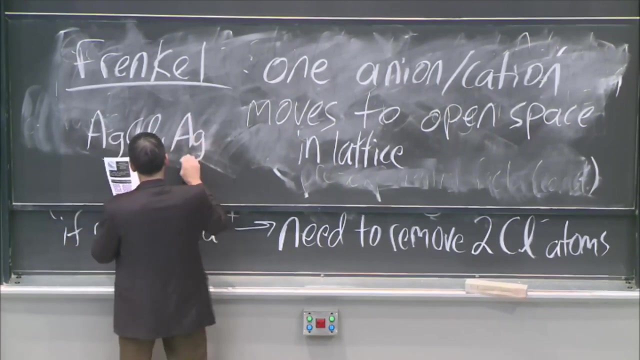 Space In The Lattice And You Can Already Kind Of Feel Where This Might Be Kind Of Common. It Might Be Common If Some Are. 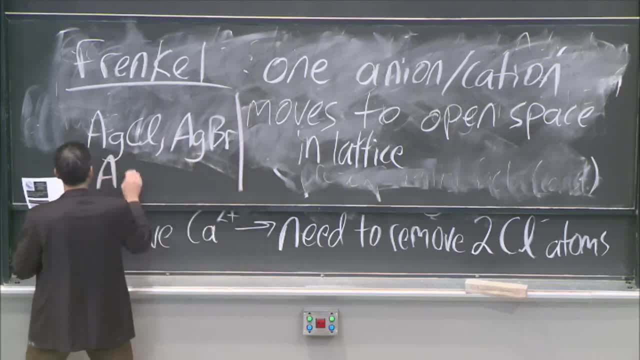 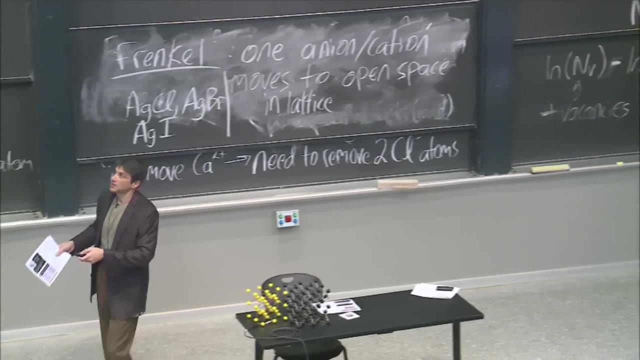 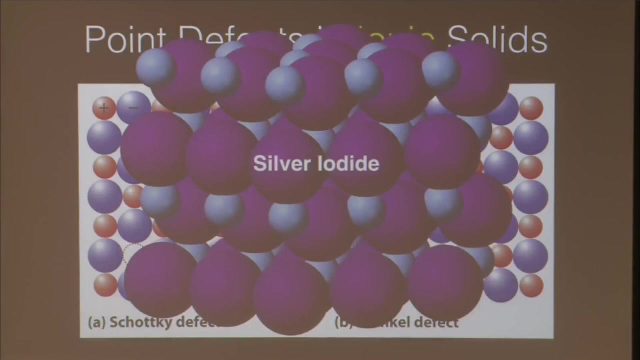 On Neutral At The End Of The Plan T Of The Dü. These Top Of The Program And It Seems To Pay A Lot Of. 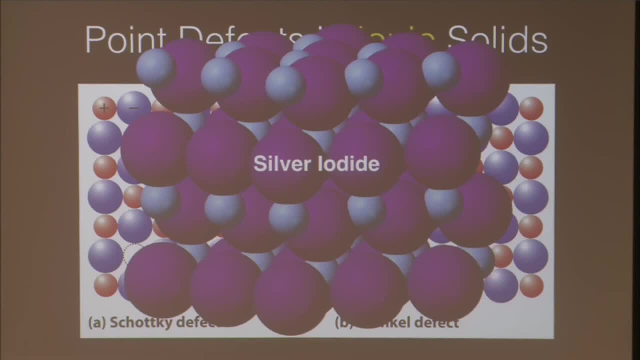 Money is small enough that it actually doesn't mind. It's actually pretty easy to move it. Now, if you think about it well, if you have enough vacancies in there, then maybe those ions can actually move really freely Because they're so small and the voids are all kind of nearby. 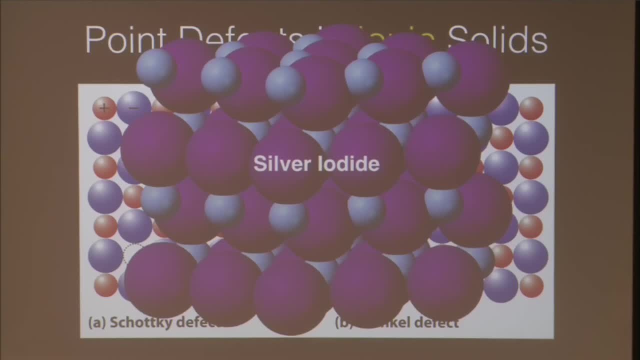 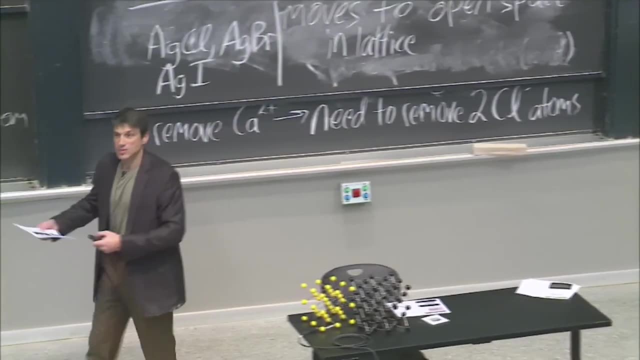 and you actually can get a conductor, a good conductor. this way, You're creating vacancies on purpose, so that one of the ions can move around the smaller one. That's what we do. We make these solid state ionic conductors. 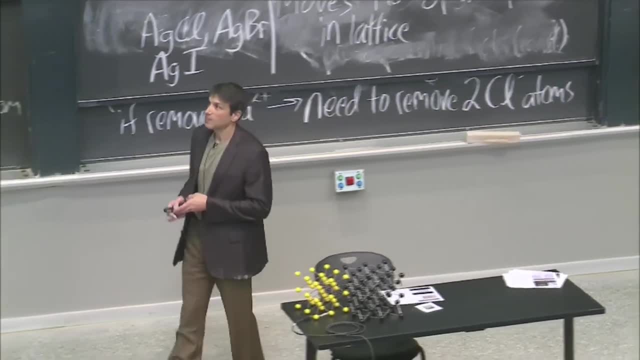 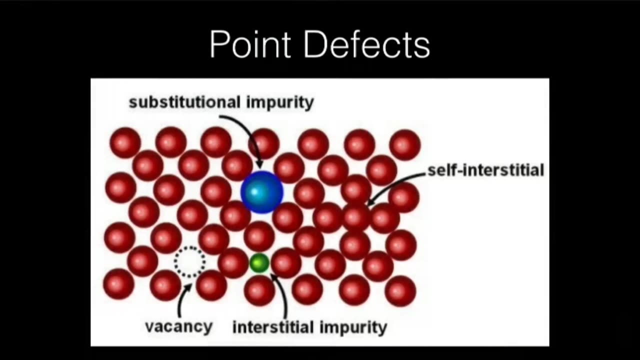 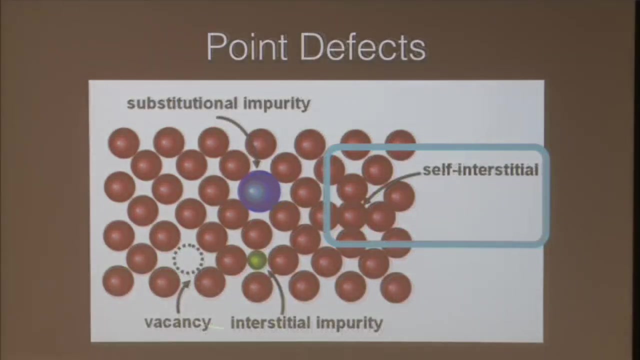 You need the vacancies, You need the vacancies. OK, now, I told you that we got this map here. We've talked about literally just one. Luckily, I don't have nearly the same amount of material to talk about these others. The vacancy is clearly the one that I'm very interested in. 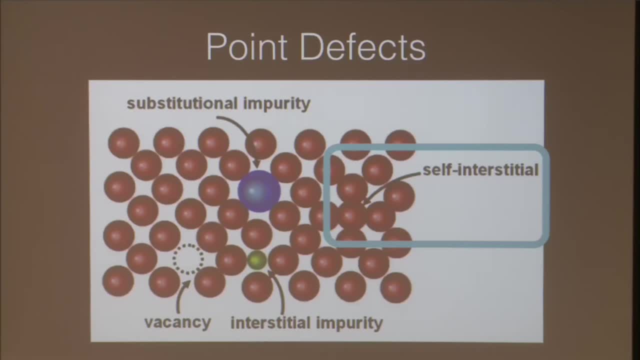 The self-interstitial is actually pretty easy to understand. The self-interstitial is actually pretty easy to understand because it simply doesn't really happen much, And the reason is, if you look at this- here's a picture- It's basically what I drew on the board. 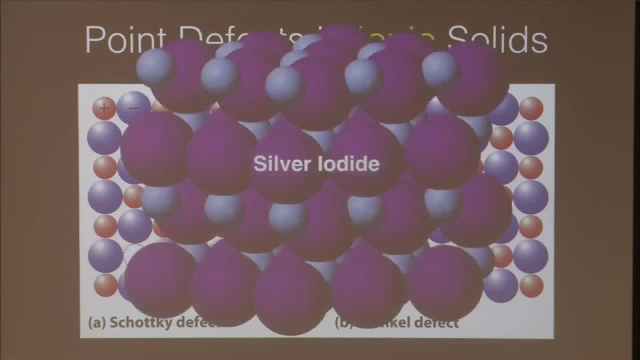 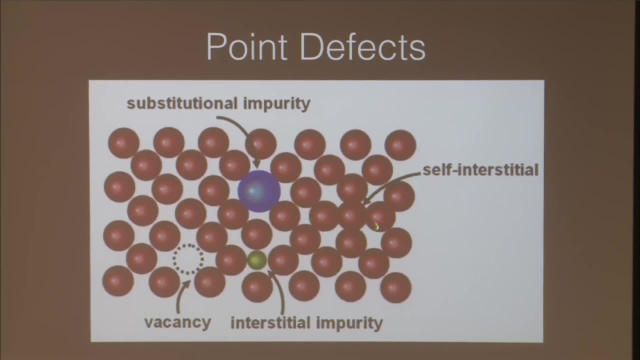 But now I've put so this is not a vacancy. This is a kind of point defect, but it's not a vacancy. I've actually added an atom into the lattice and I've squeezed it In between all the others. you can just. 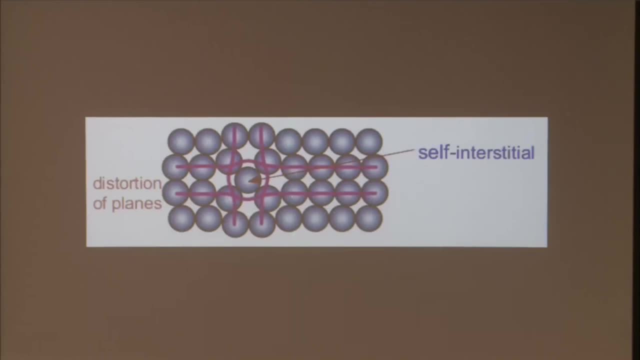 feel how much energy, how much strain those other atoms are going to have to make and how much energy that's going to cost. Those are high energy defects. So a self-interstitial, a self-interstitial self just means it's the same atom as the rest of them. 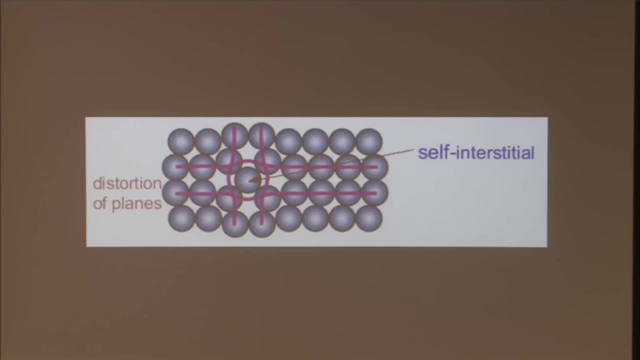 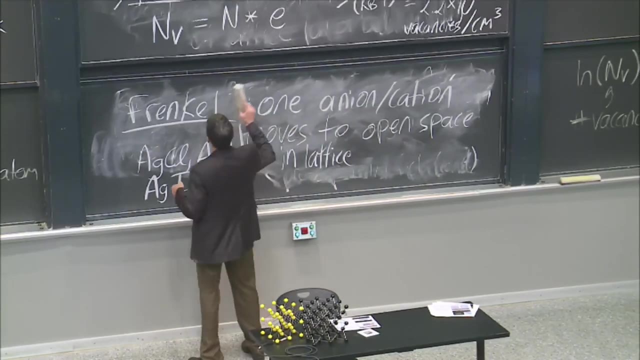 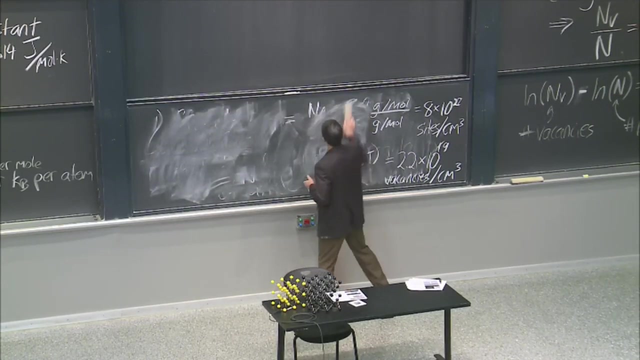 is very infrequent, is very infrequent. The self-interstitial, let's see, I'll just use this one again. The self-interstitial has an energy of Formation of something like five electron volts And you think, but five electron volts.